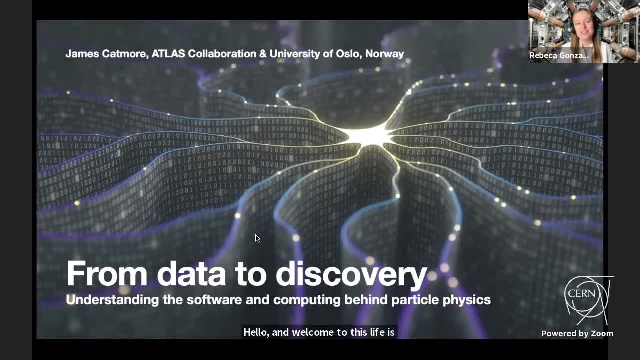 Hello and welcome to this live physicist talk from the ATLAS collaboration. My name is Rebeca González Suárez and I am a particle physicist working in ATLAS, and today I will be the host of this live event. So in the next minutes we will have a live talk that will be followed by 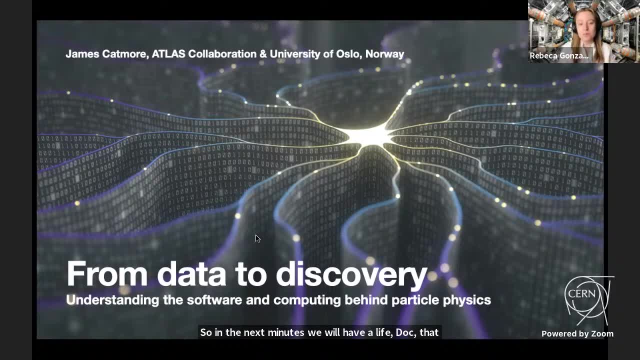 questions at the end. So please use the chat, ask any question you may have. we are going to collect them and we will try to bring up as many as we can at the Q&A session later. So we will also be taking questions from our Instagram account so you can head to our stories there and you can ask. 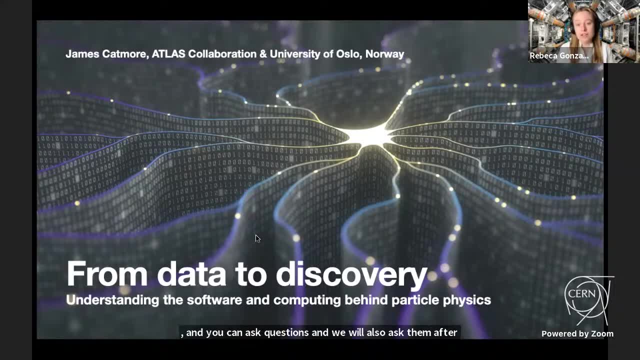 also questions there and we will also ask them after. You can find the link to our Instagram account in our channel description, if you don't have it, so you can go check that. So now let's think about the talk a little bit. So this is the fourth talk in our series and, as the previous three, 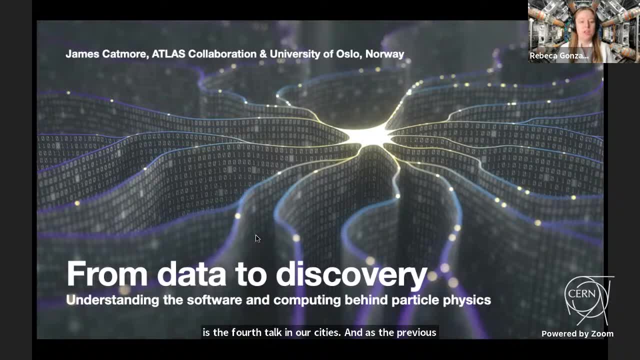 talks will also be made available in our channel after, So do check out the other talks also, if you have not done so before. I think they are all very interesting, But today in particular, our speaker is Dr James Catmore. So Dr Catmore is an experimental particle physicist working in ATLAS and between 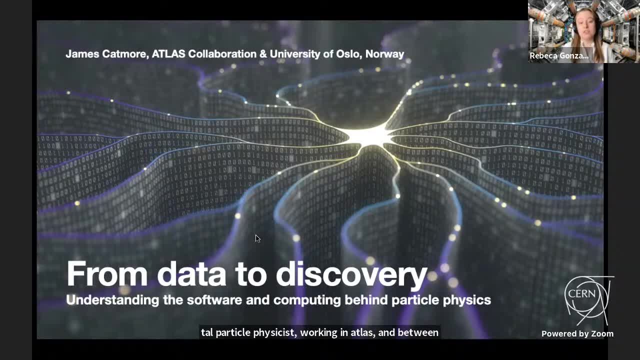 2019 and 2020, he was computing coordinator for the ATLAS collaboration. He did his PhD at Lancaster University in the UK, where he also worked as a postdoctoral researcher afterwards, and then he joined CERN with a fellowship and studied for a couple of years, and now is a researcher at also. 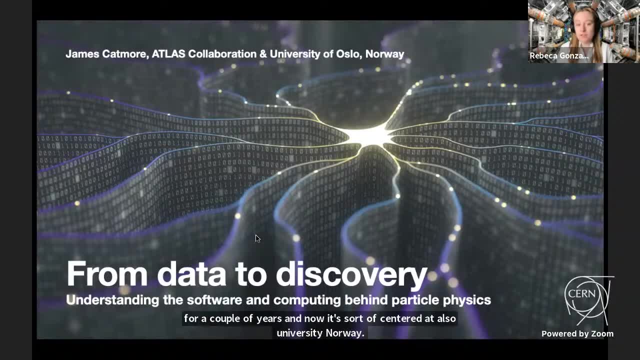 University in Norway. He has been a member of ATLAS throughout his career and today he's going to tell us about something quite important in which he is an expert: The software and computing behind particle physics, something that is really relevant for what we are doing in ATLAS. So hello, James, we are really happy to have 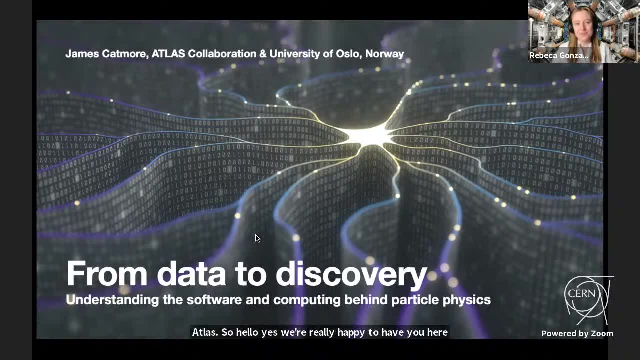 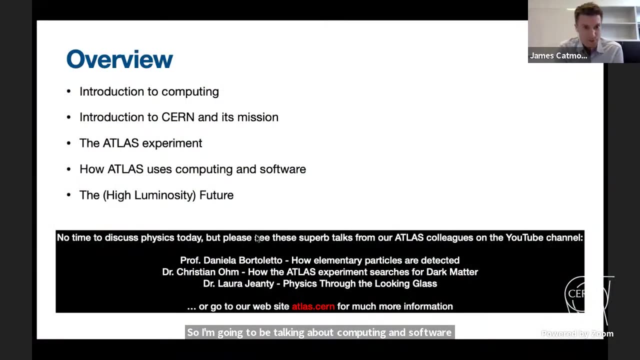 you here today and you can start whenever you want. Great well, thanks very much for the nice introduction and good evening to everyone from Oslo, Norway. So I'm going to be talking about computing and software as a part of what's applied to particle physics. There will not be any time, unfortunately, today to talk about physics, but please, as you already heard, look at the YouTube channel, where you'll see three excellent talks on the physics that we're doing in ATLAS and at CERN, and if you go to our web page, atlascern, you'll find a lot more information. 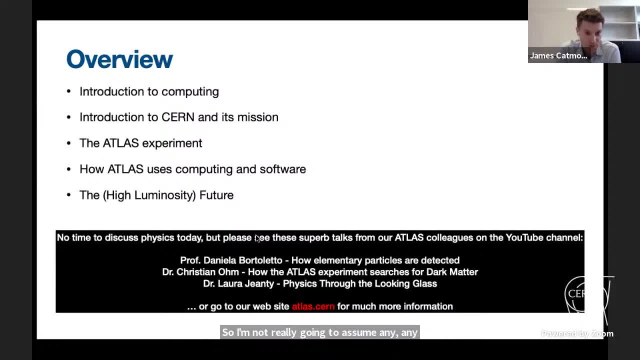 So I'm not really going to assume any knowledge for this talk. so I'll first of all give a brief introduction to computing, and then I'll talk briefly about CERN and its mission, before I go on to discuss the ATLAS experiment and how ATLAS uses software and and computing, and then I will 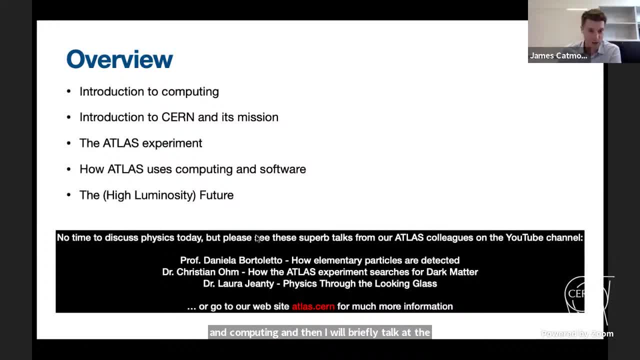 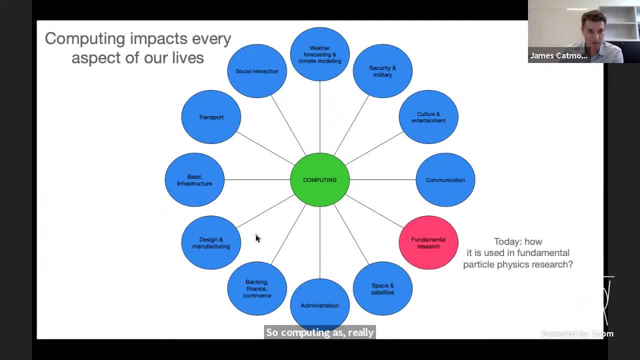 briefly talk at the end about the high luminosity, as we call it, future. So computing really impacts now every aspect of our lives. It's hard to think about anything that we do in our daily life that doesn't, at some level, involve computing, and today I will. 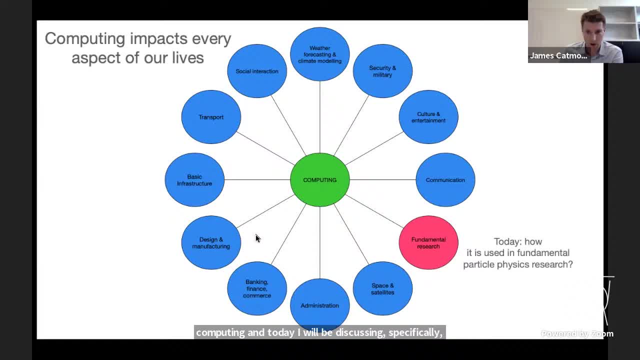 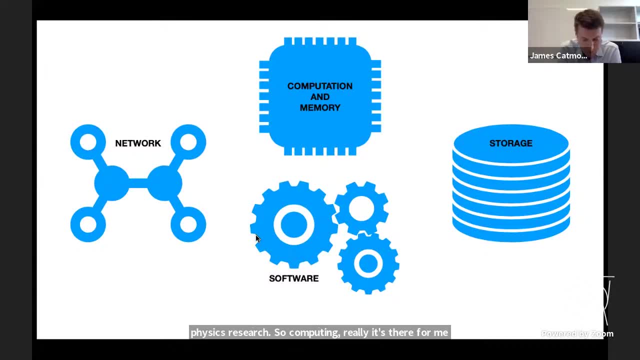 be discussing specifically how we use it to do our fundamental physics research. So computing really it's? there are four main aspects to it. There's the aspect of computation and memory itself, the machinery that actually does the calculations, and then there's the software that we run on that. 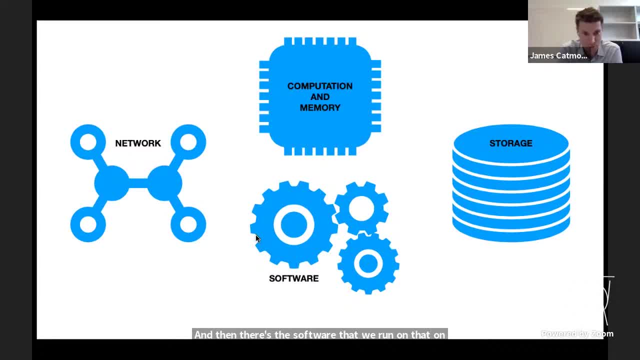 on that computation hardware where we give it instructions for what we need it to do. We have storage where we keep the data and we have network for transmitting information from between computers, and I'll be discussing all of these in the next few minutes. So if we take 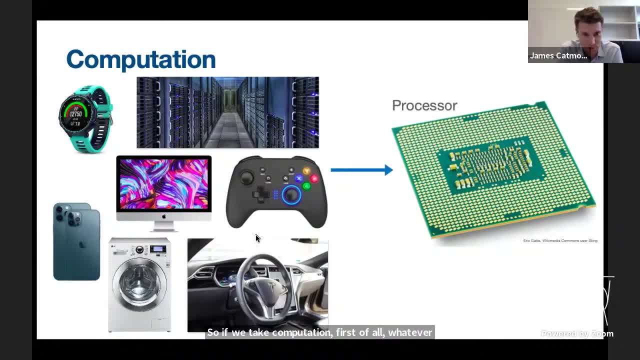 computation. first of all, whatever device you have in your homes or that you use, whether it's your washing machine or games console or your phone, or even a very sophisticated data center in Google or wherever, it all boils down really to this object that I've shown on the right hand. 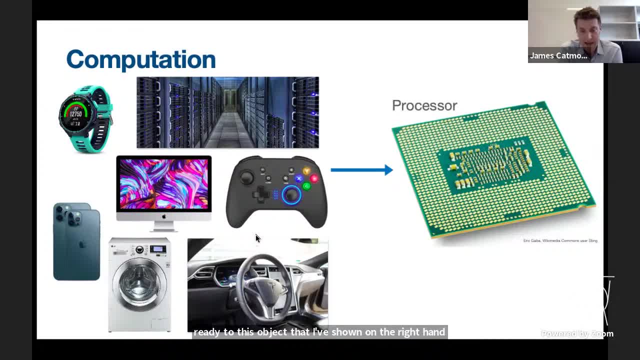 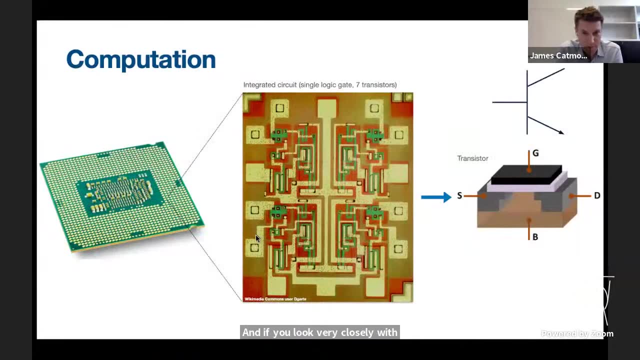 side, a computer processor And the way to think of this really is the mathematical brain of a computer that performs calculations very, very quickly in order to enable it to do the tasks we need it to do And, if you look very closely, with a very powerful microscope at the surface. 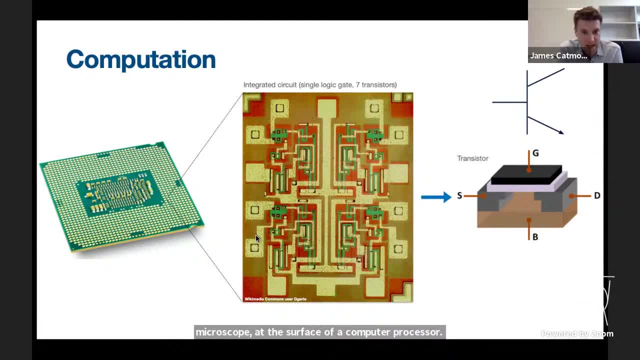 of a computer processor. what you will see are tiny electronic circuits which are etched into the silicon that the chip is made of. These are called integrated circuits, and they themselves are comprised of something called transistors. And the easiest way really to think about a transistor- 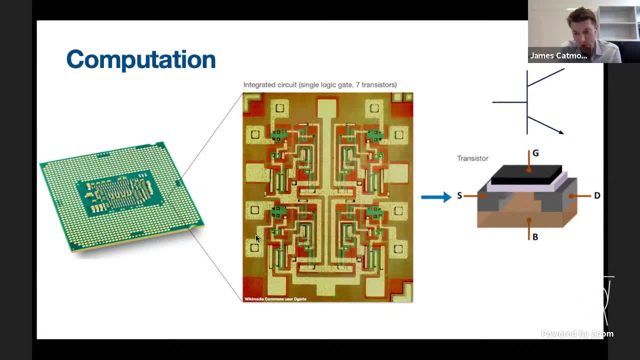 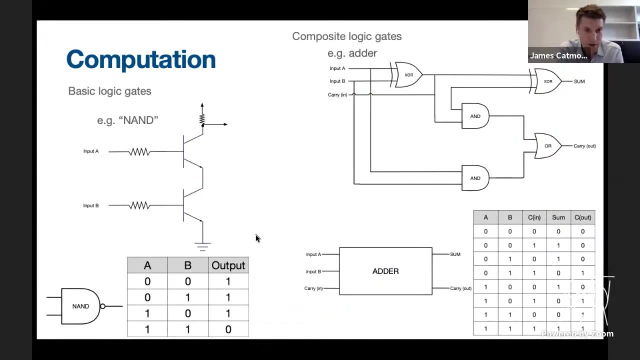 is a form of electrical switch that can be switched on and off using another electrical signal. So this really is what you find on this surface of a computer processor, And using all these transistors we build up something called logic gates, And a logic gate is a small group of it's, an electronic circuit, a small group of. 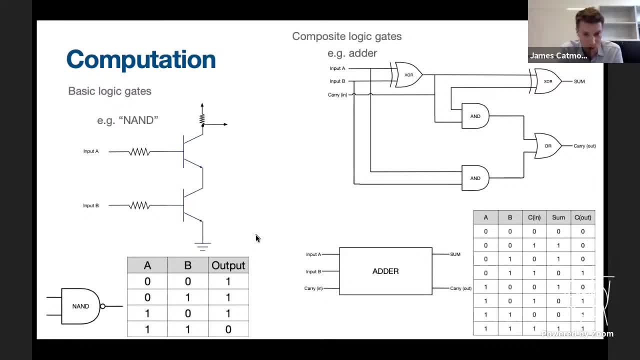 transistors which can perform very simple logical or mathematical operations, depending on whether the inputs are on or off. With computers, you only have on or off one or zero. that's what binary means. And if those of you who've either done physics or are doing physics or electronics at school, 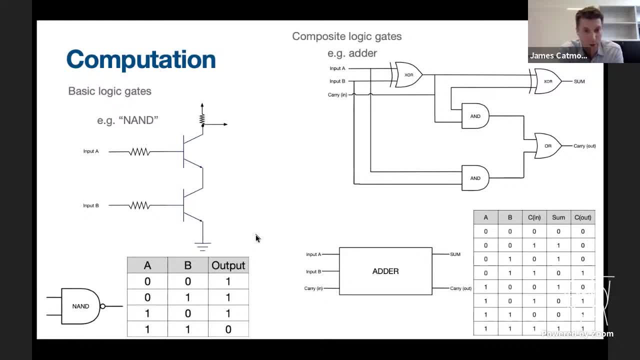 may remember these tables that define how a particular logic gate behaves, depending on whether the input is on or off, And these can be combined into more complicated circuits. So the one on the left is a very simple one, and I've shown a more complicated. 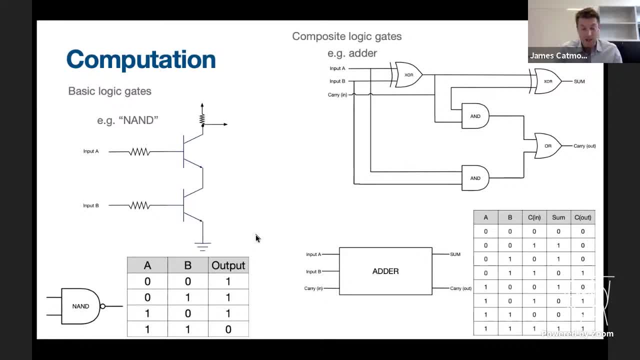 composite one, And they can be made more and more complicated until you build up an overall, a much more sophisticated device that can perform all the tasks that we need of it. And modern computer processors are mind-bogglingly complicated. They typically have more than 100 million of these. 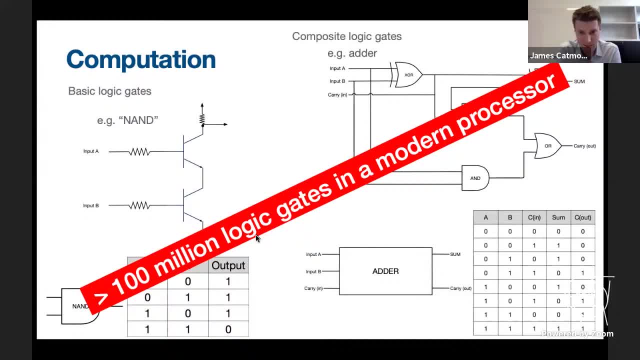 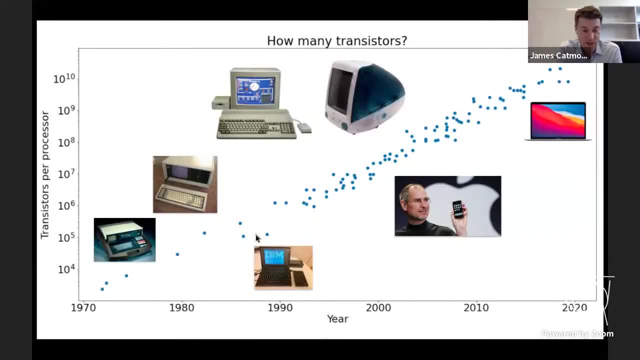 logic gates etched in a tiny surface of this processor. It's really quite amazing how tiny these circuits are In terms of the number of transistors, the number that has. since integrated circuits first came out in the 70s, the number of transistors has grown. This plot is showing how many transistors were. 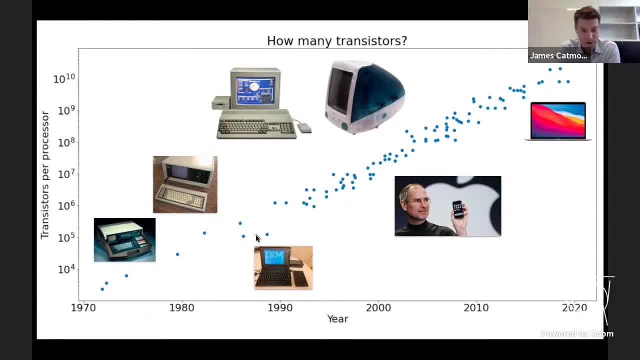 found on a computer processor with time from the 1970s to last year. It looks like this is a straight line, but if you look at the scale, each of these numbers is 10 times bigger. So 10 to the 4 is 10,000, 10 to the 10 is 10 billion. 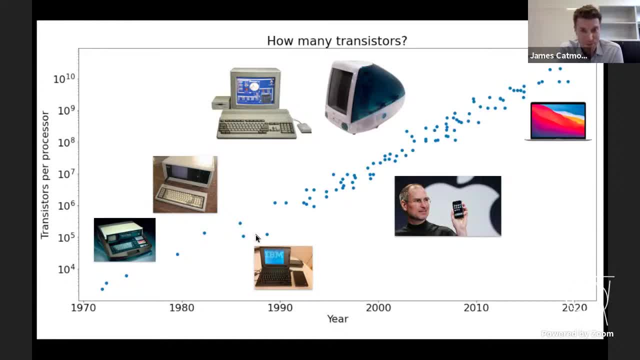 And you can see that computer processors have millions of times more transistors on them than they had back in the 70s, And this has enabled us to progress, as you can see from these pictures, from very basic, old-fashioned looking machines to the sort of sleek laptops that we have now. 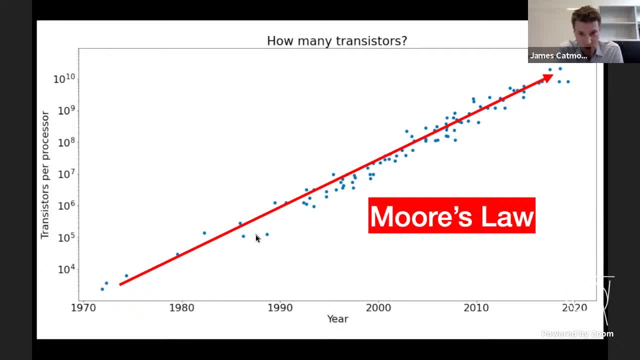 And this increase in the number of transistors is something called Moore's law And this says that roughly every two years the number of transistors in a computer processor or a processing unit roughly doubles every two years And that trend has started in the 70s and 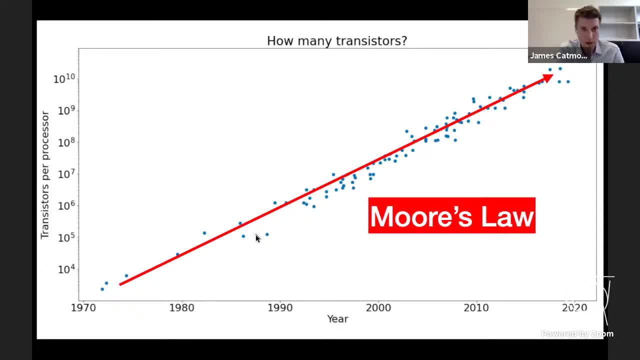 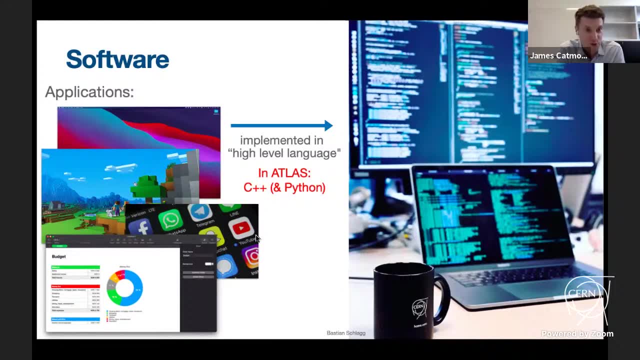 it more or less continues to this day. And then on software. this is the instructions that we give to computers to make them do what we want, And the the side of software that we interact with in our daily lives are called applications, And I've shown some screenshots of typical applications. 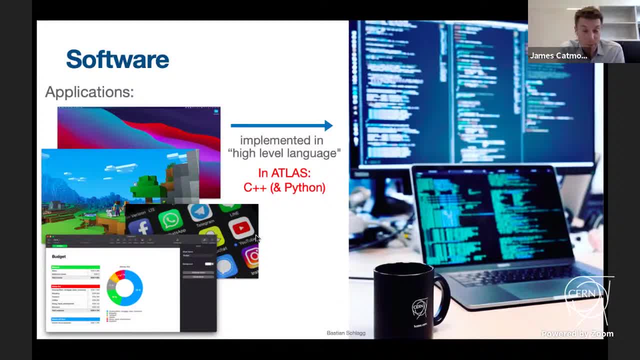 the things that you're used to using on a daily basis, And these are implemented in what's called high-level computer language, And these are instructions that human beings usually write to the computer, giving instructions as to how they want the software to behave. 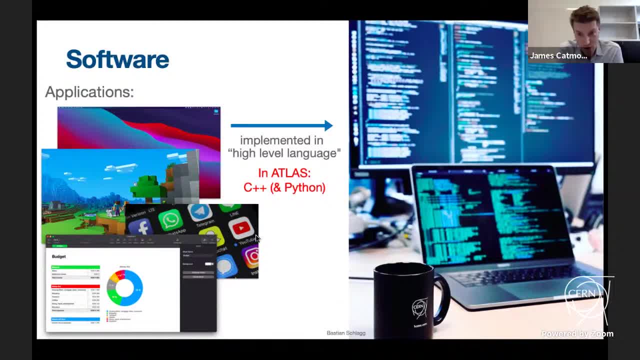 And the reason they're called high-level is that they can be read off the screen or off paper even by a human being, And if the person is sufficiently experienced they can usually understand just by reading the software what it's supposed to do In the Atlas experiment. 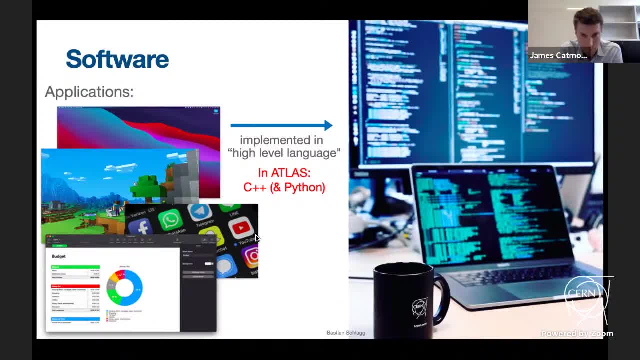 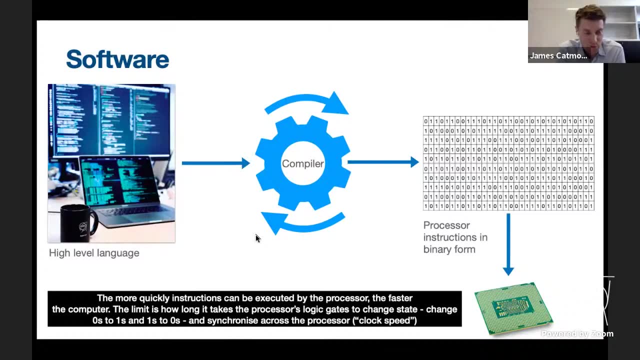 the main high-level language we use is called C++. We also use another computer language called Python for certain tasks, But for the big mathematical processing, heavy-duty processing, we use the C++ language And this software that's written in a human-understandable form. 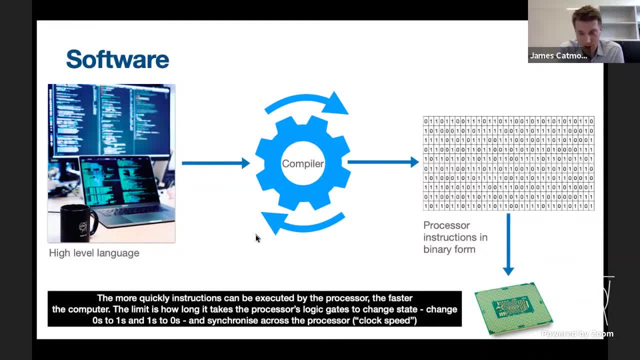 has to be digested by something called a compiler and turned into a series of instructions that the computer processor can understand, And of course these have to be expressed as ones and zeros. These instructions get loaded onto the processor's memory, and then they get executed, one at a time, by all these logic gates that I mentioned earlier. 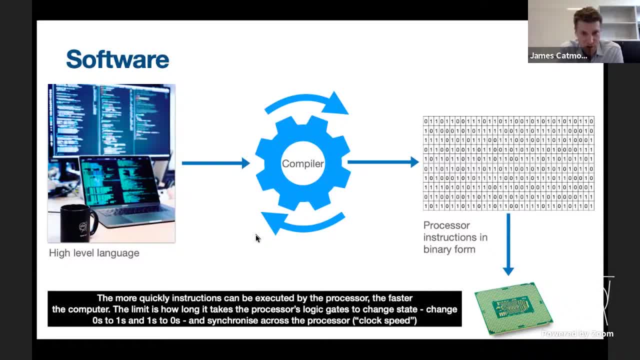 on Now. the more quickly that these instructions can be executed by the processor, the faster the computer seems to be to the user. And what limits how fast a computer processor can run is how long it takes all of these logic gates, as I described earlier, to change state. So for all the ones to go to zeros and the zeros to go to one. 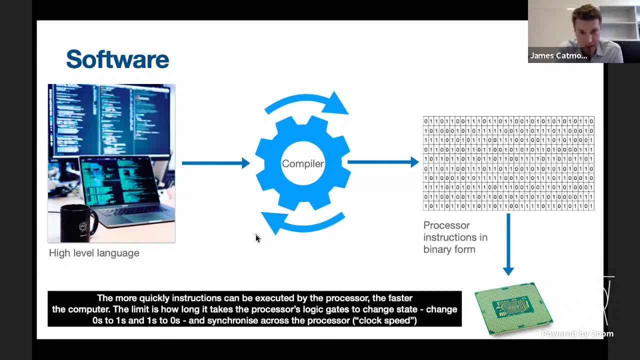 and then for this to be synchronized across all of these hundred million logic gates. This is the sort of what sets the limit as to how fast the computer processor can operate at, And this synchronization is referred to as the clock speed. You sometimes see this on the 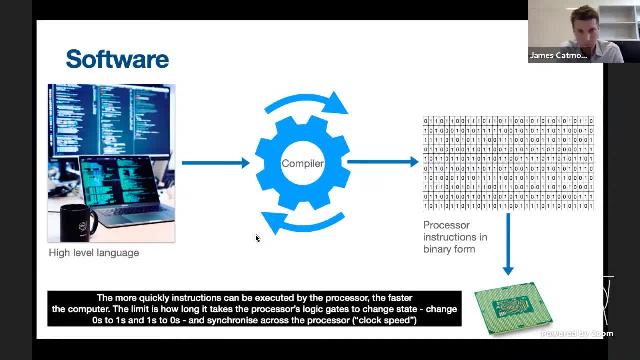 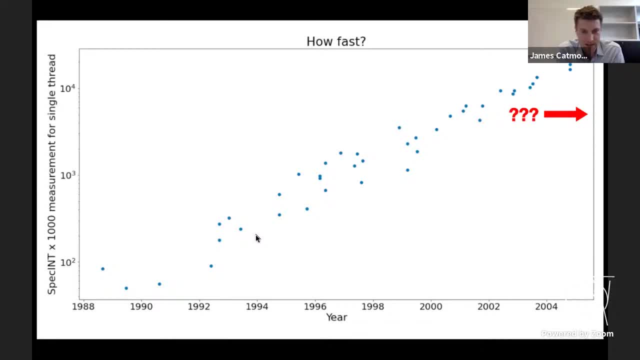 processor. It has this many gigahertz or whatever. Now if we talk about how fast the processor is, again, if you look at this plot, you will see a similar effect. that say, from 1990, mid-1990s. 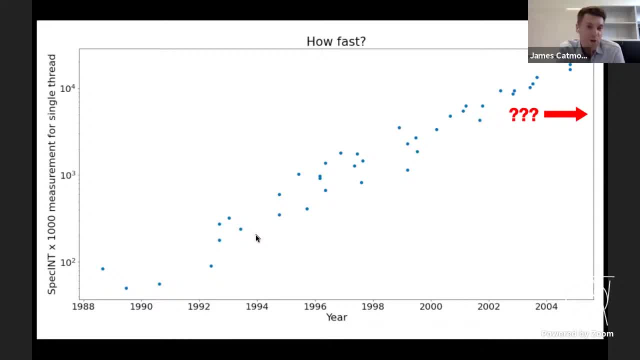 early 1990s to the early 2000s the computers roughly got something like 100 times faster. But then you'll see I stopped at 2004.. And it's kind of a good rule of thumb that if somebody draws a plot like this where the data is mysteriously chopped off, 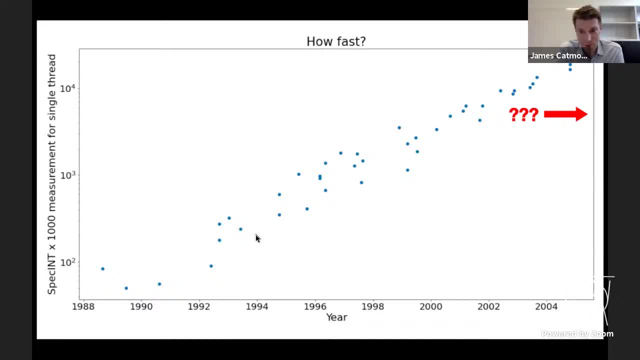 for an unknown reason, the person who made the plot probably knows what the data is, And so the person who made the plot probably knows what data is lying beyond the limit, And they don't want to show it you because it somehow undermines their argument. And this is the case here because 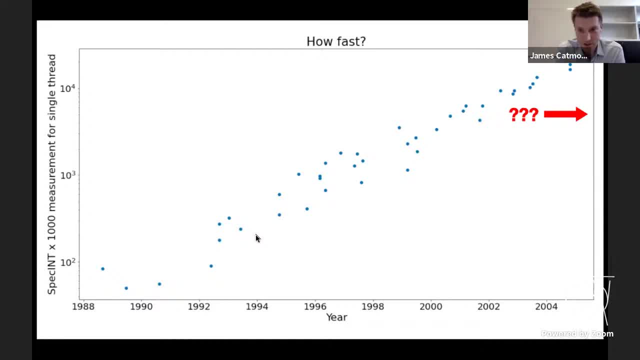 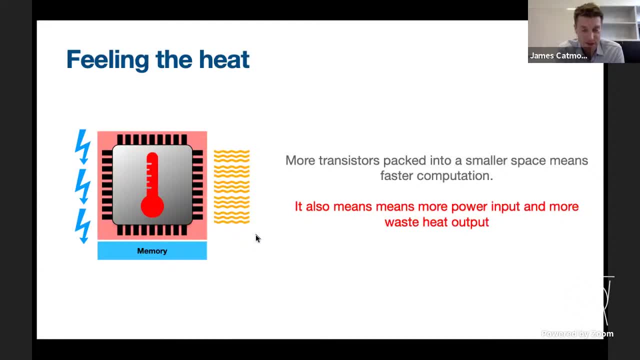 in fact, after the mid 2000s the speed of a single computer processor stopped getting faster at the rate that happened earlier, And the reason for this is kind of slightly mundane. There are several reasons, But the main reason is just to do with heat. 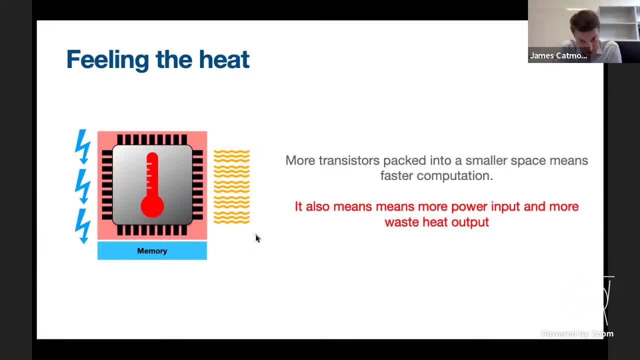 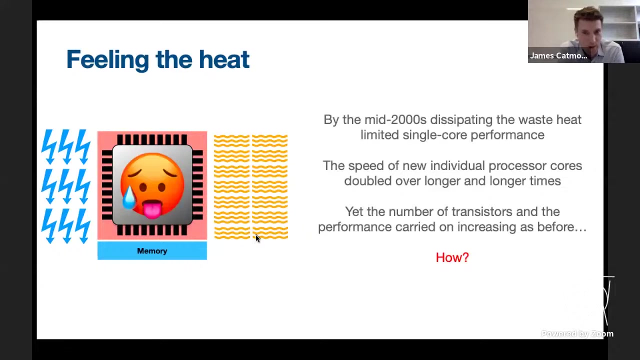 You have to put more electrical power into the chip in order to drive all of those transistors. And the more power you put in, the more heat, the more waste heat comes out, because this energy has to go somewhere And, by the mid 2000s, dissipating all of this waste heat. 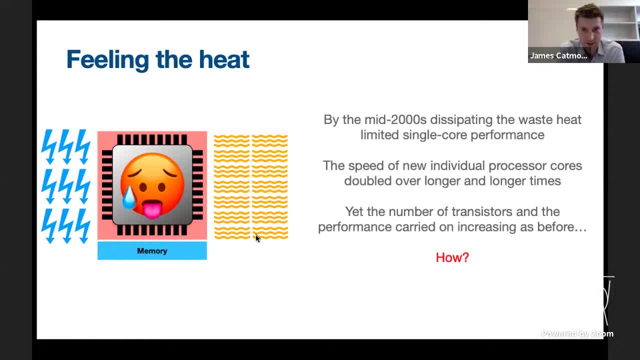 limited the performance of a single computer processor core. The time it took for the speed to double was taking longer and longer, So they weren't getting faster anymore. But yet we don't notice this in our daily lives. Computers seem to get more and 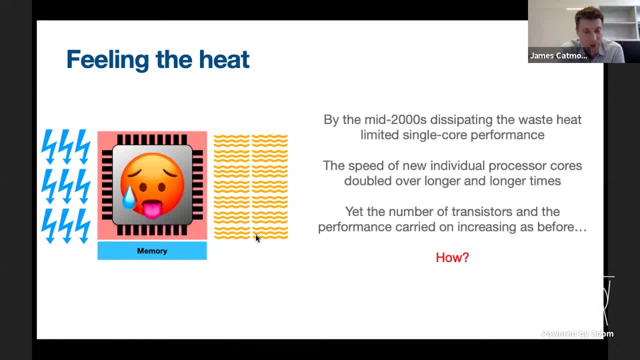 more powerful all the time. And you can ask how is this possible? The number of transistors has kept going up, as I showed you on that plot. So how is it possible that they can get faster and faster still even though we have this limit of heat? And the reason is that modern computer processors 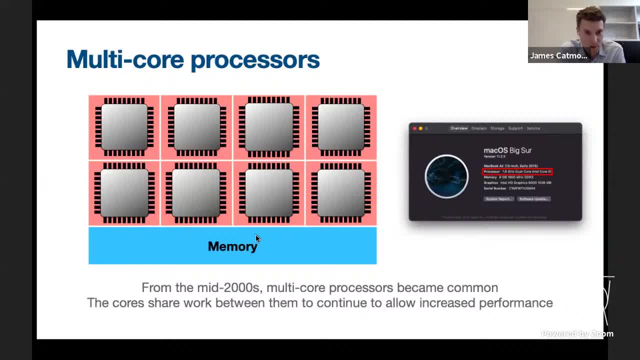 have more than one core. So there are a number of transistors that have more than one core. So there are a number of transistors that have more than one core, And the reason is that modern computer processors have more than one core, And the reason is that modern computer processors have more than one. 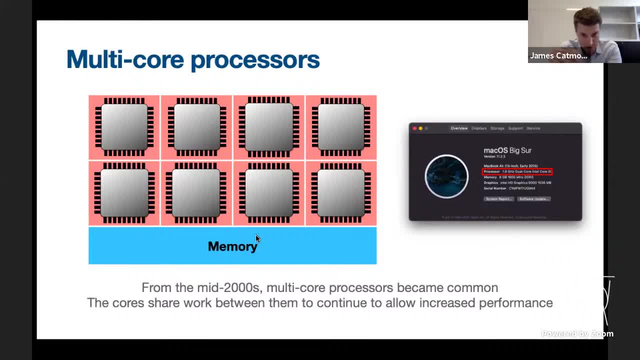 element of the processes that are working through these instructions, these mathematical problems that they're solving, And between them, the cores share work to allow them to continue to have increased performance. And it's highly likely if you look at your laptop, if you get the information. 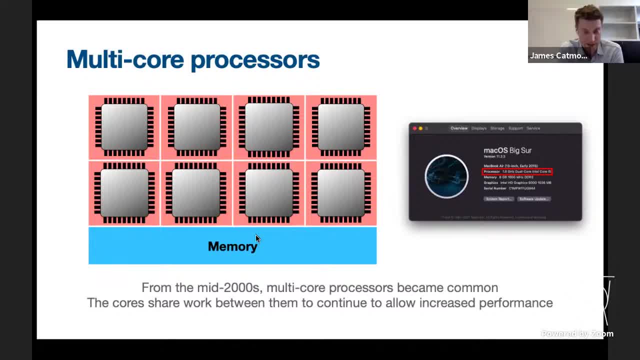 about your laptop or any computer that you've got, you'll see that it probably has more than one core in there. So that's how we've been enabled to continue. Computers have got to continue to get more and more powerful, even though the performance of a single core has not been getting. 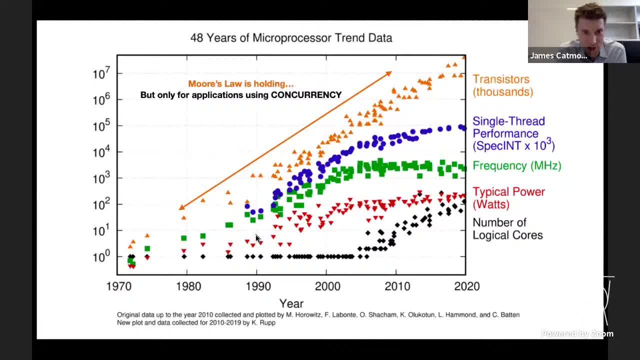 faster, And you can see this from this plot that I'm showing now. It's quite a lot to digest, But if you look at the orange triangles, this is showing the number of transistors. That's the data I already showed you a few slides ago And you can see that carries on going up according to this. 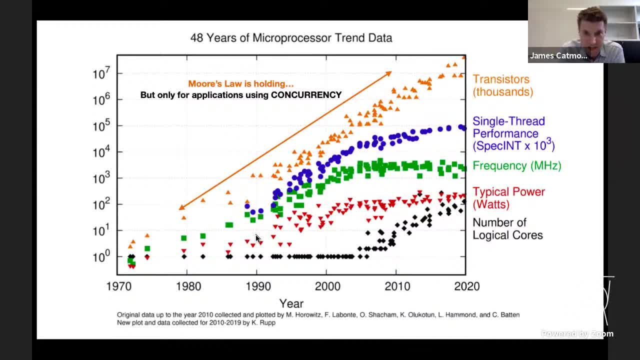 Moore's law. But you can see that the speed for a single computer processor has started to level off And this clock speed, the frequency that I mentioned, has also leveled off after the 2000s And the power in red that it consumes also leveled off for the reason of heat that I mentioned. 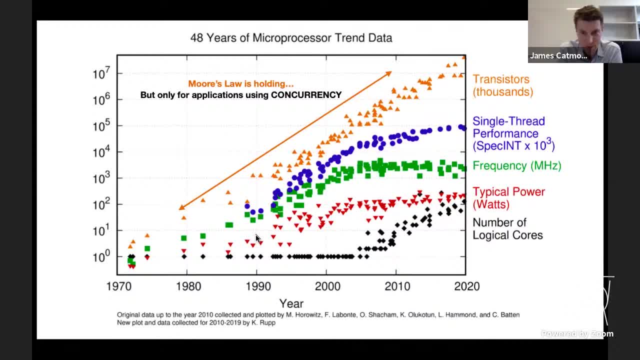 earlier, And then you can see at the bottom these black points. the number of cores has been going up increasingly since the mid 2000s, And this is how we've managed to make computers continue to get faster and more performant. But this can only work if the applications, the programs that people 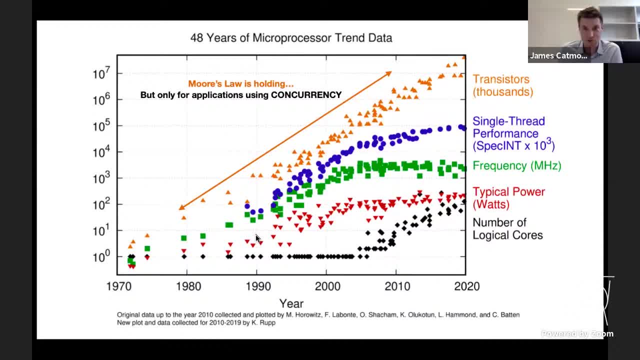 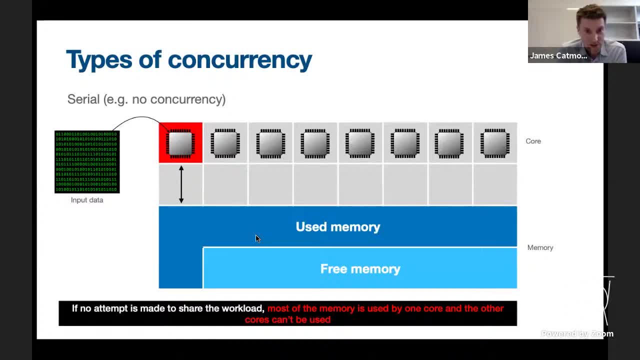 them are able to use all of these cores together, And that's been extremely important for Atlas in the last few years. So if you don't use what we call concurrency, using more than one core at once, what you find is that if you just set one of the cores to do the work, it needs a certain 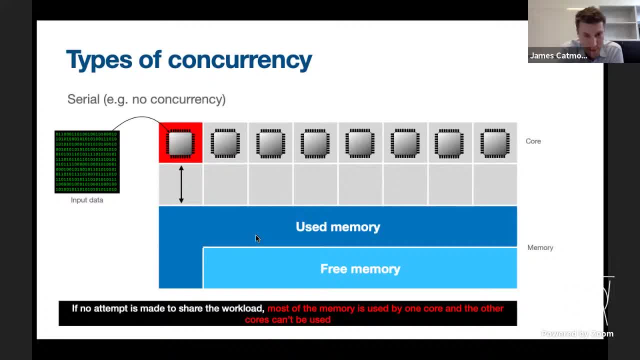 amount of memory to do the tasks. The memory is connected to the core And in order to do the task it needs, it uses up almost all of the available memory. And then there's no spare memory left for any of the other cores to work on the problems. So you are wasting seven of the. 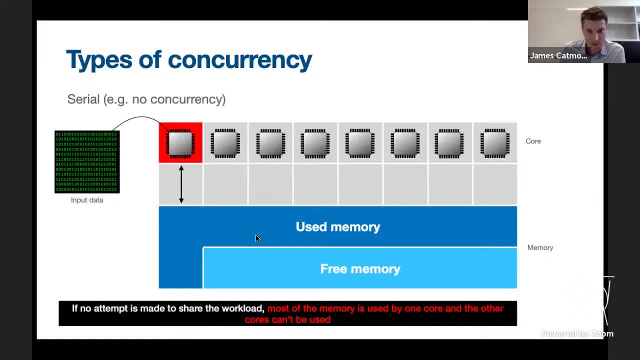 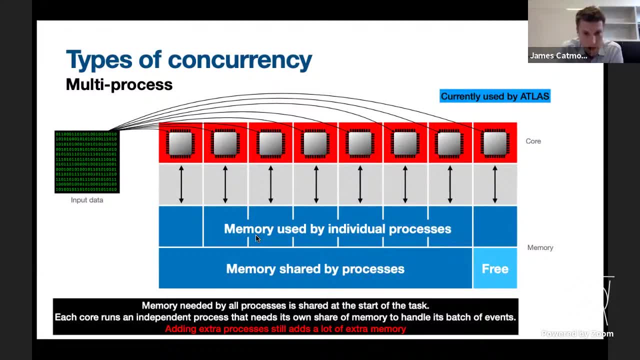 cores, Only one of them is able to do the work, because there's only enough memory for one of them to do the task. Now, the kind of software that we currently use in Atlas is called multiprocess, And here what happens is at the beginning of the computing task, data is dispatched to all of the 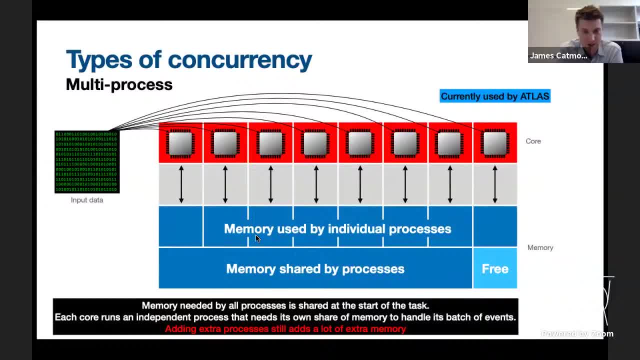 cores. So all of them work on the problem And they share a certain amount of memory that they need to do the task at the beginning. They still have to have a certain amount of memory assigned individually to them, which still means that we can't add many extra cores. So it's still expensive in memory to add additional cores. So 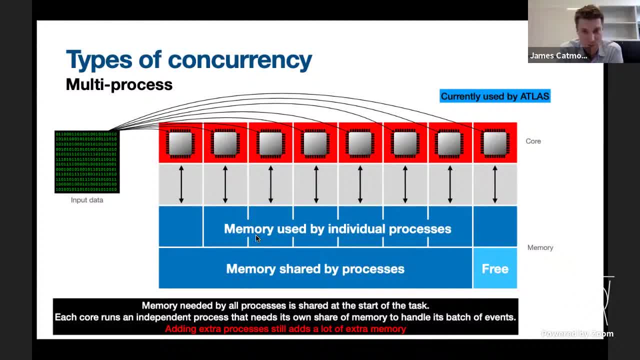 this is still limiting, but at least it means we can make use of all of the available cores, as long as that number isn't too big. So in this diagram here I'm showing eight. And then the kind of software that we will use is called multiprocess, And that's the kind of software that we will. 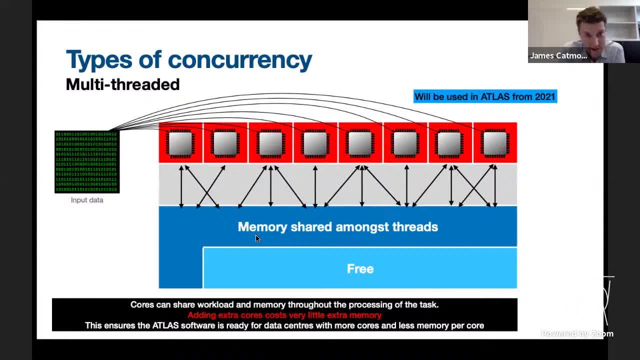 use from 2021 is called multi-threading. This is much more sophisticated and with multi-threading, the memory is shared all the way through the computing task, and this means that adding extra cores takes far less memory. It means that we can add extra cores very cheaply, by which I mean they. 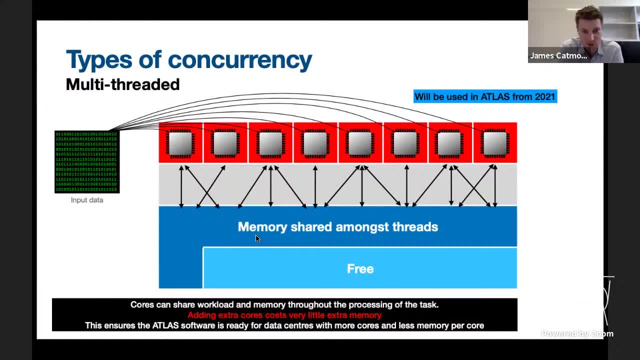 don't add very much extra memory, and this means that the software is ready for data centers that provide large numbers of core but not very much memory- extra memory per core. So this is how we will be working in Atlas from 2021.. This has been a big part of our work. It turns out that writing. 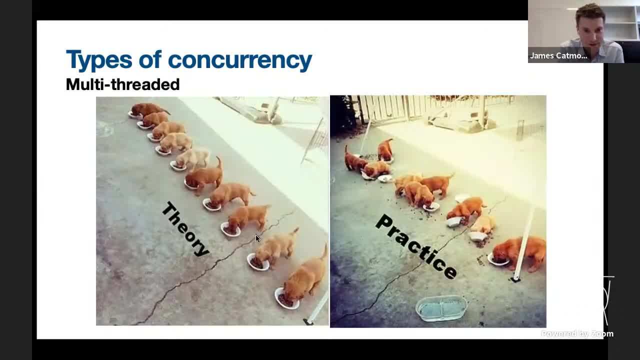 this kind of multi-threaded software is really quite difficult and there's a very well-known meme that goes around computer programmers that the theory of multi-threading looks like you have on the left hand side and the practice of multi-threading looks like you have on the right. 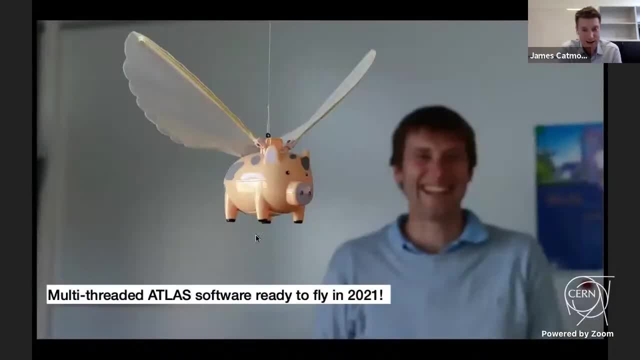 hand side. This is a bit of a joke. We even had a joke about this in Atlas, because my predecessor as computing coordinator put this flying pig on the ceiling of our office at CERN and said that once the software was able to run multi-threaded, we would switch this pig on and it would fly around. 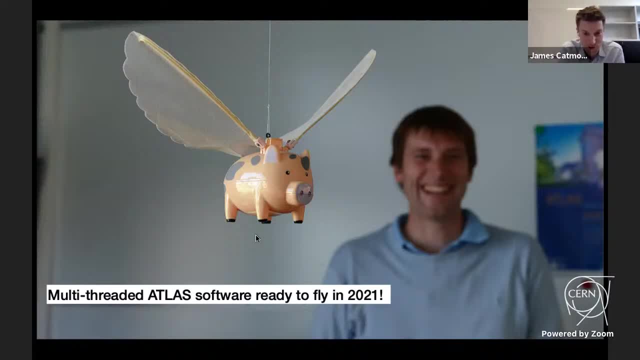 the office and I'm very happy to say that, because of the work of hundreds of people, the multi-threaded Atlas software is now ready to fly. So this is very good news and we're very happy that we've been able to get to this position. 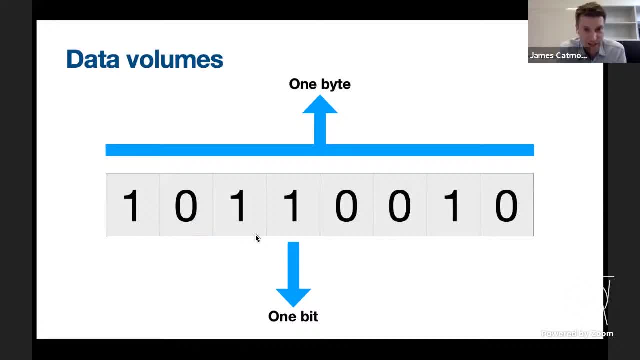 So I now want to say for a few minutes something about data volumes. So you may have heard terms about bytes and bits, so I'll tell you briefly what these are. So one bit is simply a one or a zero. It's a signal in the in the processor, in these logic gates, that a switch should either be on or 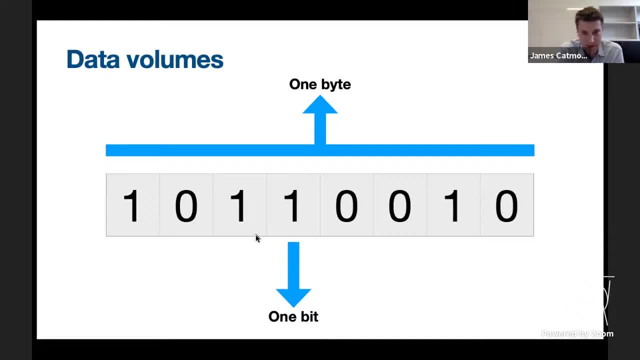 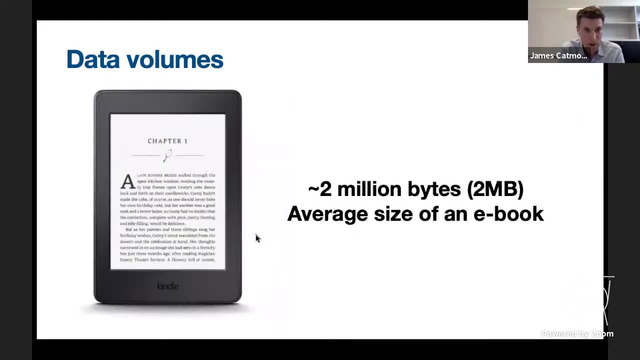 off, and if you put eight of these together, that makes a byte and that is the number of bytes. that is the basic unit of data storage, of data memory. Now, if you have an e-book on your Kindle or your iPad or whatever, typically this e-book is around two million bytes, or around two megabytes, not the 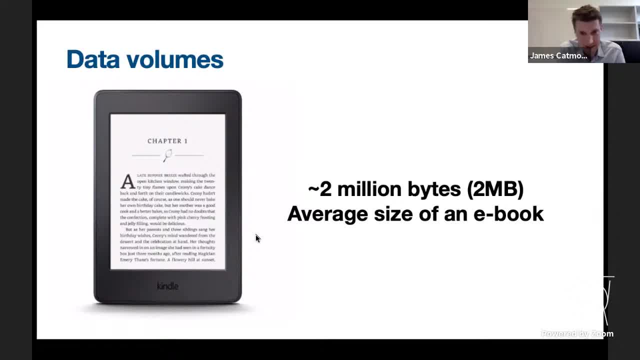 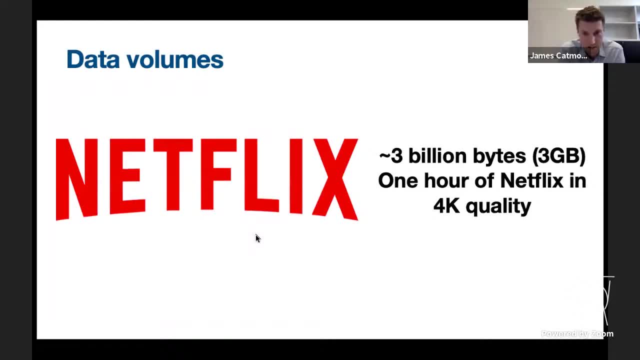 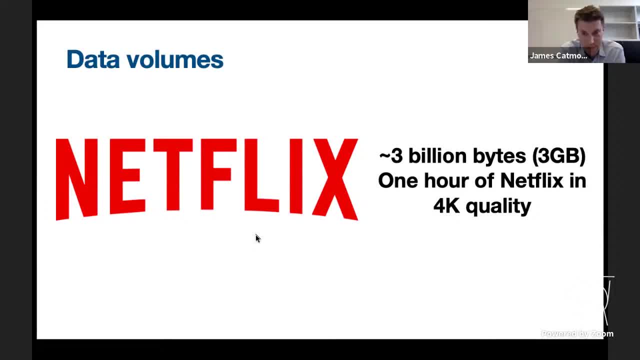 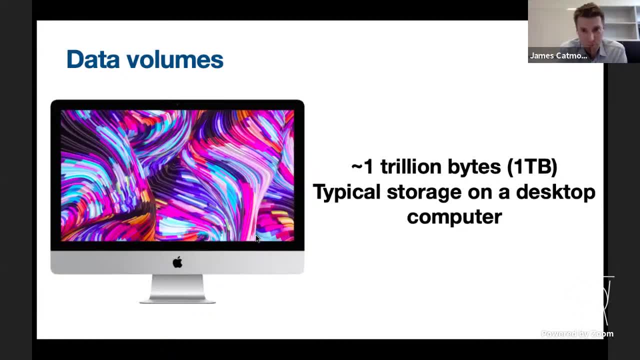 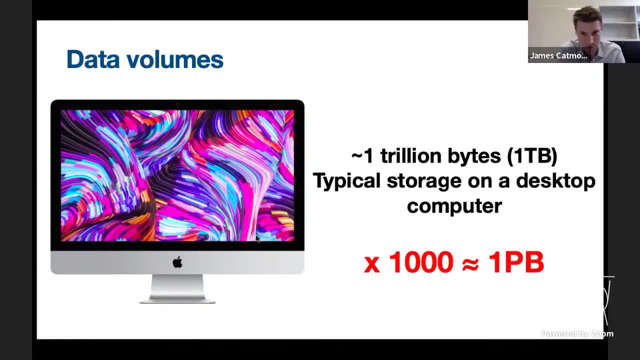 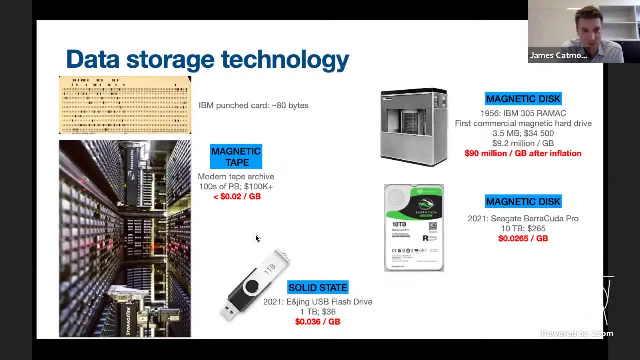 is about 1,000 desktop computers worth of storage. The technology that we use to store data has improved enormously over the years. It all began with IBM's punched cards, which could store around 80 bytes, And the first magnetic disk storage system came out in 1956. 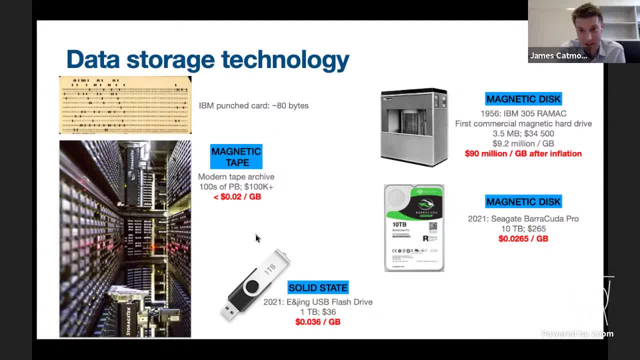 And it could store 3.5 megabytes. So that's just one and a half e-books on your Kindle, And it costs $34,500, which after inflation, is about $90 million per gigabyte. Magnetic disk from 2021, which can store 10 terabytes, costs $265,, which then means it's 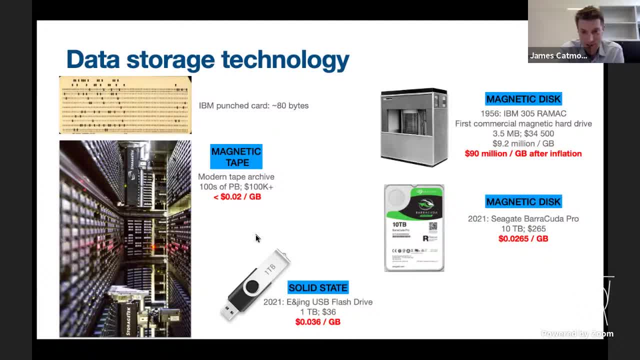 about 2.6 cents per gigabyte, So you can see how much cheaper magnetic storage has become. The very best kind of storage is solid state. This is very fast, but it's a bit more expensive, So you would pay, for instance, something like 3.6 cents per gigabyte for solid state storage. 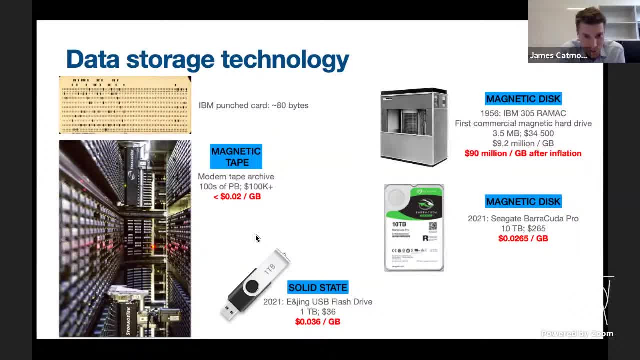 And that's kind of like a flash drive that you might plug into your computer, for instance, And you might be surprised to hear that we actually still use magnetic tape as well. It looks very different from these kind of old school reels that you might have seen in old pictures. 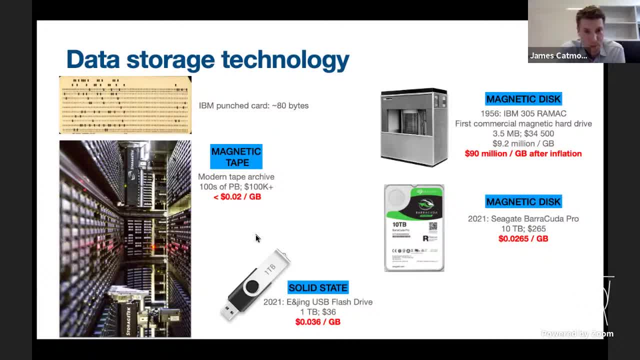 And we use this for storing enormous amounts of data. So, although a modern tape archive might cost more than $100,000, they can store hundreds of petabytes, And this is the cheapest. It comes to about 2 cents per gigabyte. 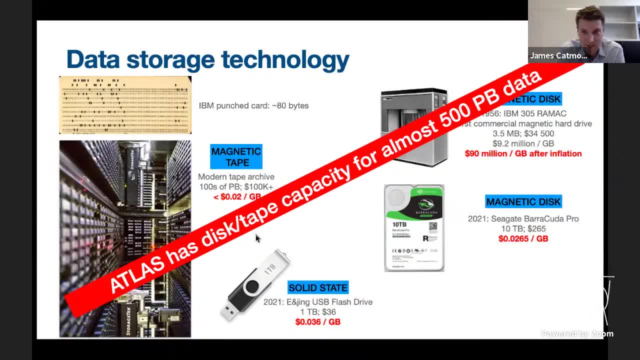 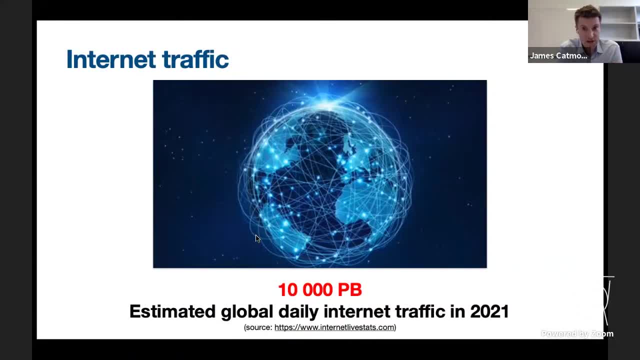 And in Atlas we have about the disk and tape capacity for about 100 petabytes of- sorry, 500 petabytes of data. And just to finish off this introduction to computing, to give you a sense of how much internet traffic is being moved around the world, 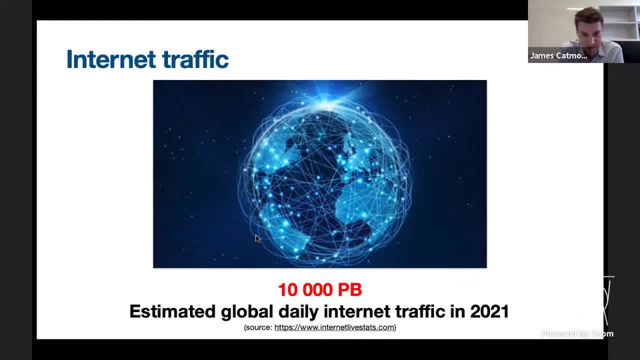 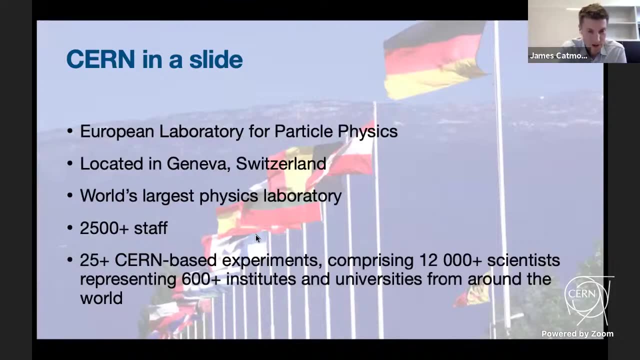 roughly every day. around 10,000 petabytes are beamed around the internet by fixed telephony and data And also mobile data. So that puts everything into context. So I'm now going to change topics slightly and talk a bit about CERN and Atlas. 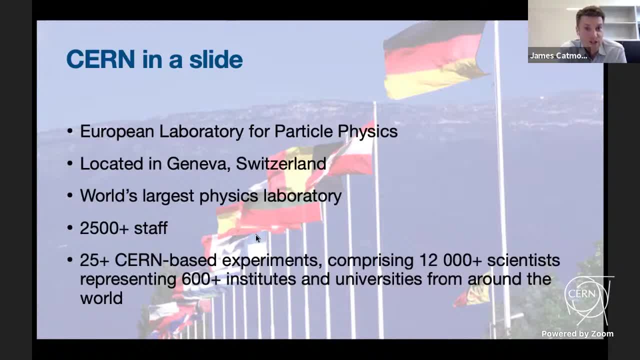 before I bring the two topics together, So in one slide. CERN is the European Laboratory for Particle Physics. It's located in Geneva in Switzerland. It's the world's largest particle physics laboratory. It has 2,500 staff who are actually employed by CERN. 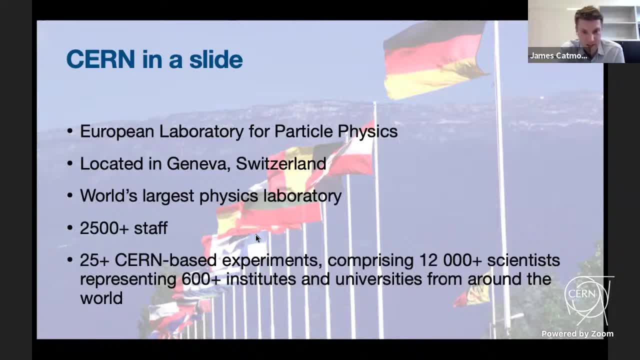 But then there are more than 25 CERNs- They're CERN-based experiments- And together there are more than 12,000 scientists representing more than 600 institutes and universities from all over the world, who either can work at CERN or they are using CERN facilities. 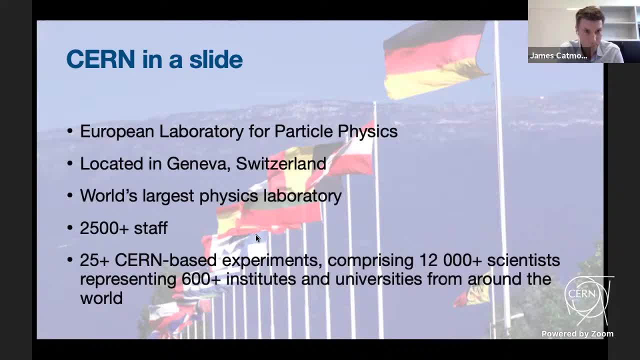 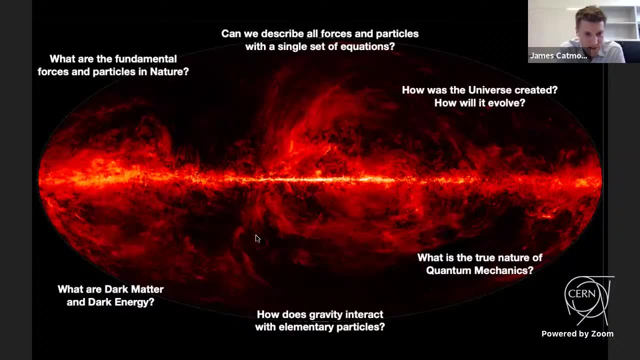 but working in other countries, like I am, And the questions that CERN is seeking to ask. I'm just going to show these on one slide, but you can look at the other YouTube videos to find more about this. Questions such as: what are the fundamental forces and particles in nature? 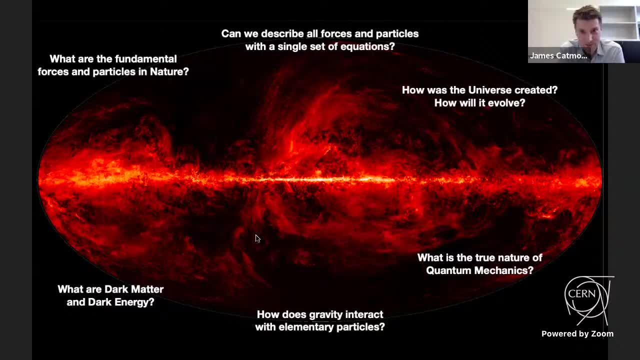 Can we describe all of these forces with a single set of mathematics? How was the universe created? How will it evolve? What's the true nature of quantum mechanics? How does gravity fit in with all of these different elementary particles? And what are dark matter and dark energy? 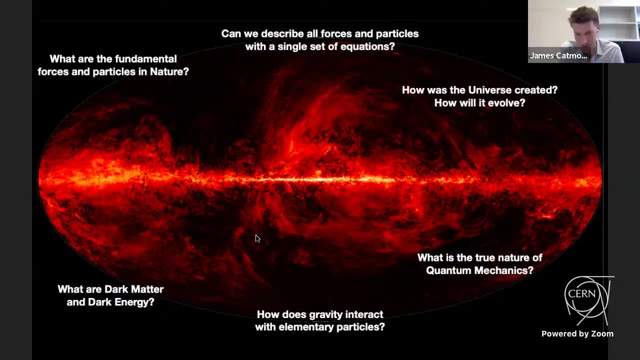 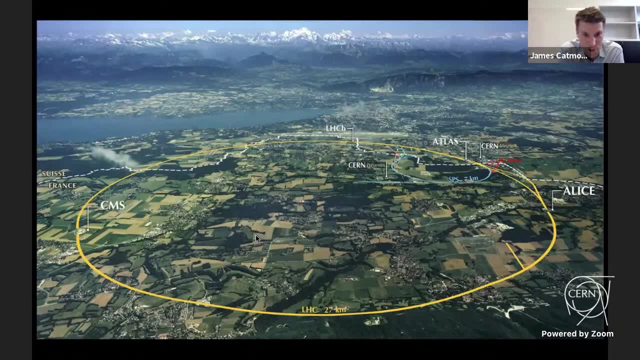 This is why we're here. These are the questions we're trying to ask, And this is CERN's pride and joy. It's the Large Hadron Collider. It's a particle accelerator 27 kilometers in circumference. This is an aerial photograph. 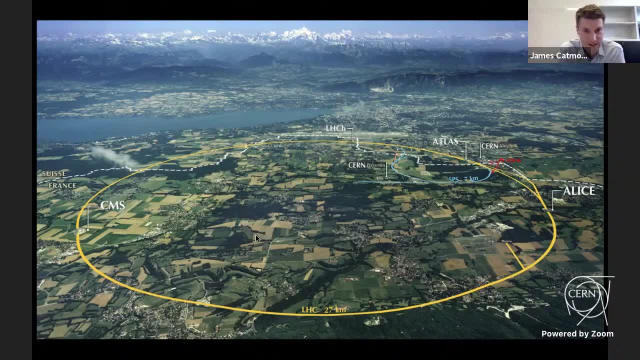 You can see the Alps in the far background, Lake Geneva slightly nearer And you can see this. You can't see very much of the accelerator above ground because it's 100 meters underground, But there are four experiments located at four points where the beams of particles collide. 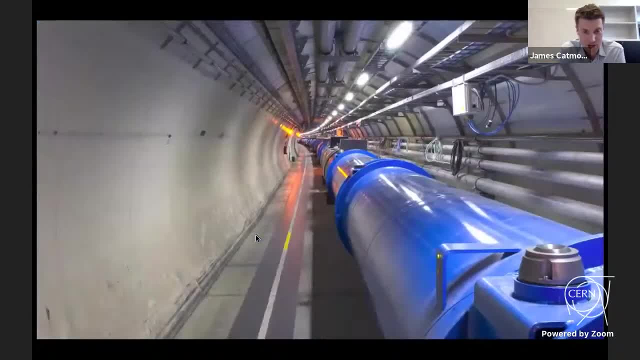 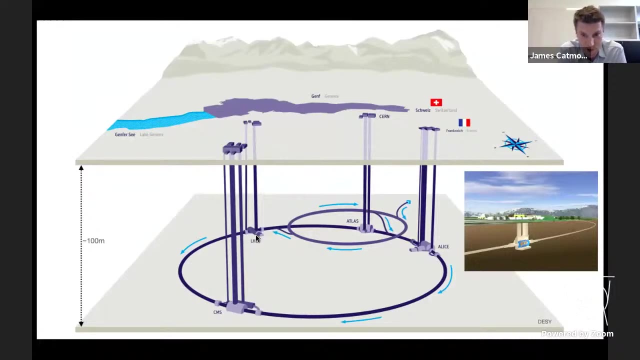 This is the kind of iconic shot of the Large Hadron Collider tunnel. The blue object is one of the magnets which we use to steer the particles around the accelerator. This is a schematic to show how it actually looks in more simple terms. So, as I said, it's 100 meters underground. 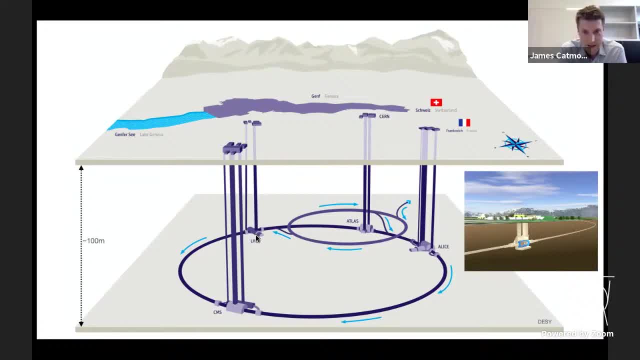 And you have these four experiments at this: LHCb, CMS and ALICE, which are spread out around the ring, And this schematic in the corner, the small one sort of, shows you the scale in a more realistic sense, how deeply buried the experiments are. 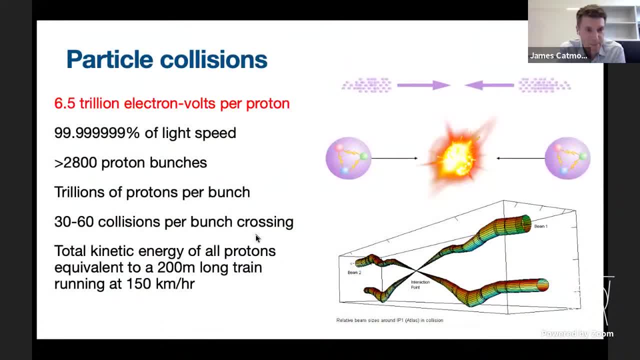 So the collisions that are occurring, each beam, each proton in the beams, the colliding beams of proton have what we call 6.5 trillion electron volts worth of energy. That means that they're going at 99 point, many, many nines percent of the speed of light. 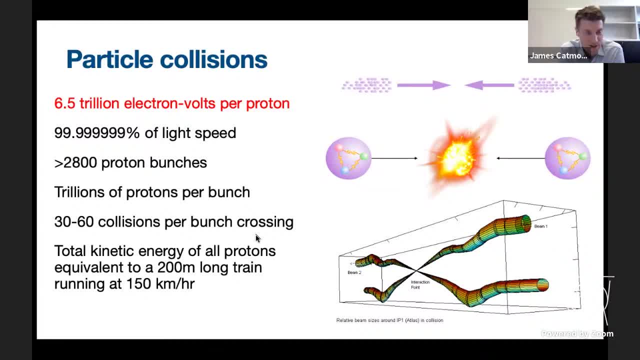 In each. we have the protons move around the accelerator in bunches And there are around 2,800 bunches of protons there. There are trillions of these protons in each bunch And every time these bunches cross through each other. 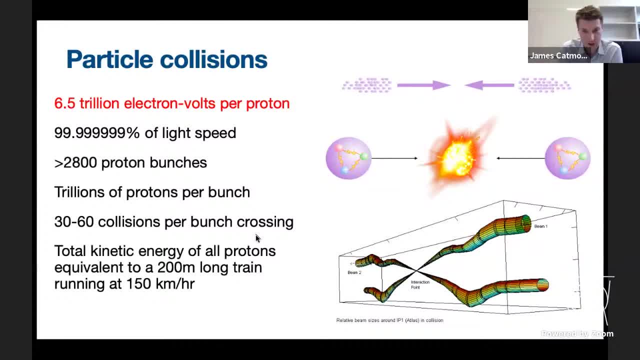 between, say, 30 and 60 pairs of protons. the protons collide, If you're interested. the total kinetic energy of all of those protons, if you add them all up, is about the same as a 200 meter long train running at about 150 kilometers an hour. 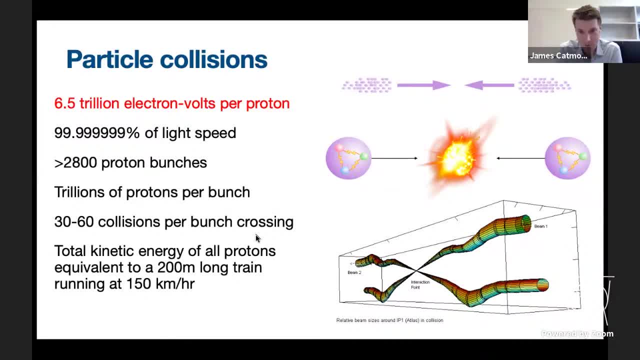 When the beams are going around the accelerator, they're about the thickness of a human hair And, as you can see in this sort of diagram in the bottom corner, they are really brought into a very, very tight focus when they're collided, to ensure that as many of them collide as possible. 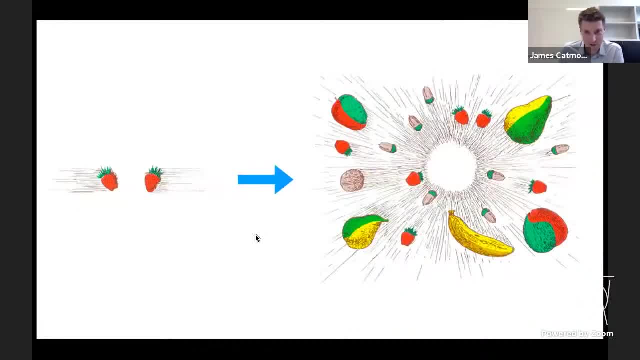 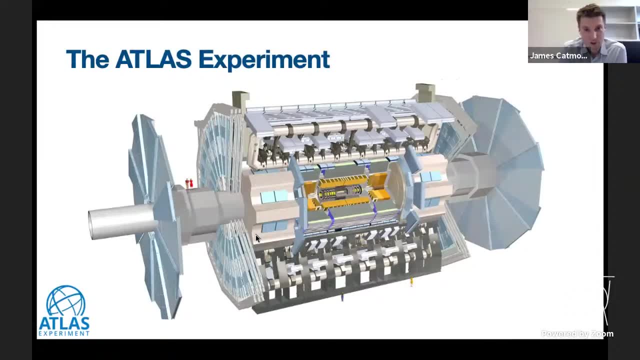 So a sort of humorous way of depicting this is shown here. This is a very old picture, from the 1970s, but it's I still quite like it. So I'm going to talk about Atlas. So in one sense, Atlas is a machine. 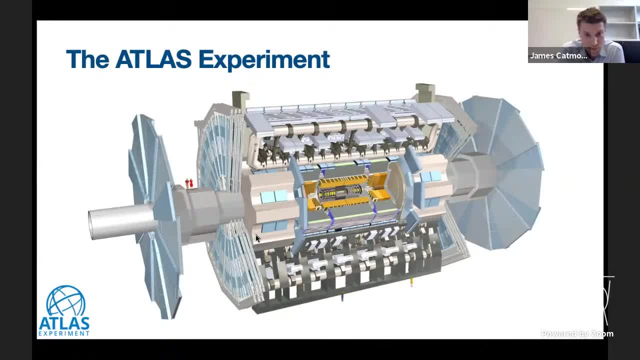 It's a. it's a particle detector. It's very, very large, 44 meters long and 18 meters high. You can see a cutaway image of it here. The particles arrive in the bunches from either end and they collide in the center. 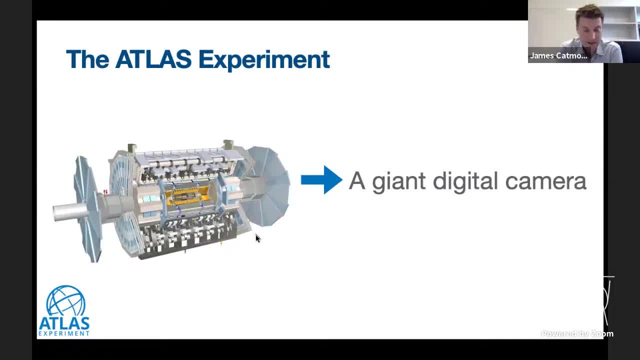 So the easiest way to think about the particle detector- a particle detector like this- is that it's a giant digital camera, but it's a giant digital camera with a difference because it's in 3D, And it's also a digital camera that can detect charged particles as well as photons which carry light. 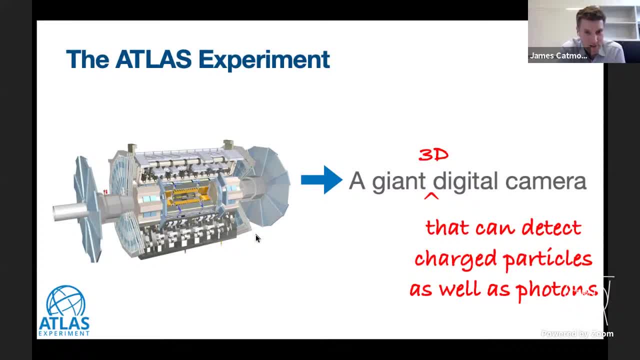 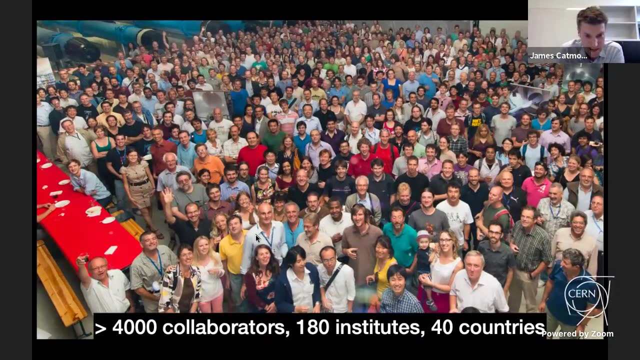 So that's the easiest way to think about a particle detector. It's a. it's a giant digital camera that can take in quotes, photographs of the collisions that are occurring inside the inside the detector. But equally as important, Atlas is also people. There are more than 4000 of us in Atlas and a similar number in in our opposite number, CMS. 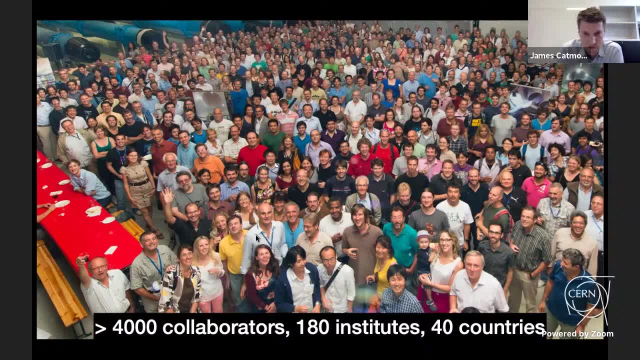 It's made up of one hundred and eighty different institutes, universities and labs across 40 countries. This picture was taken shortly after the discovery of the Higgs boson. This is a celebration we had. I think this is the biggest gathering that Atlas had. 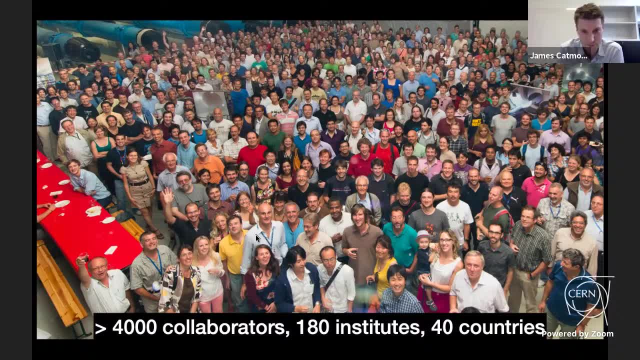 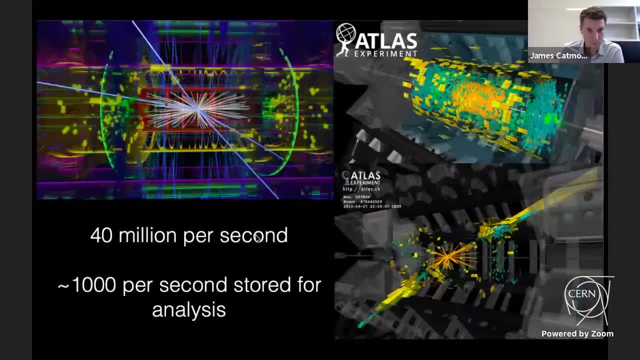 But even in this picture there's only a tiny fraction of the total number of people on Atlas. So Atlas is a detector, But equally or more importantly, it's also people. So these collisions occur in the center of the detector around 40 million times per second. 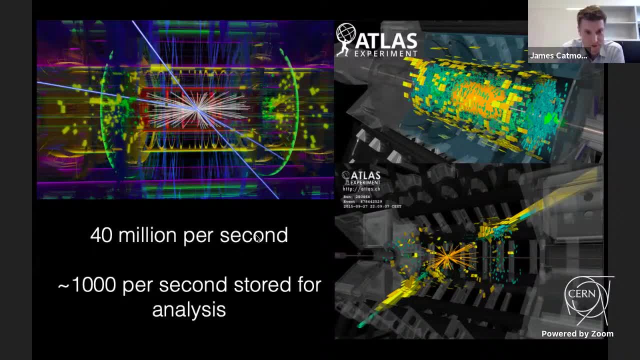 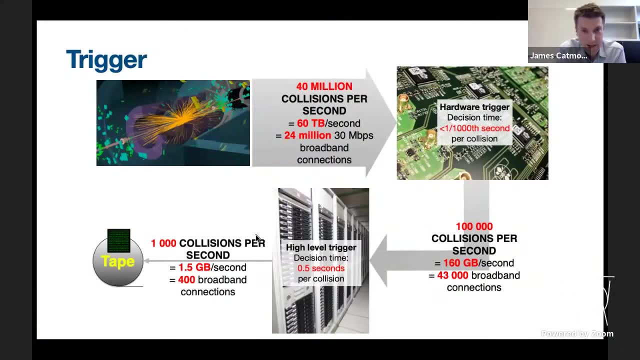 And we only store around a thousand of these per second for analysis, And the way we do this is by something called a trigger. Now, 40 million collisions per second equals something like 60 terabytes a second, And that's kind of the same amount of data that a small country. 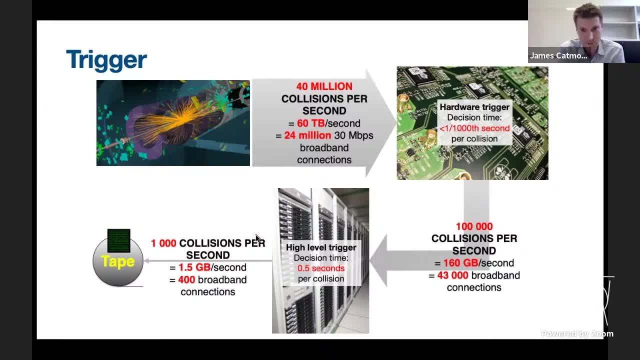 A small country's worth of broadband connections would need to deliver. So of course it's completely impossible to handle that amount of data, And it also turns out that most of that data isn't of particular interest, So we can throw away almost all of this. We do this in two stages. 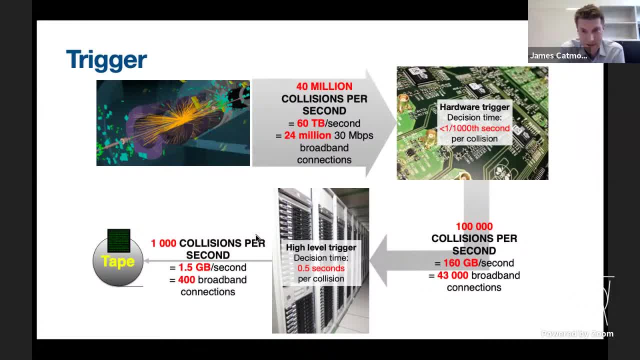 The first is done with hardware, electronics that's based inside the detector And it only has the time of one, one thousandth of a second to determine whether to keep to save the data from a from a collision. This gets us down to about one hundred thousand collisions per second, which is around the number of broadband connections in a small town. 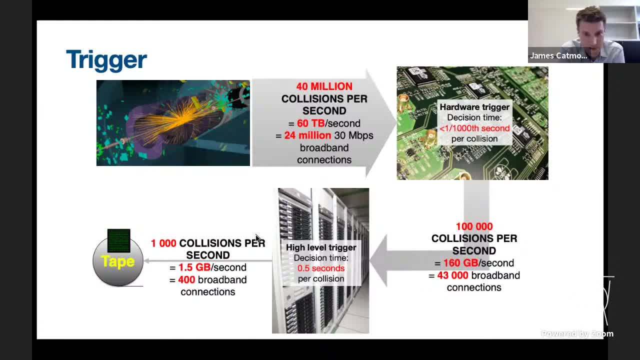 And we have a bit longer to deal with this. So we get the data out of the detector itself, We put it onto computers that are nearby the the experiment And we have about half a second to decide whether we want to keep each of these collisions. 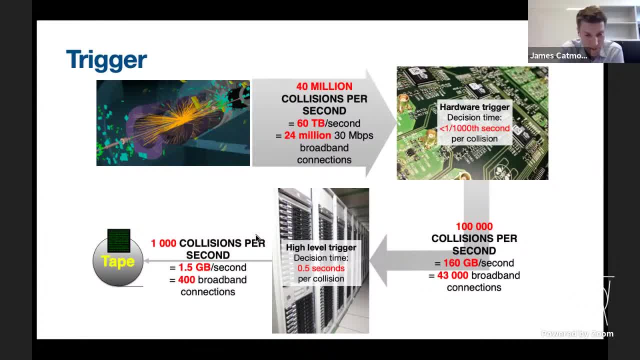 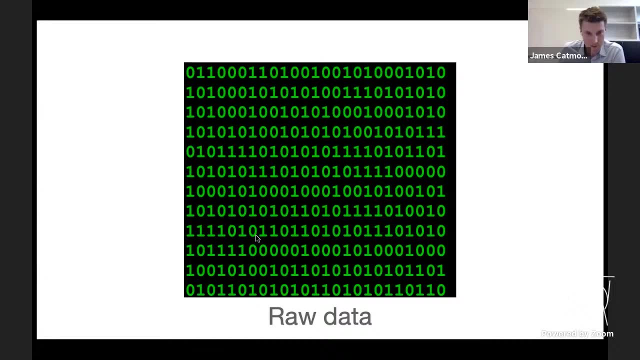 This gets us down to a thousand per second, which is around the broadband connections in a big apartment building, And all of those are stored On tape And this gives us something called raw data, And raw data is literally the data that comes out of the of the experiment. 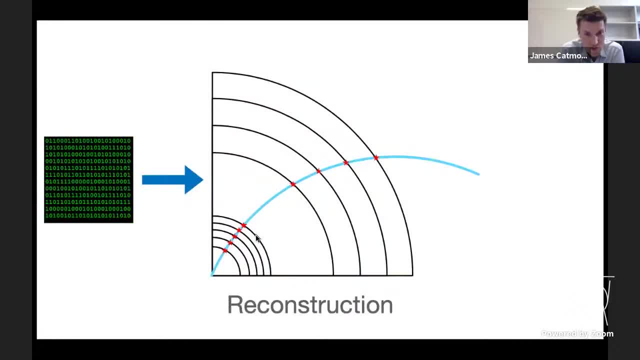 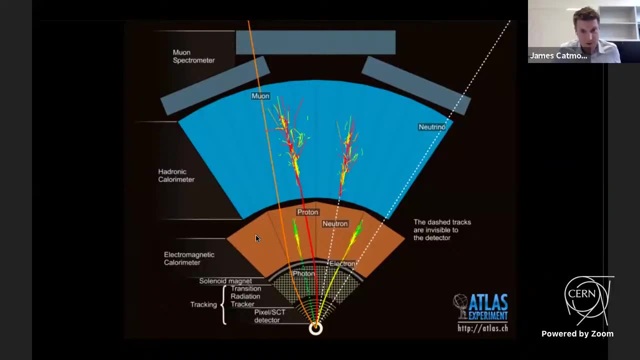 And then we do something called reconstruction to the raw data, And reconstruction is where we rebuild, or try to rebuild, the particles that were emerging from the, from the collision, The detector, as you kind of saw from the picture that I showed earlier. it's a series of layers. 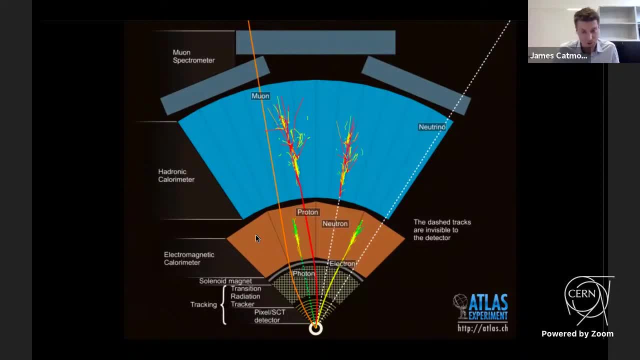 You can kind of imagine it as a, as a series of rushes, And you have more or less three components. There's the middle most part, called the inner detector. Then you have a section in the middle which we called calorimeters, And then there's a section on the outside called the muon spectrometer. 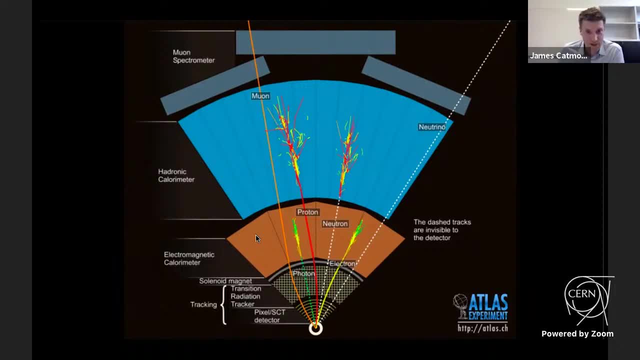 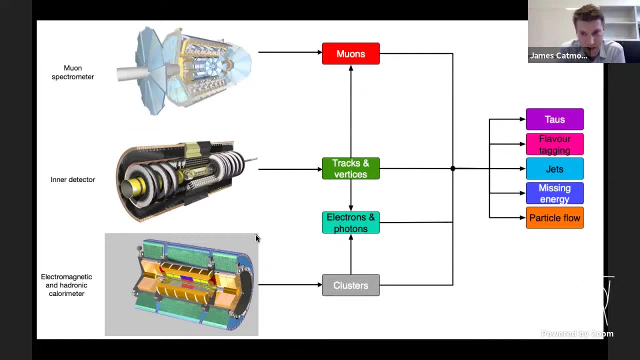 And they all do different jobs and detect different kinds of particle. And in this reconstruction step, what the software does is it merges them together and builds a global view of what happened in each collision. So we take the information from the inner detector, We make this into something called tracks. 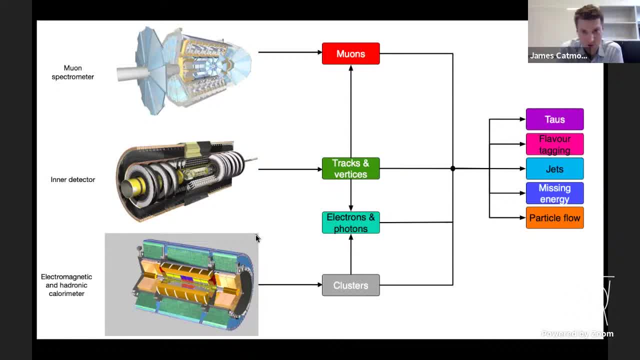 We combine that with information from the muon spectrometer to make muons, which are a kind of particle, subatomic particle. We also use information from this calorimeter system to make electrons on photons, And then these basic objects are then combined to build the more complicated objects that we as physicists actually use to do our analysis. 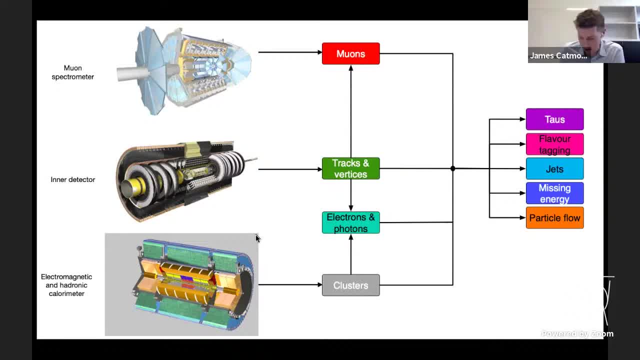 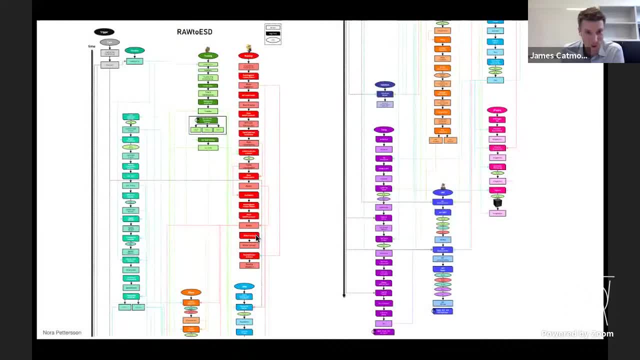 So this diagram maybe doesn't look too complicated. I've actually spared you some of the details, Because on the next slide this is what it actually looks like. It's afraid a bit more complicated than what I showed. This gives you the idea of how this works. 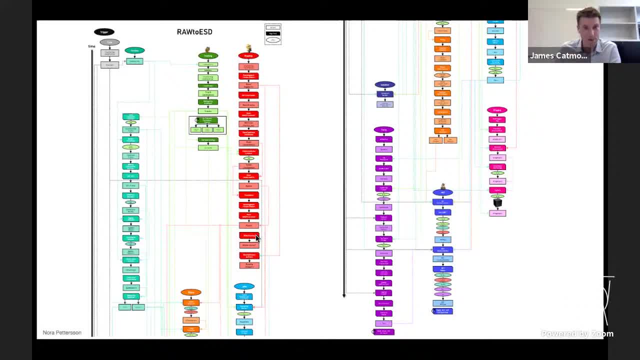 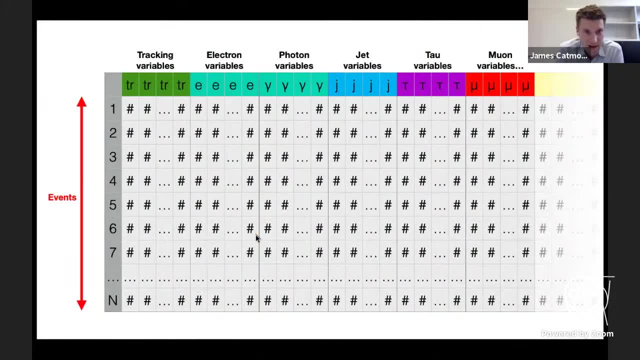 We start off with basic levels of information and we build it up into more and more complicated objects. And the way this data looks to a physicist is it's like a very large table split across many, many computer files. And this table, the columns of the table, are different variables for different kinds of objects. 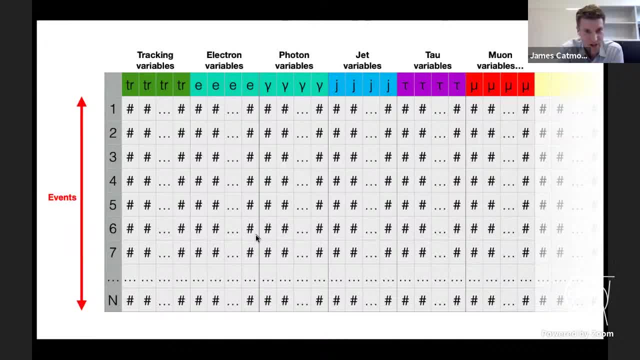 Now you have different numbers of objects in each collision, So the number of columns can can kind of change. But this is gives you the view of what the of what the data looks like. And then the rows of this table are the events. 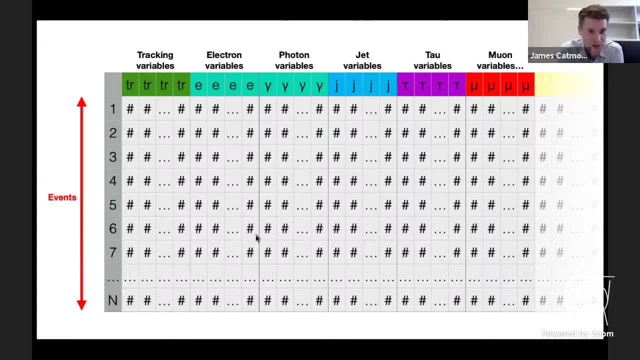 And each row represents a single event. If you read across one row, that gives you all the information about the tracks, the electrons, the photons, the jets and all the other different reconstructed objects, as we call them, that you need that. the physicist needs to do that analysis. 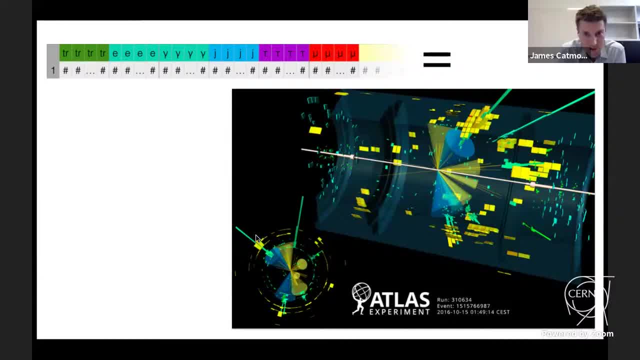 So one row. So one row of these tables of data gives you one of these images. We very rarely look at images like that. We normally just use them for, for essentially giving presentations, so that people can see what the data looks like. Normally we see them, these, as rows of numbers, and one row of numbers gives you one of these, one of these images. 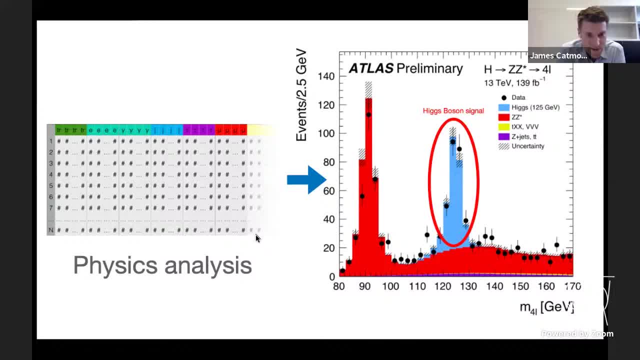 And then the most important thing that we do is is called, or the individual physicists do is something called physics analysis, where we look at these tables of data And we process these into and through us through a process called physics analysis. This is done by individual physicists. 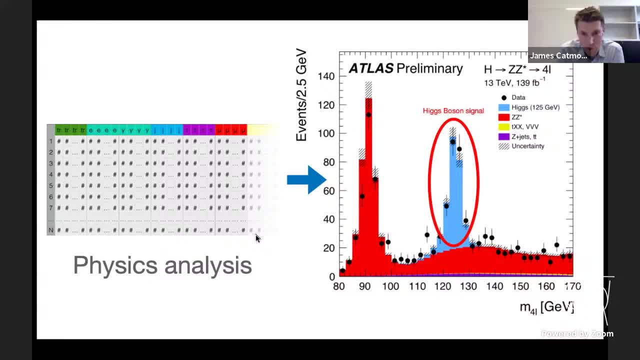 And after many different steps, we produce plots that look like this. This is a particularly famous plot because it shows the famous Higgs boson signal, which is which is is visible here, And to get from the tables that have come out of the reconstruction all the way to the to the plots. 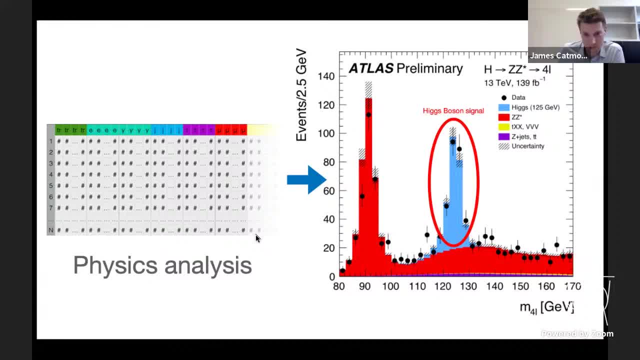 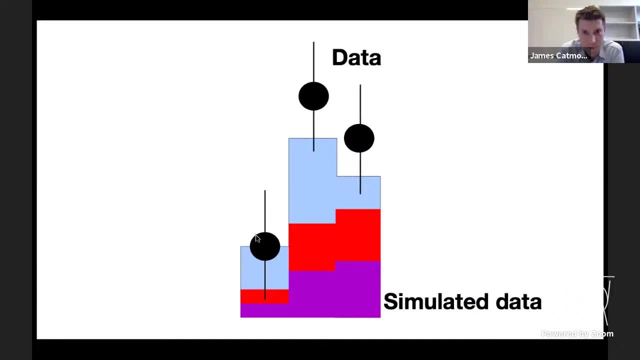 Look like this takes many steps, And I'm going to describe a few of these steps Now. the first thing to note is that there are two kinds of data shown on these plots. There are the black points, which represent data, real data that we've recorded in the experiment. 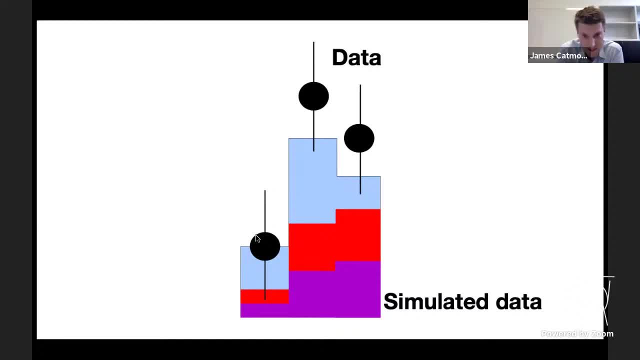 And then there are these colored blocks which are simulated data. We have to simulate data to understand how the detector interacts with the particles, because unless we simulate the behavior of the particles going through the detector, we're kind of lost. We're kind of blind to see how any physics should affect the, should affect how the data looks. 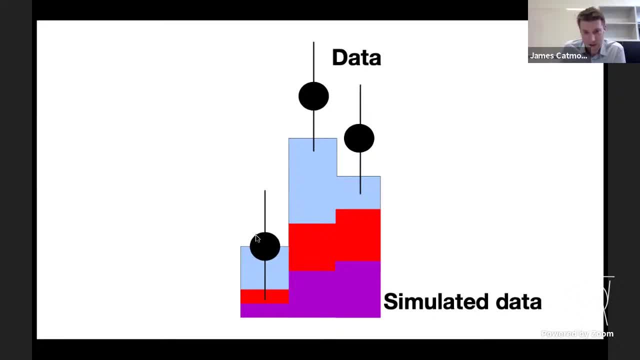 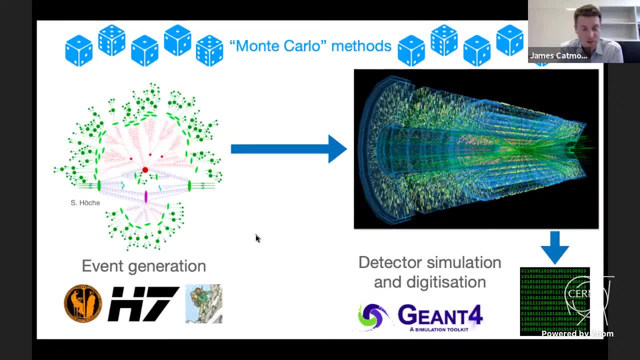 So without simulated data it's very, very difficult to do analysis. So we have to do simulation as well as just recording the data. Now for the simulation. this this is two steps. The first step is called event generation, And this is a kind of computer program that simulates the collision of the particles in the detector. 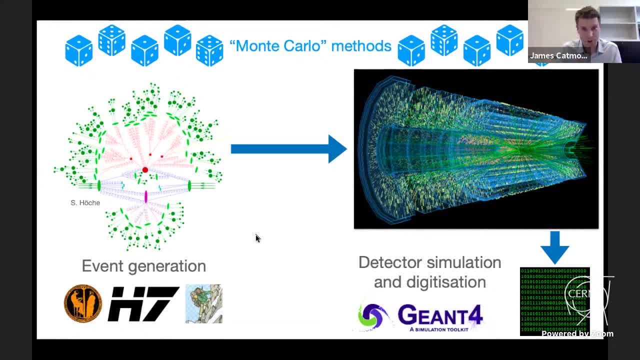 And then the evolution of this collision into the particles That we see as they fly through the detector. And the second step is called detector simulation, where we simulate the interaction of the detector with the, with, with the particles as they fly through it, how they deposit their energy into the detector and how this energy then gets turned into digital signals. 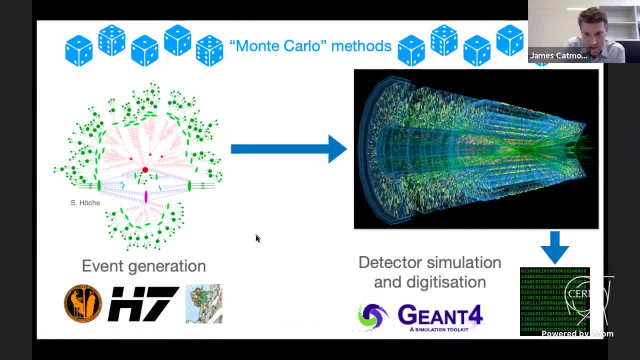 This second part is done with something called digitization, And the output of this looks very much the same as the raw data That comes out of the experiment. Both of these things are done with Monte Carlo methods, which rely on random numbers to produce the to simulate the collisions and the interaction with the with the experiment. 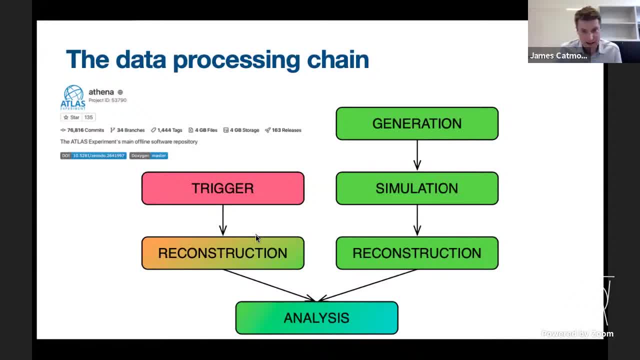 And this means that we have a processing chain that has sort of two legs. The leg on the left hand side is the leg followed by the data, the real data that's recorded by the experiment- And the leg on the right hand side is the is the leg that's followed by the data. 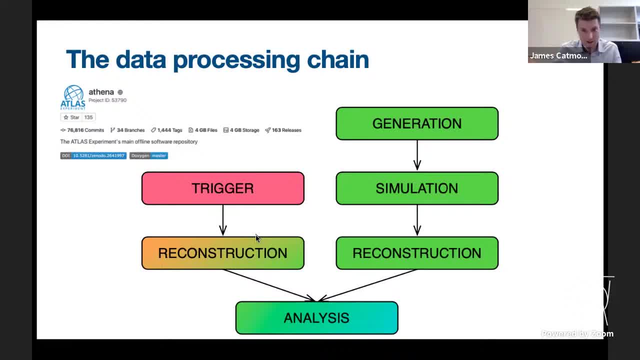 That's followed by the simulated data, And then, in the end, the simulated data and the real data are analyzed together to give you these plots that you saw on the previous slide, where you have simulated data superimposed on on real data. All of these steps, apart from the very last stage of analysis, are done with a data processing framework called Athena, which is Atlas's data processing framework. 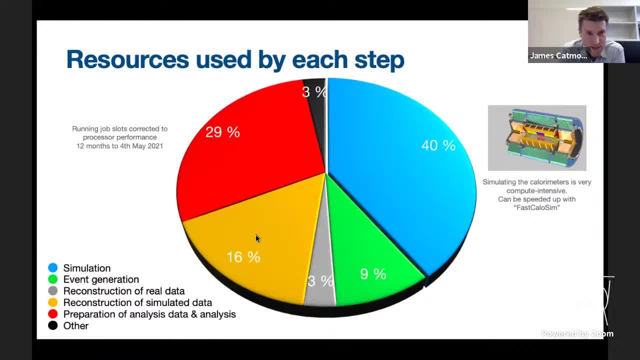 So how much resources are used by each of these steps? Well, you can see this from the pie chart that I'm I'm showing here. What you'll see very obviously is that simulation is the part that dominates. This is what uses most of our computing power. 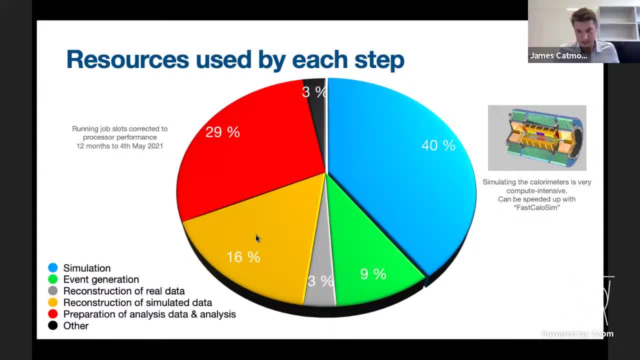 And the reason for this is that simulating these things called calorimeters- This is the middle part of the of the detector which measures the energy- is very compute intensive because there are lots of layers of material that have to be simulated in a very precise way. 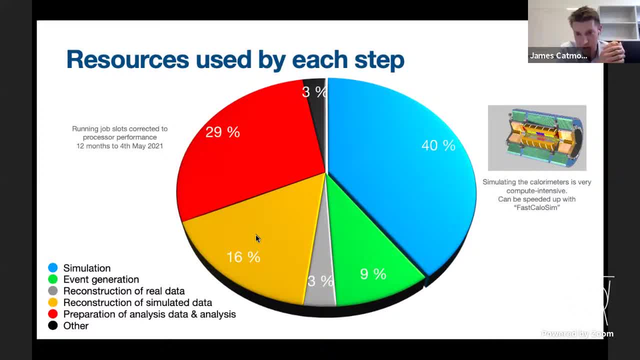 We can speed this up with something called fast color simulation Or fast callous- And I'll say a bit more about that slightly later on- And then you can see the other processes. things like the event generation and then the reconstruction and the analysis and preparation of analysis data take somewhat less. 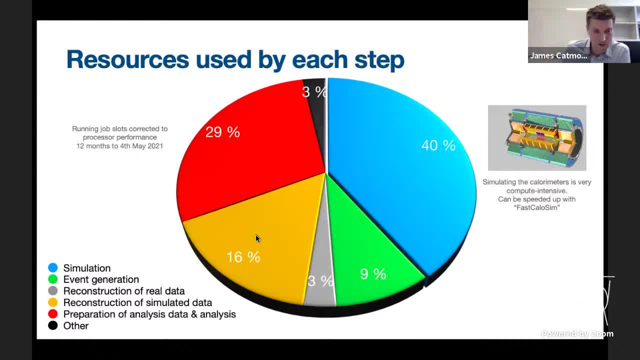 And this gives you an overall idea of of how much computational resources we're using. Now you now be probably asking: what do we actually run all of this computation on? And the answer is: we use something called the Worldwide LHC Computing Grid. 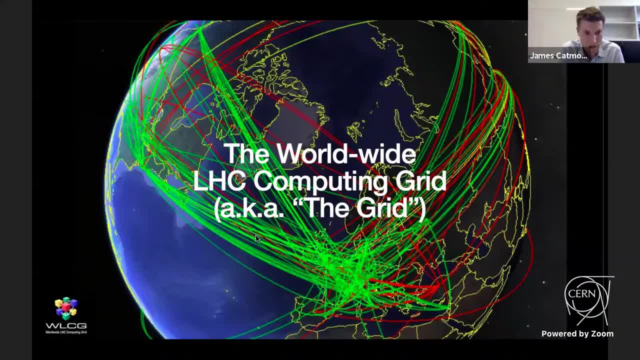 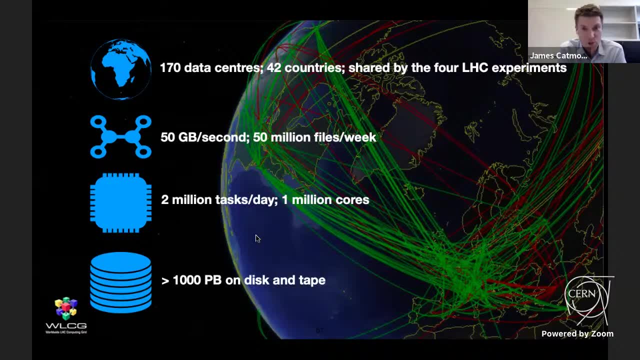 which is known in in our field as the grid. And the grid is a network of 170 data centers spread out across 42 countries. It's shared by the four LHC experiments. It can transfer up to 50 gigabytes a second, which equates to around 50 million files per week. 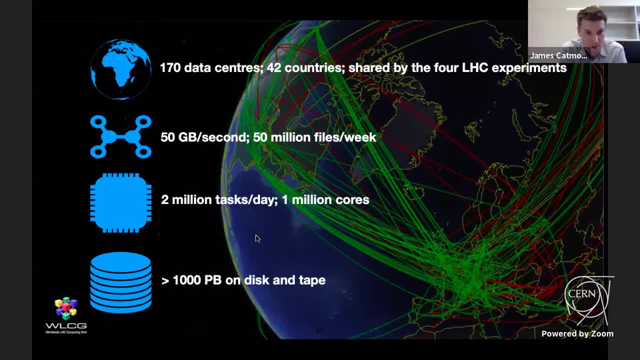 In terms of how much computation it can do, It can process 2 million computational tasks a day On average and it has 1 million computer cores. And in terms of storage, it has more than 1000 petabytes, or, as we call it, an exabyte of storage available on disc and tape which is spread out across all of those data centers. 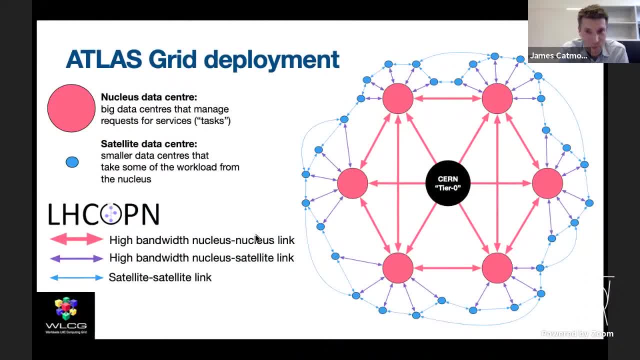 Now the different experiments organize the way they use the grid in different ways, But the way Atlas uses it is that we have two kinds of data center. There's one called nucleus data centers, And these are big data centers that manage The requests for computer services, which we call tasks. 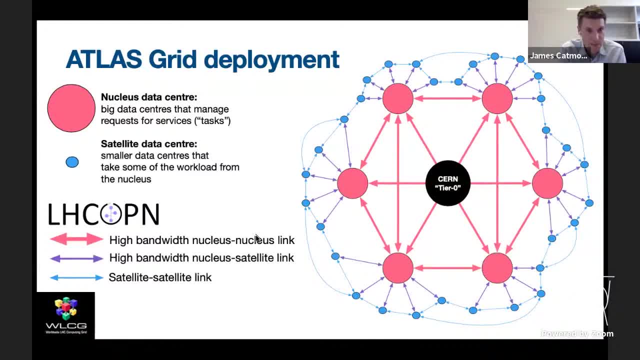 And then there are smaller data centers connected to them that take some of the workload from the, from the nucleus, And the connection between these data centers, particularly the biggest ones, is using a private optical network called LHC OPN, And this is what we use to transfer the data between the different data centers. 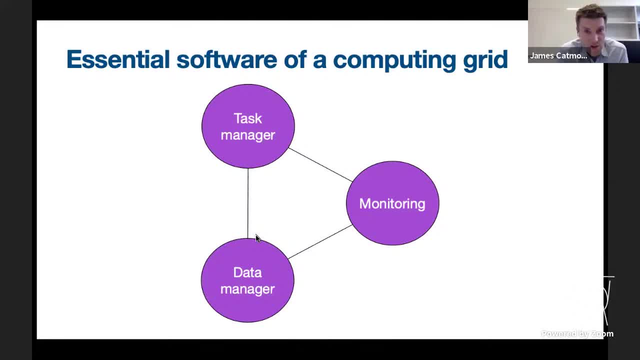 So to drive a computing grid you need three pieces of software. There's something called a task manager, Which is the software that determines what computer tasks should be dispatched to which data centers. There's something called a data manager, which keeps track of what data is stored at the different data centers. 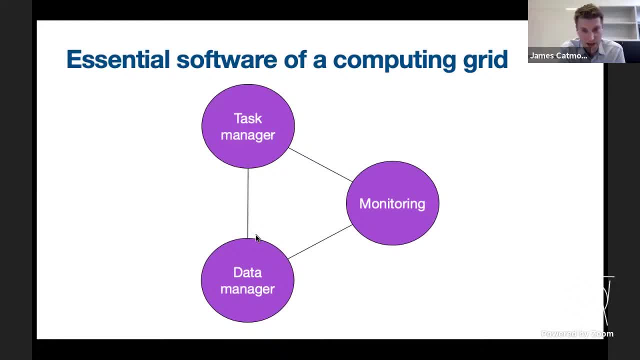 And then there's, finally, something called monitoring, which enables you to look at what's going on across the whole of the of the computing grid, And certainly in Atlas, but also in some of the other experiments. These are the three, the names of the three software components we use. 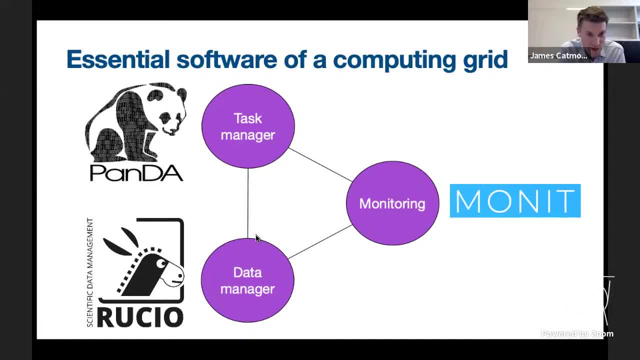 The task manager is called Panda, The data manager, which is now used quite widely, is something called Ruchio, And the monitoring is provided by CERN and it's called Monit. So these are the three pieces of software that we need to use to bind all these data centers together and turn them into a single computing grid that can do our work. 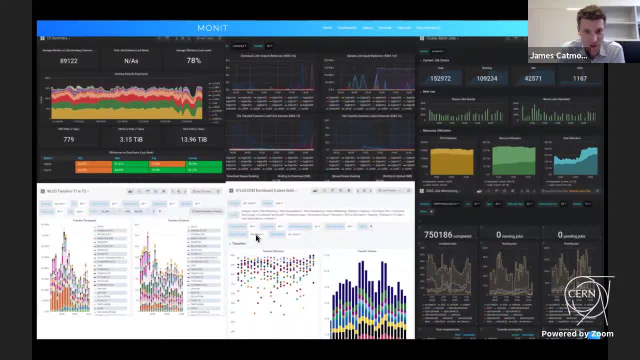 This is just a screenshot to show you what Monit can do. I'm not going to go through this in detail, but you can see all the different kinds of plots that we can use to monitor what's going on as our jobs are running. 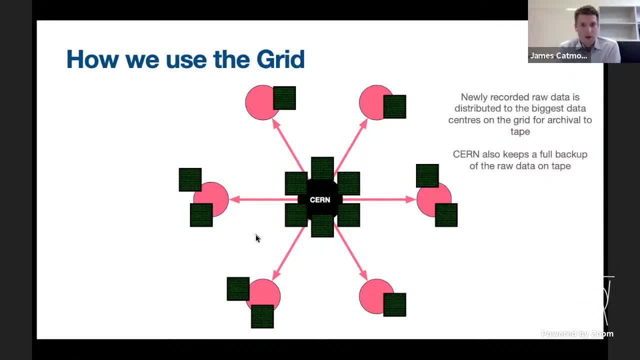 And as data is being used And as data is being transferred. So how do we use the grid? So, first of all, when we record data on Atlas, it has to be. This is raw data. It's extremely valuable. It cannot be replaced. 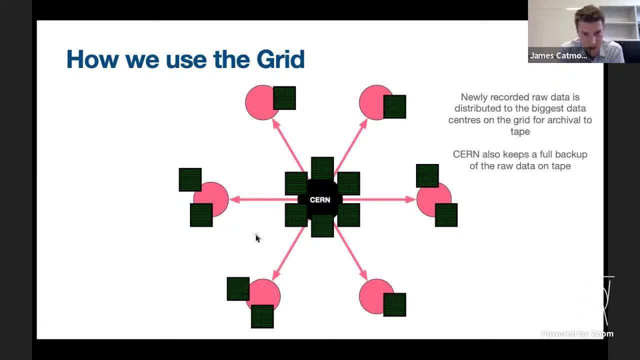 So we have to keep two copies of this. We keep one copy on tape at CERN and then we keep a second copy on one of these other data centers. So we spread the data out all over the world, so that if something bad happens in one of the data centers, it's all right. 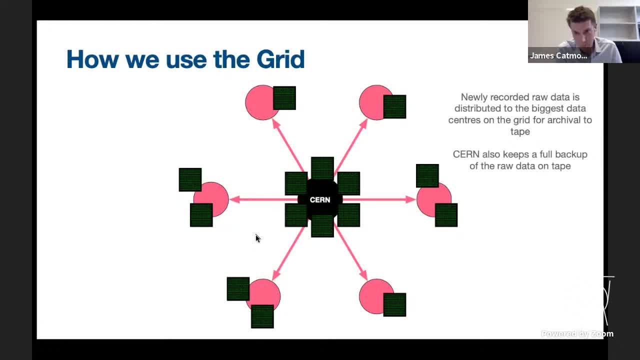 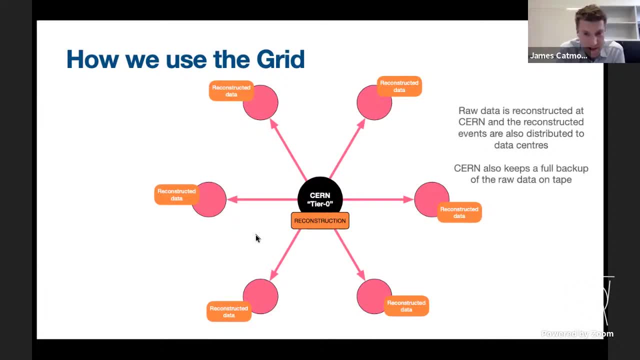 Because we've got a second copy That we can then distribute. So we spread the raw data around And then, in addition, freshly recorded data is reconstructed, turned into objects that we can understand, also at CERN. So the CERN has a very large data center, which we call a tier zero. 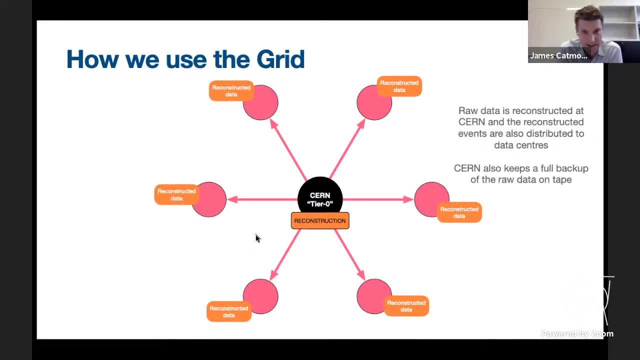 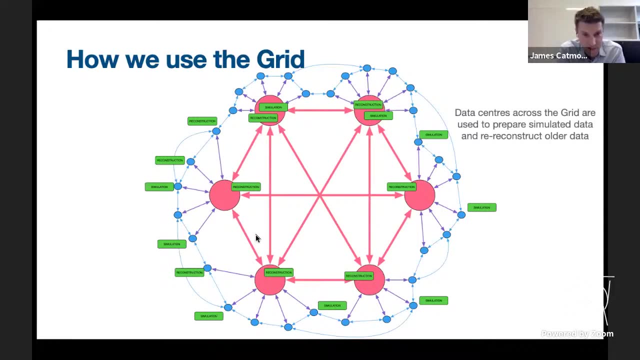 It does the initial reconstruction And then again we spread that data all across these data centers that are on the grid And then we have the reconstructed data sitting on the grid And then we have to do our simulation And we have to reconstruct our simulated events. 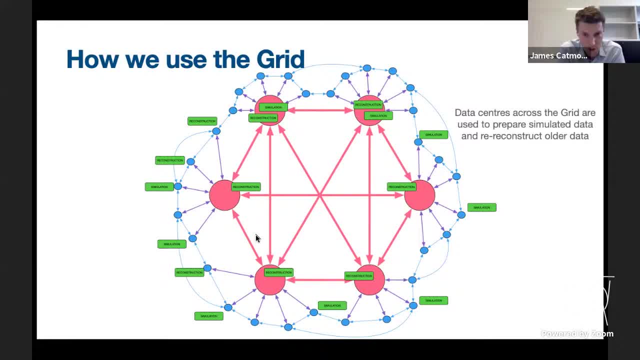 And we do this using the entire grid. So different grid sites are put to work doing different reconstruction and simulation tasks, And once these tasks are finished, this leaves us with data files and simulated files spread out all over these different data centers, And then these files are used. 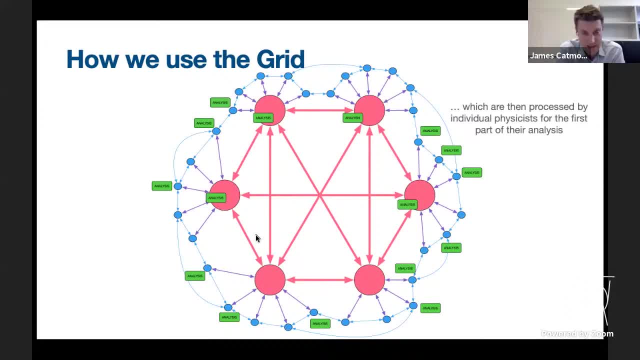 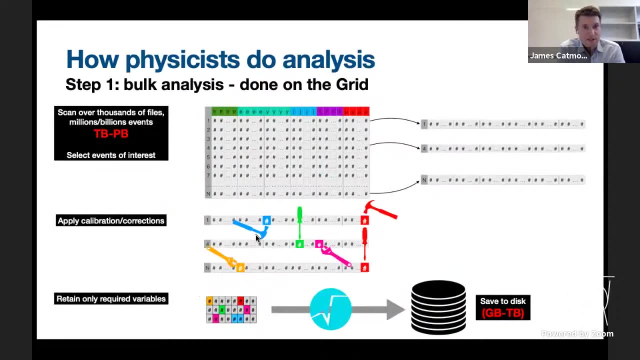 By individual physicists who are doing their physics analysis. So individual analysts are then using the different data centers to process their, to run their own, run their own analysis and to do their own research. So how is this actually done? What is an individual physicist doing when they look at the data that has been recorded and stored? 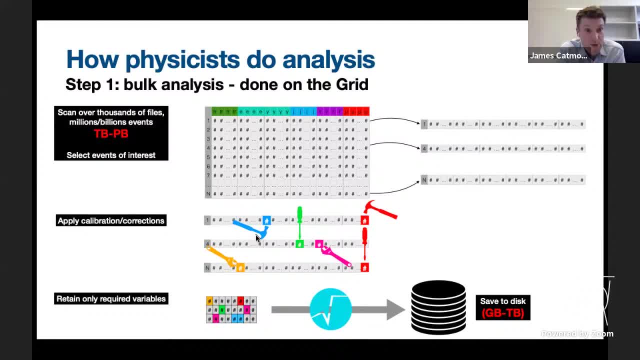 So it's done in two steps. The first step- we call this bulk analysis, And this is always done on the grid, And what happens is that the physicist- an individual physicist sitting in a university- writes a computer program that will scan over thousands of files, over millions or billions of events. 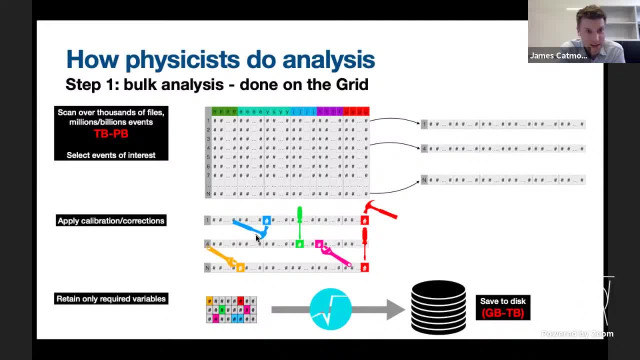 And that's terabytes or even petabytes of data- And the first thing that they do is they select the interesting events- By events, of course, I mean collisions or rows of the table- And only select the ones that are of relevance to the kind of physics studies that they are doing. 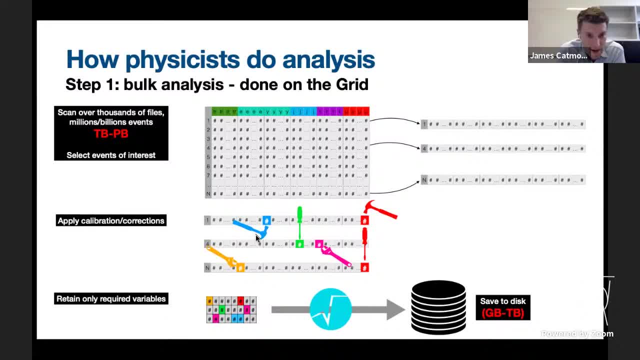 And then they apply, using their computer program, calibrations and corrections to the data, Because the data as it's reconstructed usually isn't perfectly calibrated. You have to apply various extra, you have to apply extra steps to somehow correct the data. 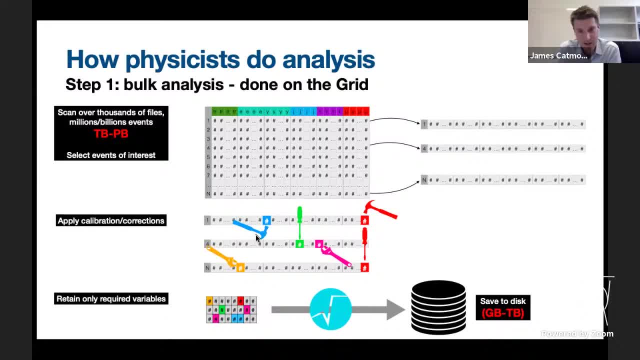 To apply our latest understanding of what the data looks like. So this is also done at this stage. And then, finally, the physicist decides which variables they need to actually run their analysis And they can throw away the rest, And then they write this into files. 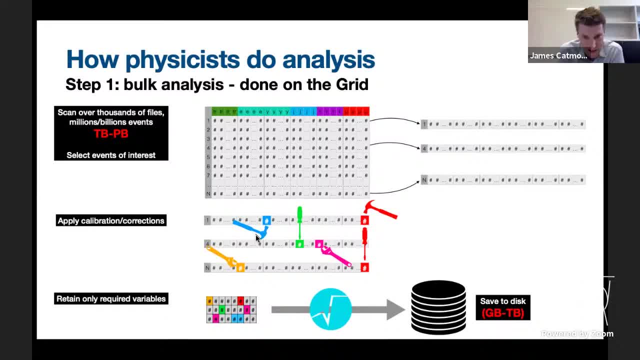 We call them root n-tuples. That's the name. Root is an analysis framework that's used across all of the CERN experiments, And then they save this back to disk for them to use And the difference between the files that they are saving. 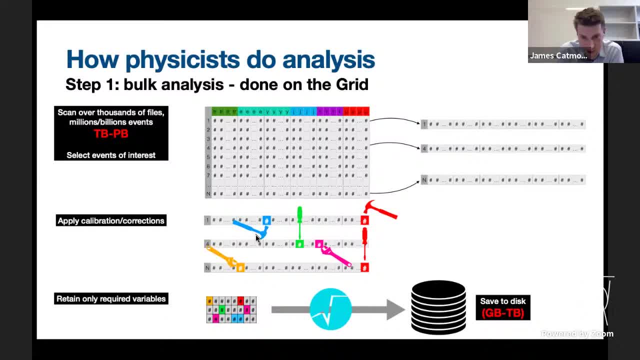 are sort of the same. The size is gigabytes to terabytes, Whereas the size of the files that they have been reading and running their program on are terabytes to petabytes. So we're talking, really, a factor of a thousand smaller, And these files are small enough for them to then analyze directly on their 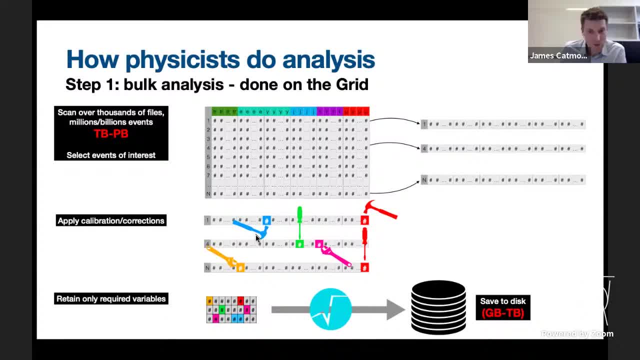 look at directly on their own laptop. So you have all of these data centers spread out, And so you might be asking how the poor physicist is supposed to know where the data is and which site they're supposed to use and how they log on to all these different data centers, and so on. 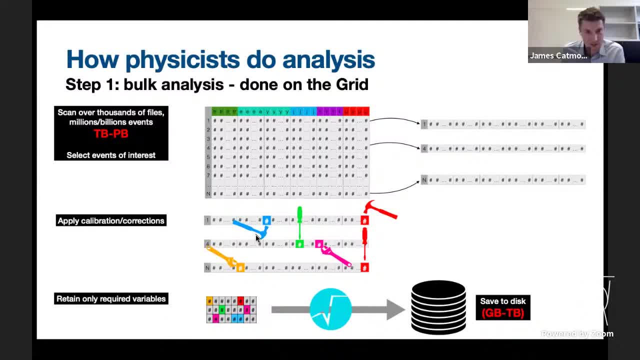 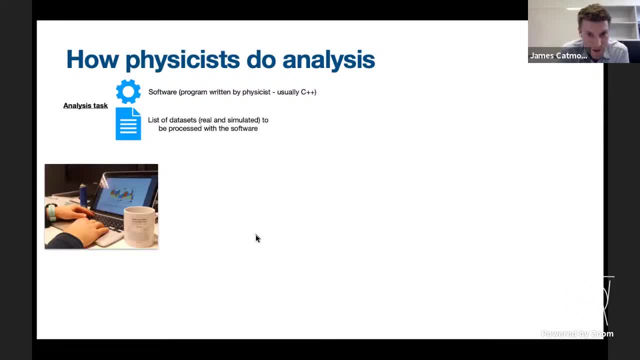 Well, the answer is they don't have to do this because the system does it for them automatically. So this is how it works: The physicist writes the program for doing the steps that I showed on the previous slide, And they also put together a list of the data sets that they need to process. 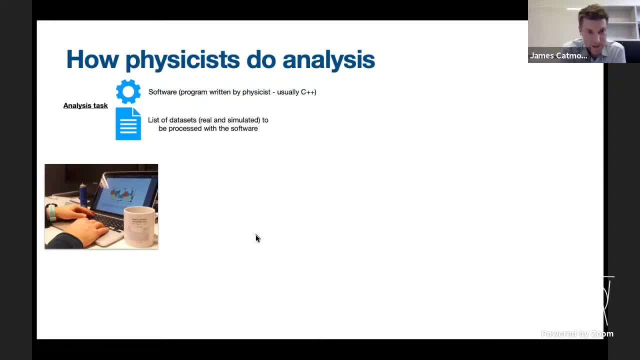 This is real data and the simulated data that they need to process in order to do their analysis, And then, using some software, they send this to this task manager, this thing called Panda, And they don't, so they don't have to decide where it goes. 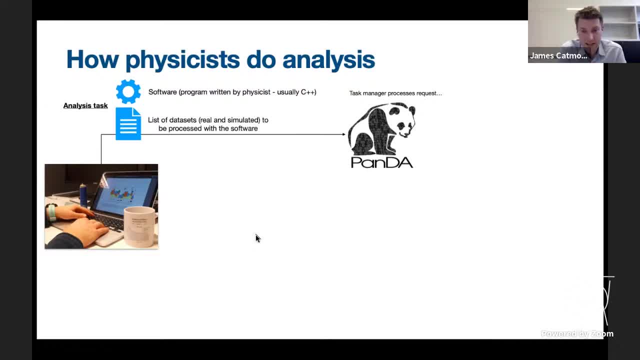 They just send it to a server which is actually at CERN And it decides: where this, what should be done with this task. So the first thing that this task manager does is it asks the data manager: where are these files, Where are these data sets that this user wants to access? 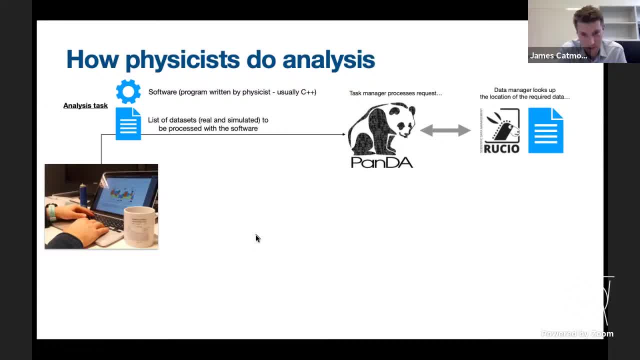 Whereabouts are they, And the data manager will tell the task manager automatically where these data sets are, And this then enables the task manager to decide which data sets they want to access, Which data centers to use. So the first thing that happens at these data centers 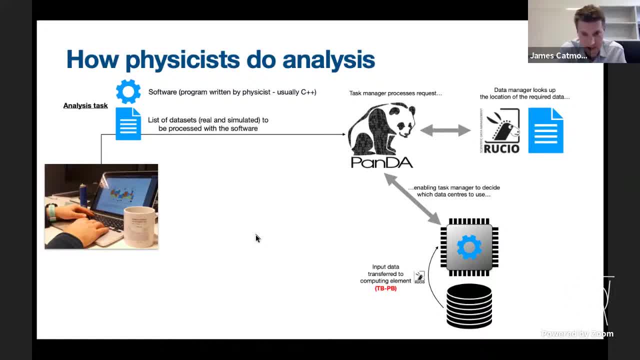 once the work has been dispatched to them by this task manager, is the input data which is needed is transferred from the disks of the site of the data center to the computing elements And the computing elements. the processors then work on that program that the physicist has written. 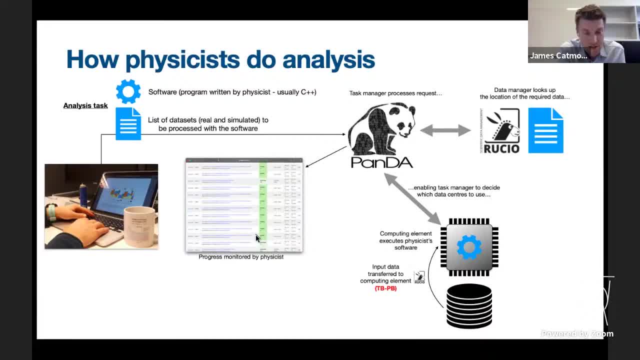 and start to run through all the files. The physicist can monitor the program. They can see the progress Again using Panda. they can just go on a web page and they can see the progress that their jobs are making as the data centers chew through their analysis. 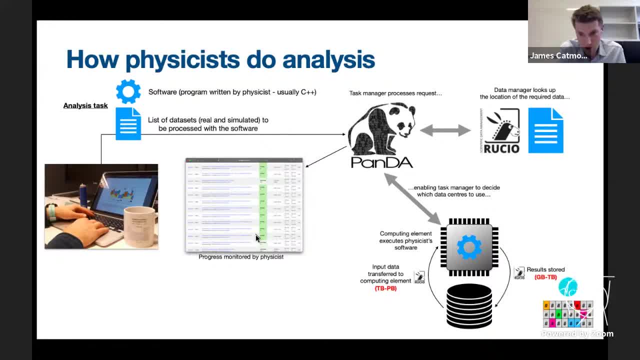 And then, once the jobs are finished, the results- which are now a lot smaller, as I showed earlier- are transferred back onto the disks of the site where the jobs ran, And then, finally, the physicist, if they want, can download these results directly to their laptop. 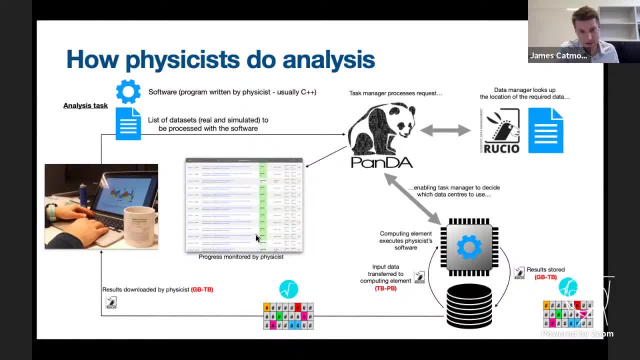 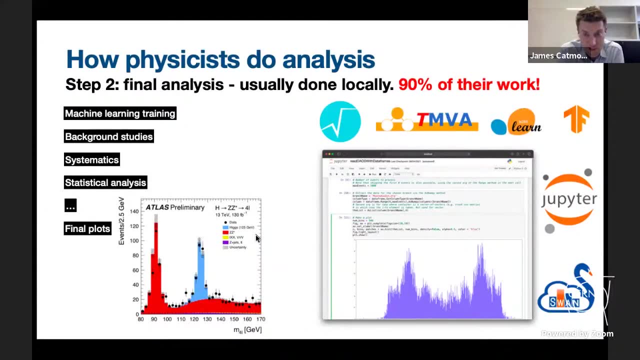 or to their university cluster, and can then do their analysis using local resources. And this local analysis is the second step, We call it final analysis, And this is, as I said, usually done on their local computers or even their laptop, if they've been very efficient. 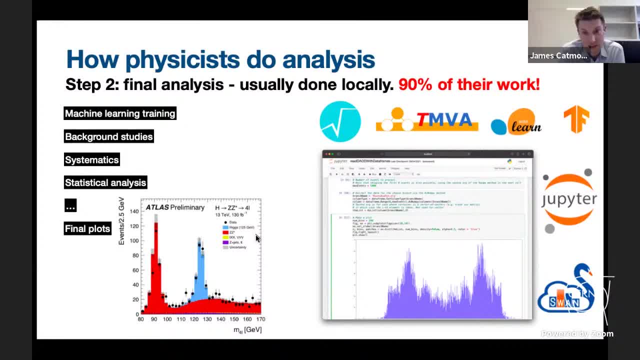 in reducing the size of their data sets, And I should stress that 90% or more of the work of an average physicist is spent at this step, The step that I described earlier. it's the step that's sort of interesting from the point of view of understanding how the grid works. 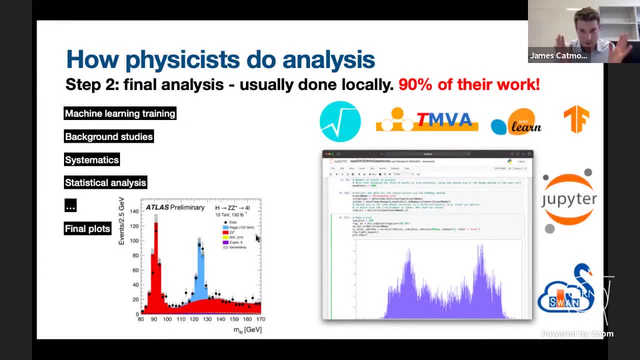 But from the point of view of how a physicist works, most of their job is spent after this is done and once they've got these small files on their laptops And they're doing the kind of work involving things like machine learning training, They're studying the backgrounds to the processes. 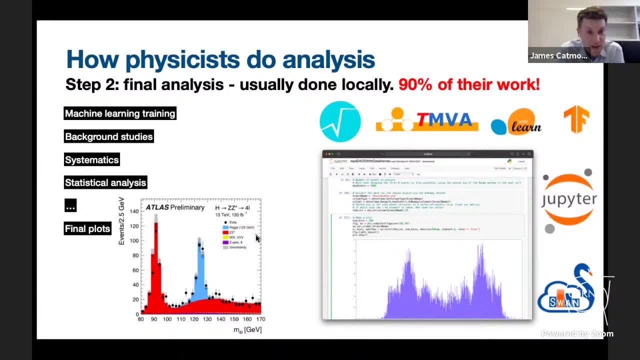 that they're interested in. They're looking at the uncertainties of their data, systematic uncertainties. They're doing statistical analysis, Many, many other tasks- And, finally, they're making their plots, which are what go into the publications, And this is done using a very large number of tools. 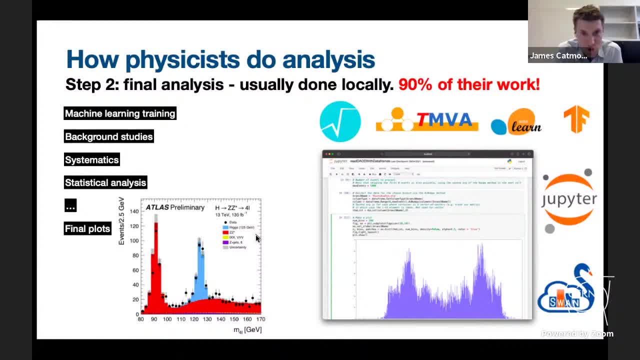 The linchpin of all of this is this root data analysis framework, which is provided by CERN and is used across the experiments, But we also use many other different software packages for machine learning and statistical analysis. We use things like TMVA, Scikit-learn, TensorFlow. 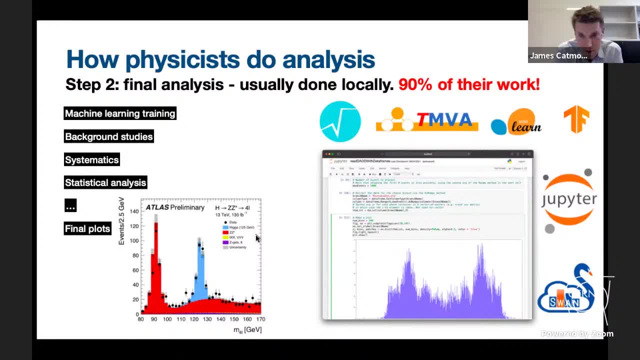 And we also use other software packages for machine learning and statistical analysis. And recently there's been a trend towards using Python for doing the final step of this, physics analysis. And most recently, physicists have begun to use more and more these mighty Jupyter notebooks. 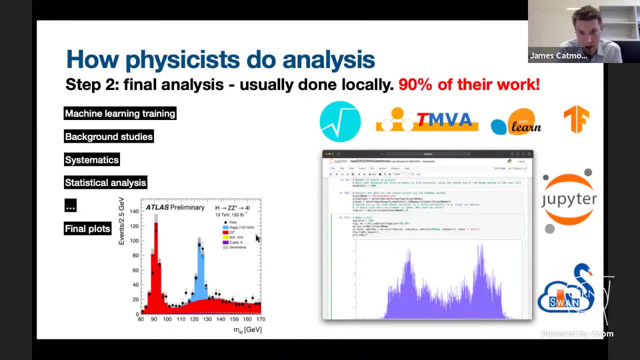 where you can directly use a web interface to do your analysis in a very user-friendly and interactive way. I've shown a little screenshot of this And actually CERN provides a facility for doing this using their data center, which is called SWAN. 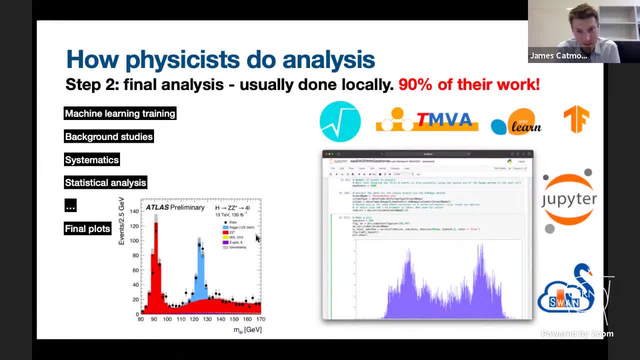 So there are many different ways for physicists to work. There are almost as many ways for physicists to work as there are physicists, But we have this huge range of tools, some of them from within the particle physics community and some of them from outside it. 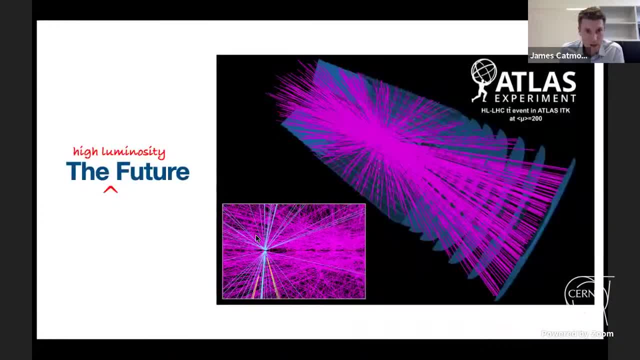 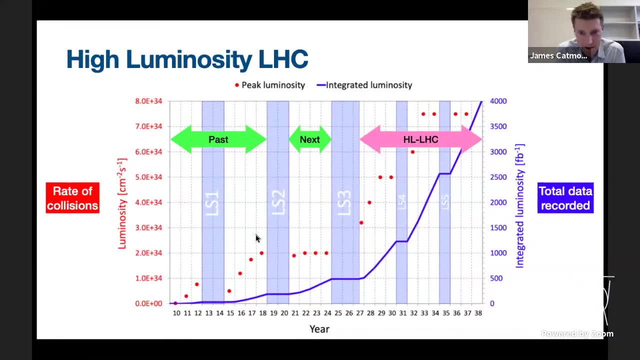 that we are using to do our analysis. So now, in the last, let's say, five minutes or so, I want to talk a bit about the future. I call it the high luminosity future because in the late 2020s. 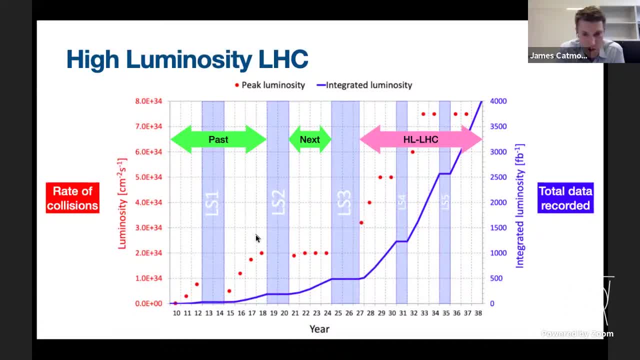 the LHC is going to get a serious upgrade. So this plot here. there's quite a lot of information to digest, But on the red dots they more or less show the rate that collisions have occurred. at how many collisions per second? you can almost envisage this is. 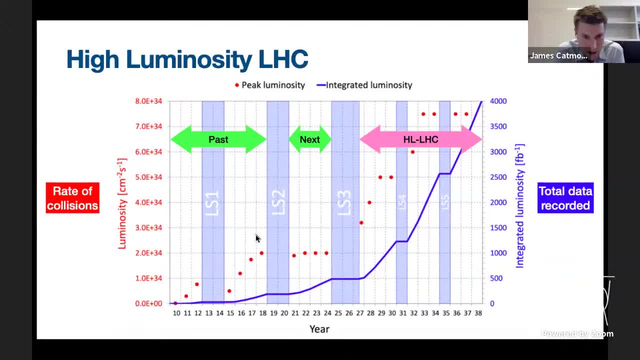 And you can see that this has grown steadily over the years. The blue bands which are labeled LS1, LS stands for long shutdown. These are periods of time when the machine has been switched off for maintenance and upgrade. The blue line is showing the total volume of data that's been recorded. 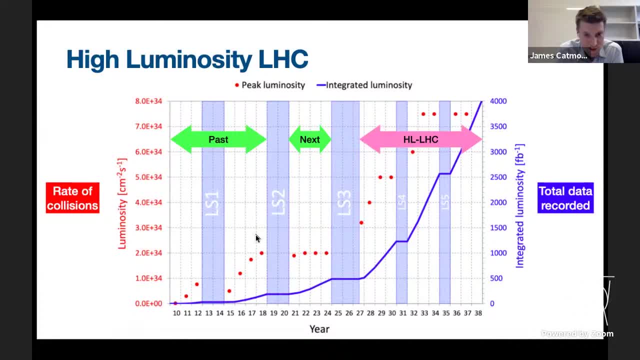 So you can see that the amount of data has grown steadily over the years. We're going to start in 2022.. The next run is called run three And we're going to be recording data roughly at the end of the year. This is the same rate that we were recording it. 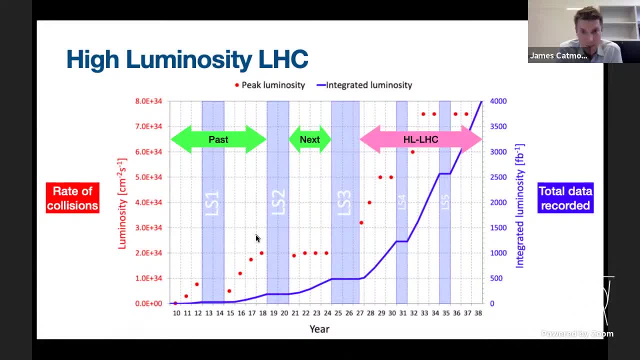 towards the end of the previous run in 2018.. But then, during this long shutdown three, which will occur in the mid 2020s, the Large Hadron Collider is going to be seriously upgraded and it's going to turn into the high luminosity LHC. 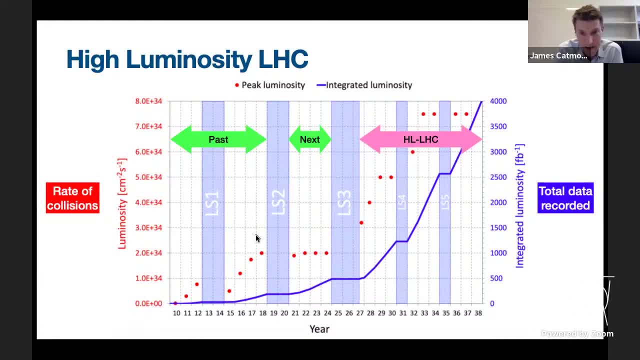 And you can see that, after this period, these red dots shoot up, meaning that the rate at which the collisions will take place is much higher. And you can see that the slope at which the data is being recorded also shoots up, Meaning that we're going to be recording. 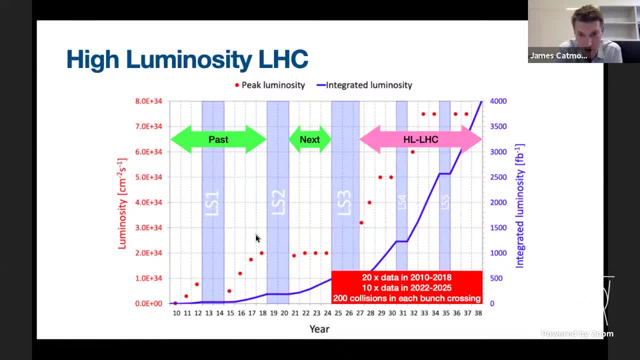 well, something like 20 times more data than we recorded during the whole of 2010 to 2018, or 10 times more data than we will record in 2022 to 2025. And whereas we have something, you know, like 30 to 60 collisions per bunch crossing now. 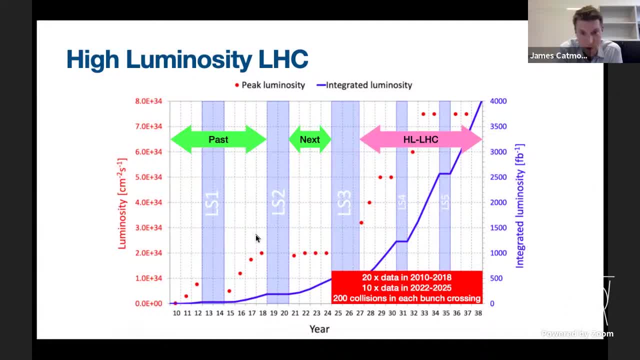 when we have the high luminosity Large Hadron Collider. there will be more than 200 of these collisions in each of the crossings of the bunches, So we're talking about massively more data to process. To go alongside that, we need massively more simulated data. 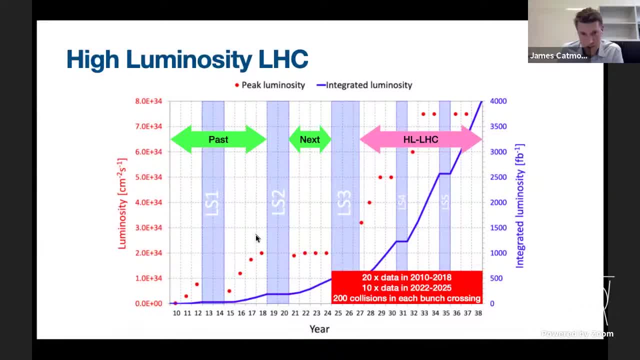 And this is a huge load on the computing And we're going to have to do things very differently in order to be able to cope with this amount of data. So how are we going to meet these challenges? So the first and perhaps most obvious thing: 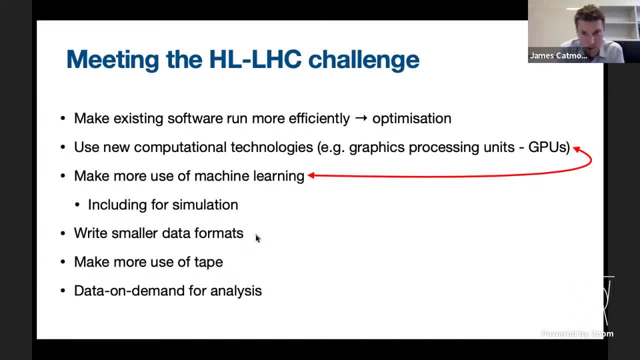 is to make the existing software run more efficiently. This is what we call optimization, And we're working on this all the time. We also want to be able to use new computational technologies, And in particular, I'm talking here about graphics processing units, or GPUs. 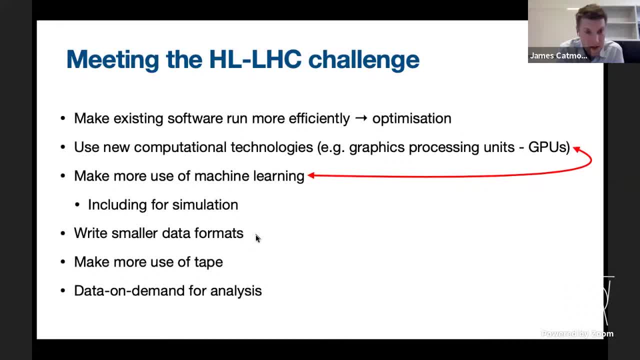 I'm going to say a bit more about that in the next slide And related to this, we could also make more use of machine learning, including for doing the simulation, but for doing a number of, for doing many other tasks as well. 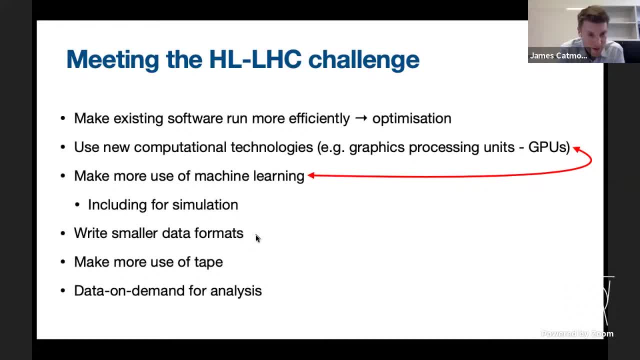 We could also write smaller data formats, So try to write slightly less data And so or we could make more use of tape. I said earlier on that tape is cheaper. That is the cheapest form of storage, And if we can make more use of this, 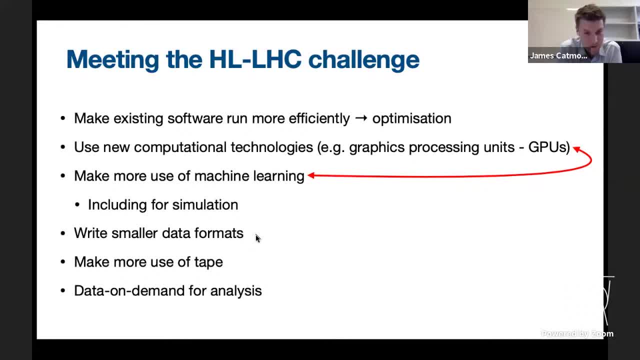 then this will enable us to store more data for the same amount of investment. And then there are ideas to do more on-demand data analysis. So you don't have to go through all the steps that I showed you earlier on that the physicist needs to go through. 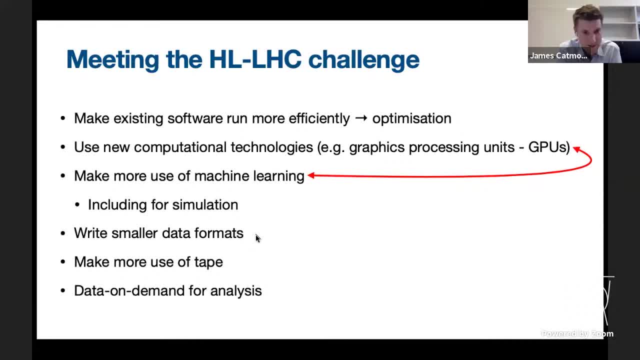 to run their analysis jobs, that you would be able to get the data in an on-demand way, Probably using these much smaller data formats. Now, this is a topic in itself and I don't have time to go into the details of all of this. 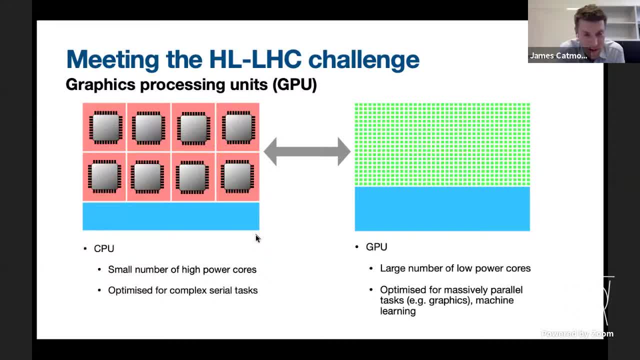 but I do want to say something about graphics processing units, because this is what we call a hot topic at the moment. So the things I've been discussing earlier on, they're what we call CPUs- central processing units- And these have a small number of very high power computer cores. 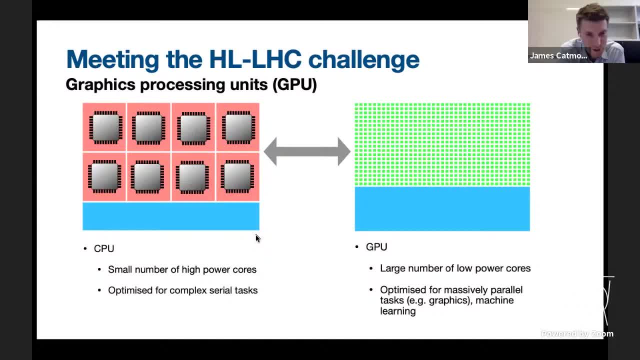 So, typically, you have maybe something like eight of these cores, like I was discussing earlier, And these are optimized for very complex but largely serial tasks. And you can, as I described earlier, you can allow these processes to share the work using either multiprocessing or multithreading. 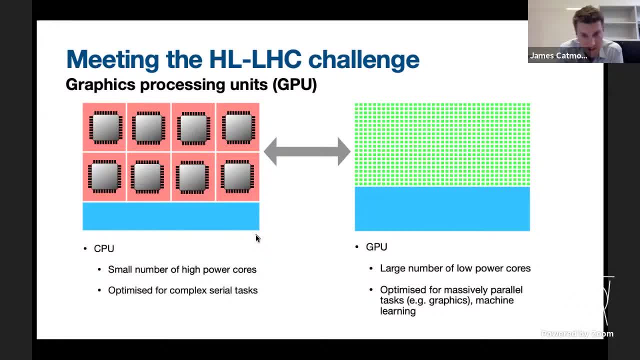 Now a GPU uses exactly the same technology. It's still the same kind of silicon and the same kind of logic gates, but they're designed slightly differently. There are far more of these cores, potentially thousands of them, or even tens of thousands of them. 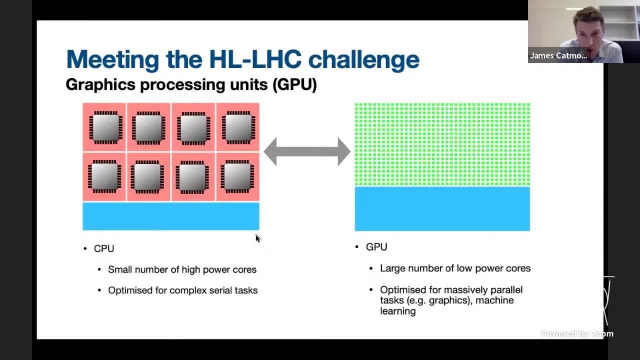 rather than just say four or eight or 16, but they are much lower power, So there's less problem with the heating and they're drawing less electricity. They're lower powered, They are slower, but because there are so many of them, 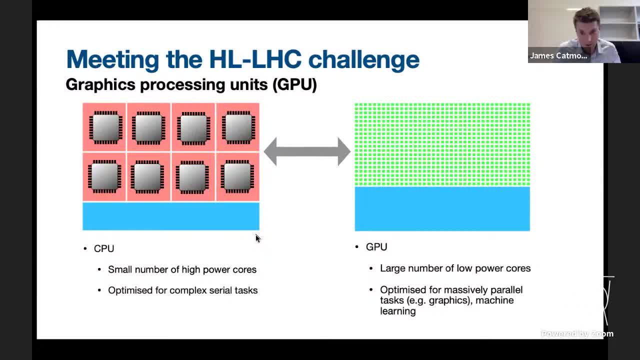 if you can write software that can be massively paralleled, run massively in parallel, you can really get very, very significant speed ups. These were originally designed for doing graphics processing, particularly for things like gaming where you need very high speed graphics. 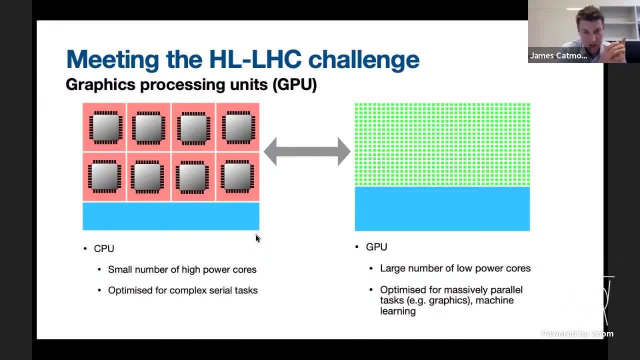 And more recently they've been used for doing machine learning, And we're very interested in Atlas, but also in the other LHC experiments, about using these for doing more of our data processing. So there are two ways we could think of doing this. 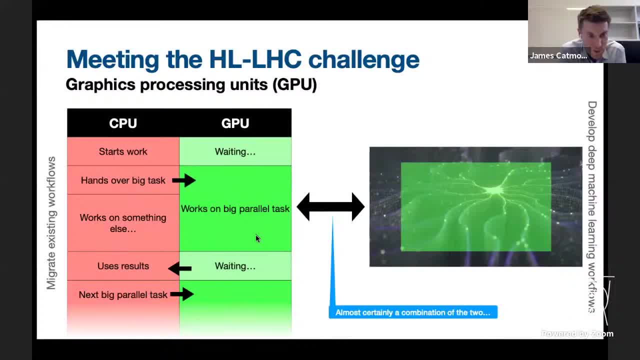 The first is to try to exist to migrate our existing workflows so that the CPU and the GPU would kind of work hand in hand. So the CPU which would start work it would come across some big parallel task that it would be quite slow at doing. 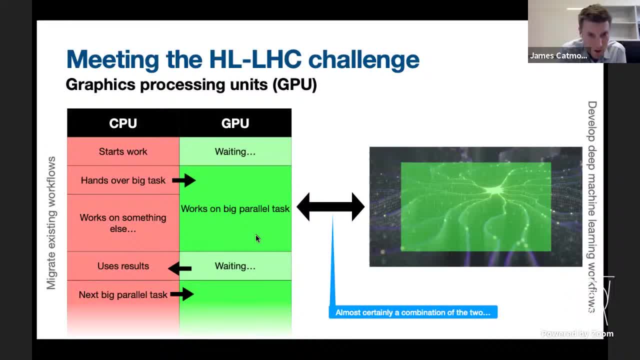 and it would hand that over to the GPU, which will work on this big parallel task. And whilst it's working on this big parallel task, the CPU can just work on something else in the software And once the GPU is finished, the CPU can use the results that it has produced. 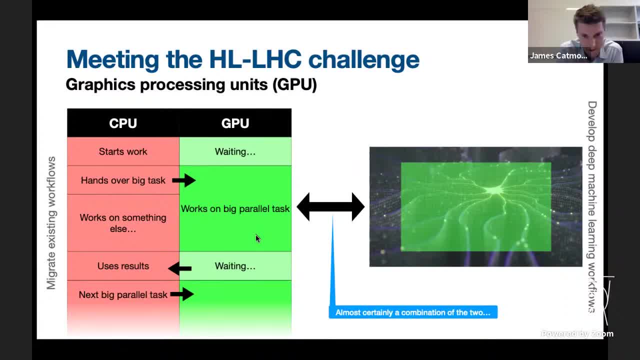 and then it can pass on to the next big parallel task. The alternative to this is to develop workflows which can largely be run using machine learning or artificial intelligence And, as I implied a few minutes ago, artificial intelligence. machine learning applications run very well on these graphics processing units. 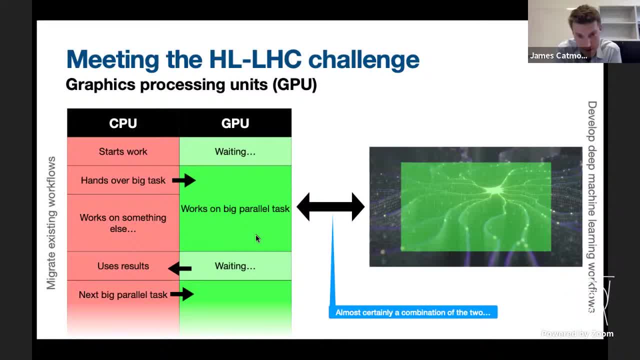 these GPUs because they are inherently parallelizable in this way. Now, it's almost certainly the case that we will end up doing a combination of two, both of these things. So some of our software will be using the existing workflows but somehow migrated so that CPU and GPU 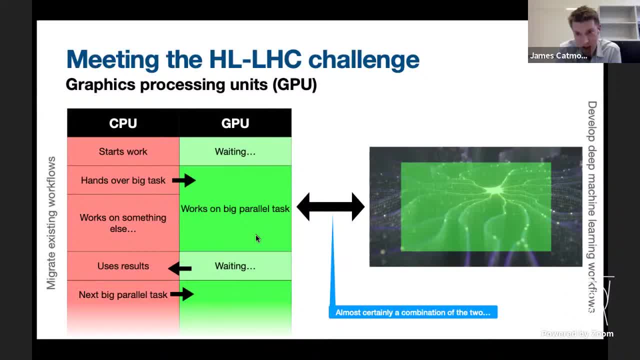 can work on it together, And then some of our workflows will be developed using machine learning workflows, And this is going to be the work for us now for the next several years, until the high luminosity LHC starts up in the late 2020s. 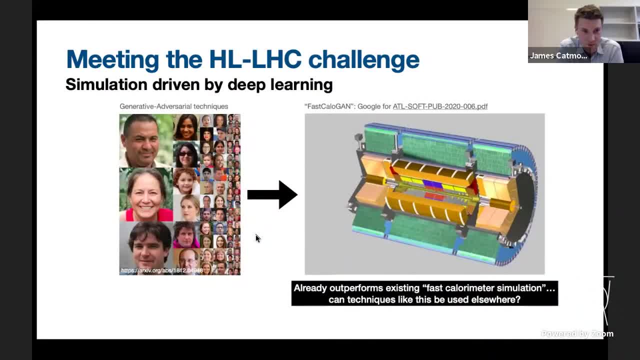 And on simulation, this is really the last topic I have to talk about. There's the possibility- in fact we already do this to some extent- of using deep learning to do our simulation. So you may have seen in the media something called deep fakes. 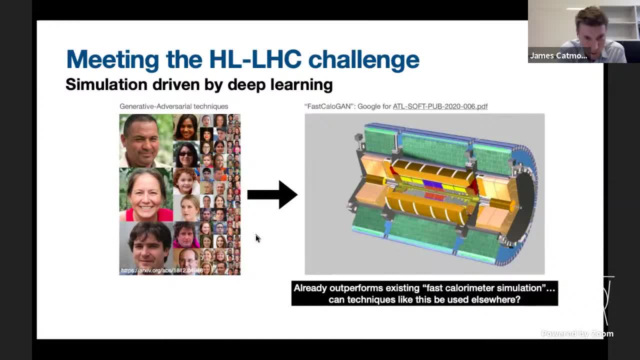 All of these images of the people here. they're not real people. They've all been generated by a neural network, by an artificial intelligence, which, and the technique we use for doing this, is called generative, adversarial. Now, I don't know about you. 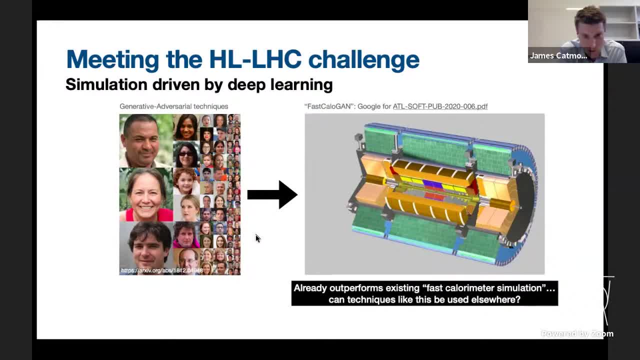 but I find these things quite creepy. But fortunately the particle physics community has come up with a much more wholesome use for these techniques, And that's for doing simulation. So we have applied these generative adversarial networks to this very time-consuming calorimeter simulation. 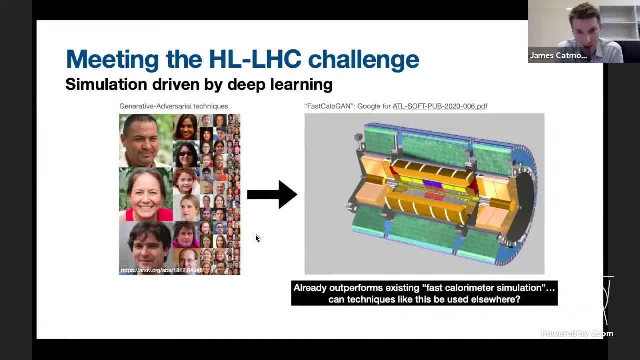 that I talked about earlier And we've developed. ATLAS has developed something called FastColorGAN. If you can Google for this document, you can even read about it And already- even now, in 2021, this technique outperforms. 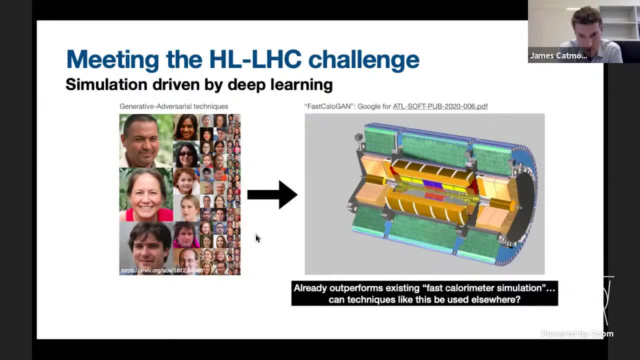 the existing fast calorimeter simulation that we've already written. So the question is: can techniques like this be used elsewhere in the simulation, or elsewhere in the reconstruction or even in the event generation where we simulate the collisions? And this is going to be a big question. 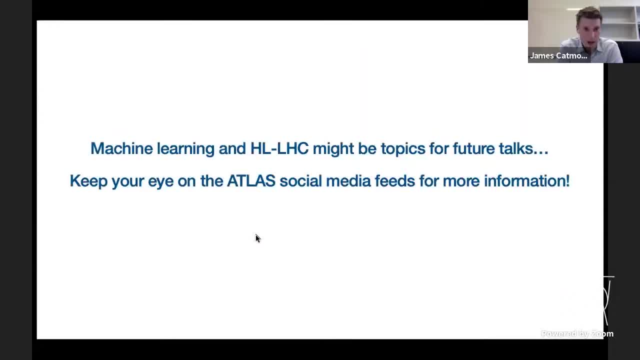 for the next run. I should point out that machine learning and the high luminosity LHC might actually be topics for future talks in this series, So please keep your eye on the ATLAS social media feeds for more information Now. I'm almost at the end now. 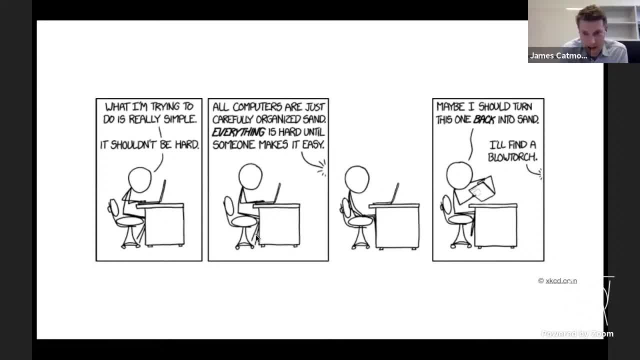 but we're going to have, hopefully, some discussion Now in particle physics, as I think in every walk of life we kind of have a love-hate relationship with computers. You have this person here saying what they're trying to do is really simple. 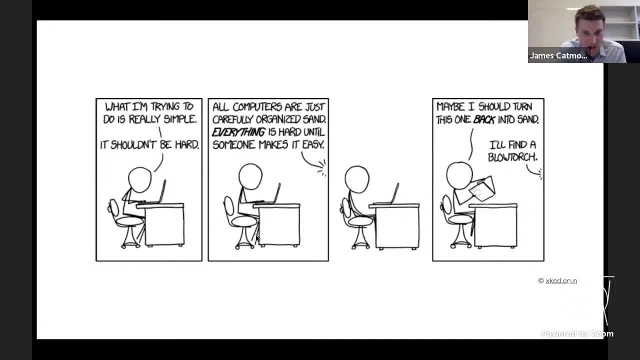 It shouldn't be hard. And their friend is telling them that really computers are just very well organized: sand, the silicon and everything is hard until somebody else makes it easy. And this person's obviously getting frustrated and they say, well, maybe I should just turn this one back into sand. 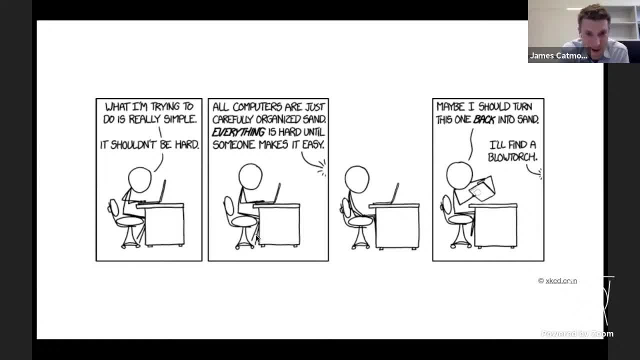 And their friend says: well, I'll find you a blowtorch. So this is kind of a humorous way of saying that, although sometimes computers and software can be incredibly frustrating things, we definitely can't work without them And actually developing software for the next generation of colliders, for the LHC. 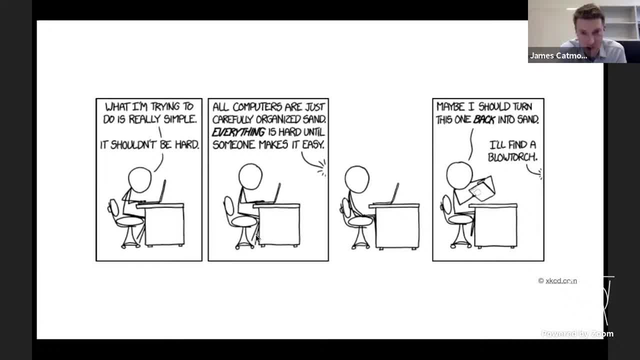 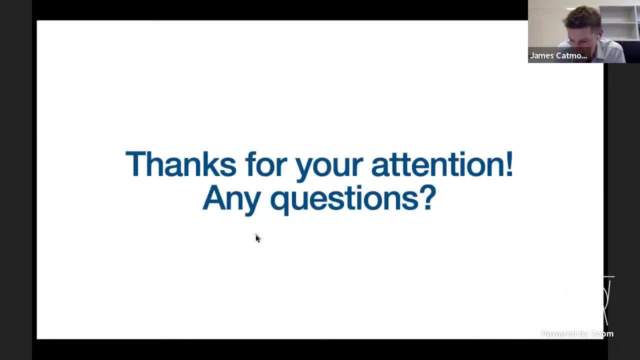 is an incredible intellectual challenge in itself, alongside physics. So with that, I'm going to thank you for your attention And at this stage I think we can have some questions. So thank you very much for your attention. Thank you very much, James. 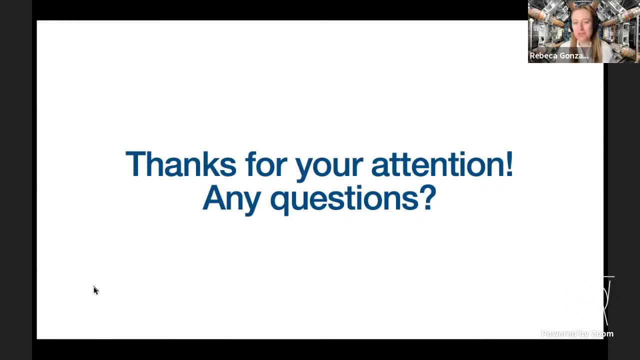 It's a pity that this is not a public talk with audience, so we could all clap. So this was a fantastic talk. I think I enjoyed it very much, And the flying pig story was just brilliant. So then I guess you are ready for the Q&A right. 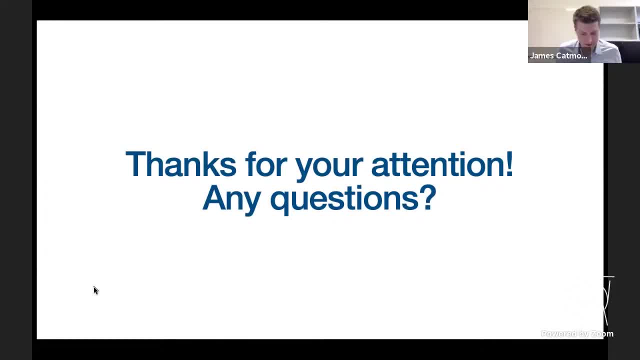 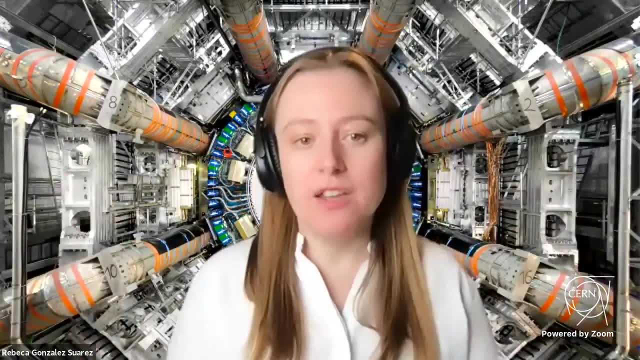 Yes, All right. So I'm going to ask you to stop sharing your slides so people can see you a little bit bigger. Excellent, So then I think we can just get into them. So we are starting asking. I mean, we're starting with questions from Instagram. 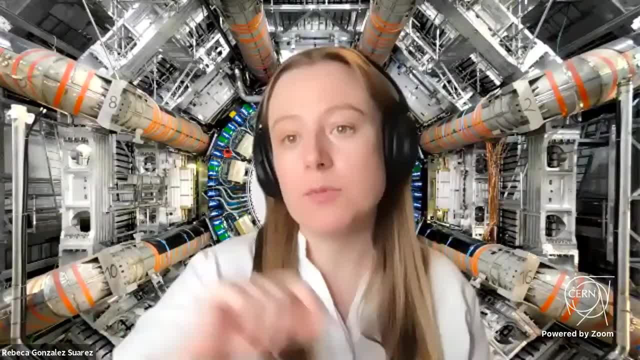 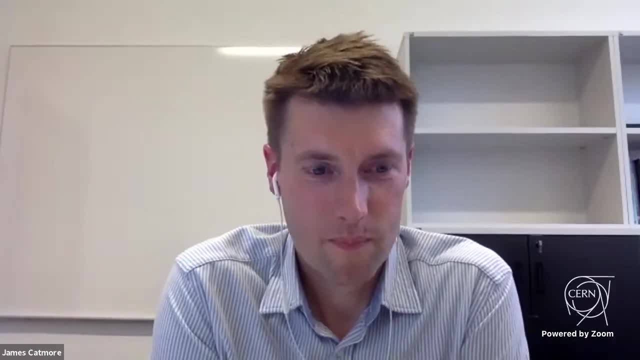 So this is going to be the first one. This is now the time for you to type your questions here in the chat in YouTube and sending us some more, And also, of course, keep asking in Instagram as well. So all right, So let's see. 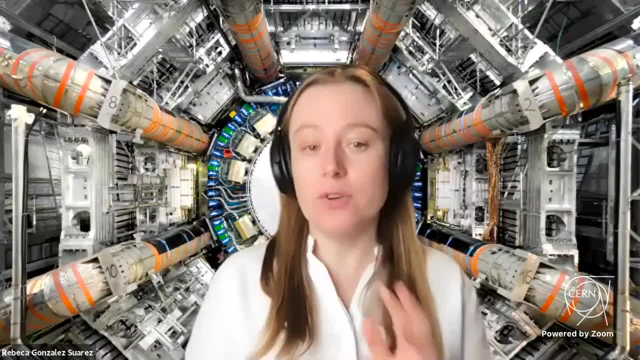 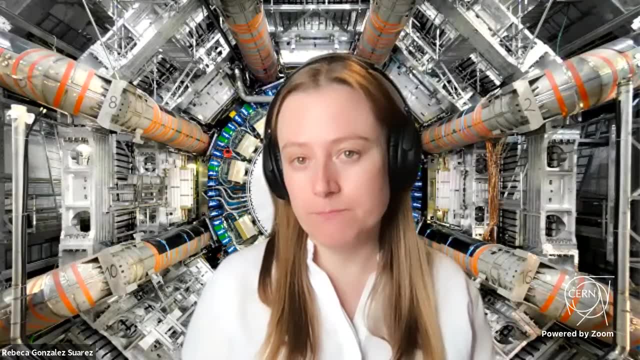 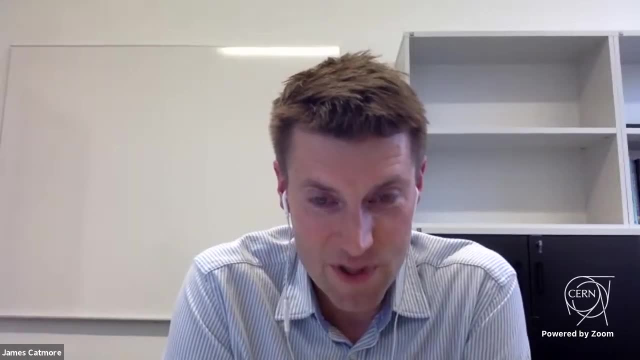 The first question that we have for you today is the following: So since when have you used machine learning techniques, particularly in the trigger system? Well, yup, So, in fact, machine learning is nothing new in particle physics. It was even being used. 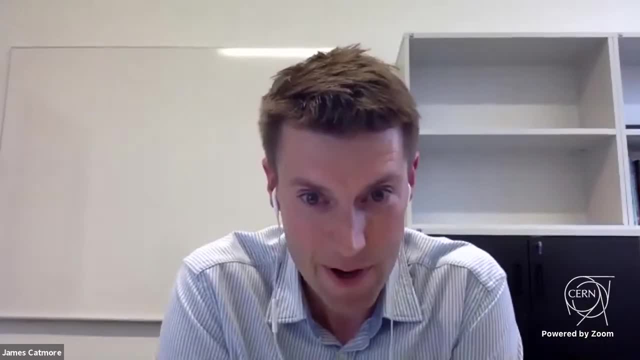 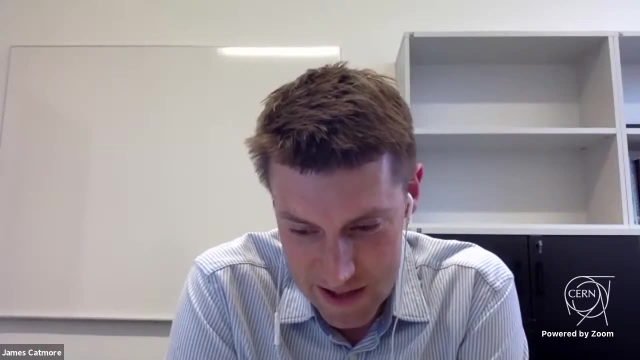 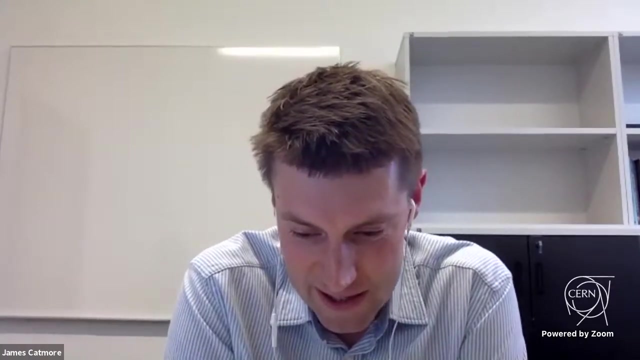 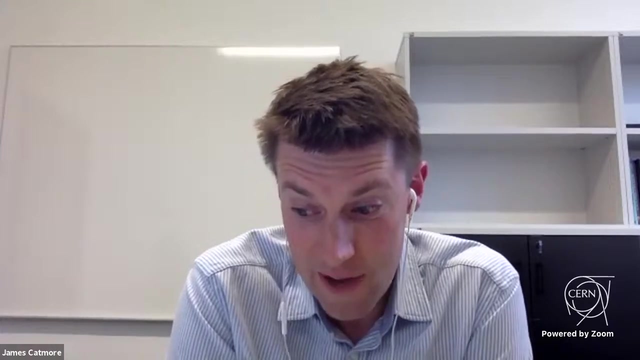 in the predecessor to the LHC in LEP when I was still at school, And very simple neural networks and then slightly more complicated systems called well, slightly different machine learning techniques, called boosted decision trees, were being used in those experiments. They were instrumental in discovering something called the top quark. 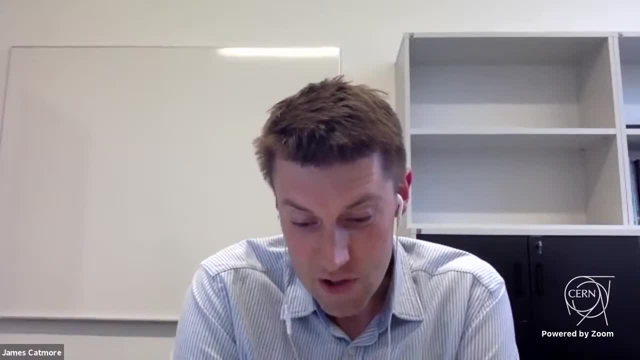 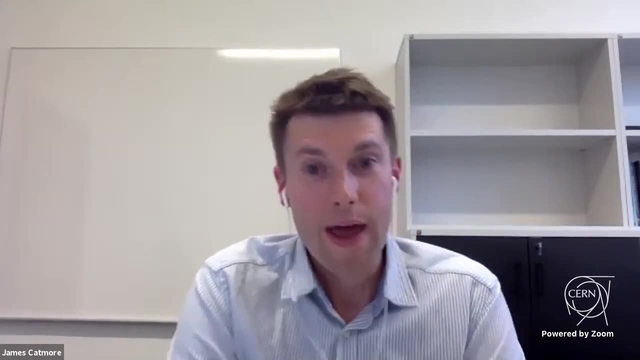 in the early 2000s, So machine learning really isn't anything new. but what has changed in the last few years is that as computers have got more and more powerful, and also as the tools have been written outside of our field, it's become easier and easier to do something called deep learning. 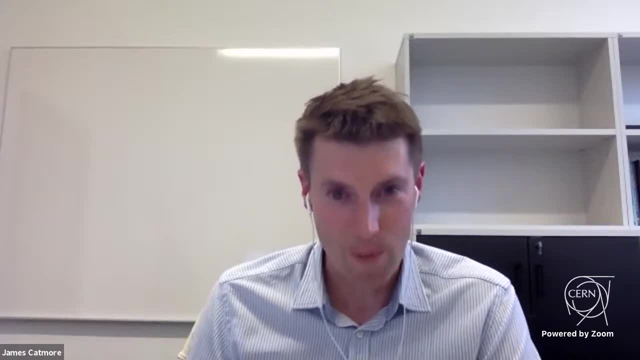 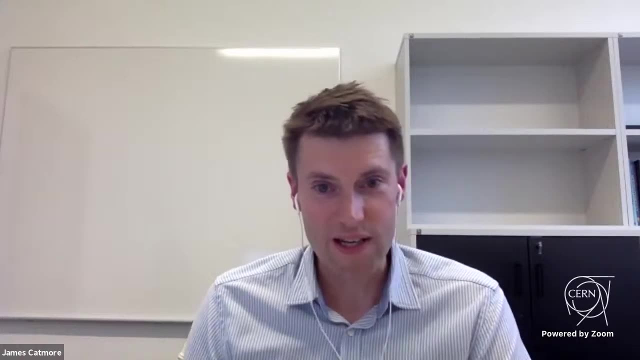 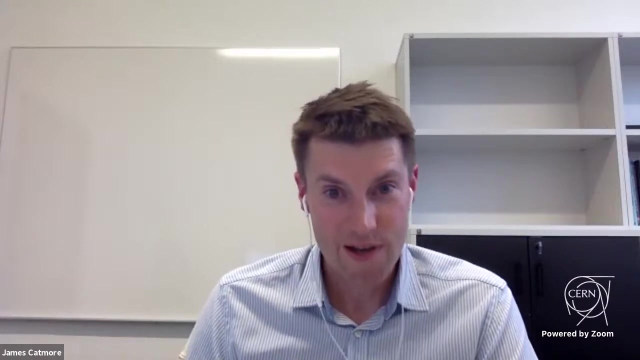 where you have these extremely complicated neural networks that have enabled us to do more and more powerful analysis using machine learning? So I think the answer to the question is that machine learning in particle physics predates Atlas. It was used in the Tevatron in the 90s and 2000s. 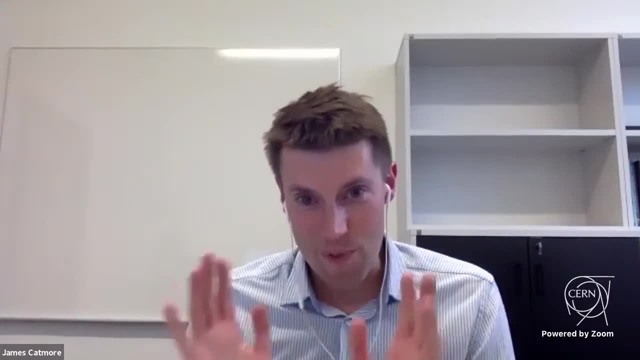 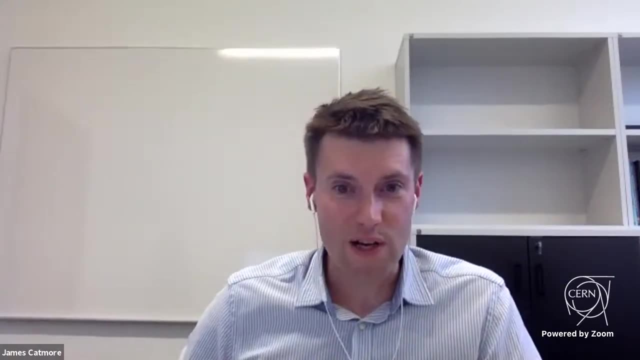 and even before that. It's just that in the more recent years it's become a lot more powerful And in fact we already use machine learning even in the reconstruction. We use it in the early stage of the tracking to do something called pixel clustering. 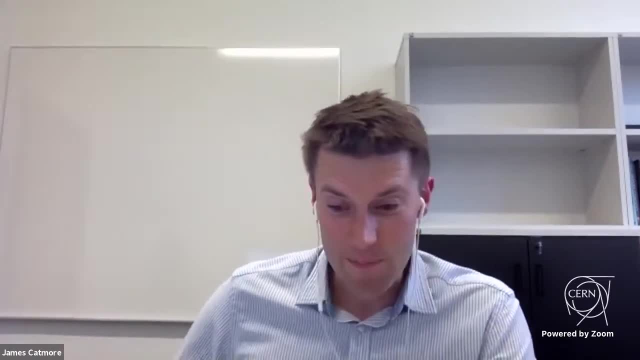 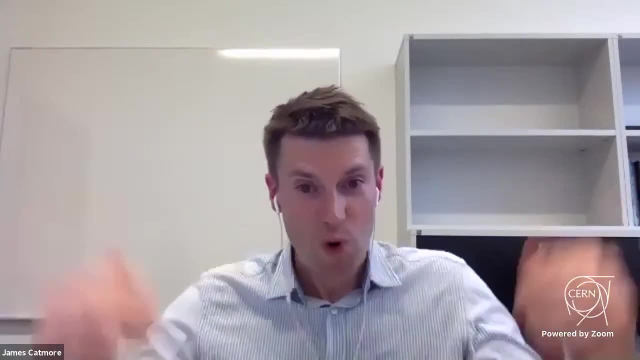 And we also use it in something called well flavor tagging. So yeah, it's really had a long history. It's just that recently it's become so much more powerful because of computers and because of the developments in industry and so on. 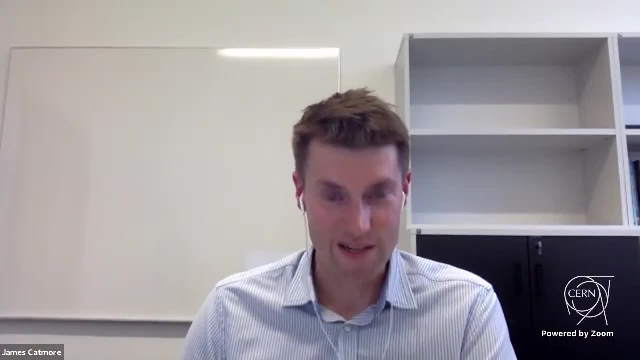 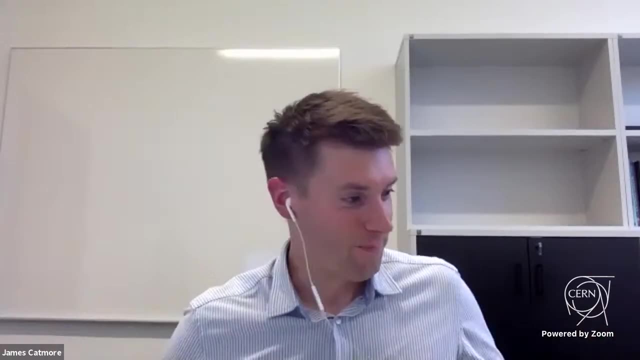 that we've been able to sort of jump on this and use it more intensively And, as I say in the HLNHC, in the future we expect to be using it even more than we are now. I hope that answered the question. 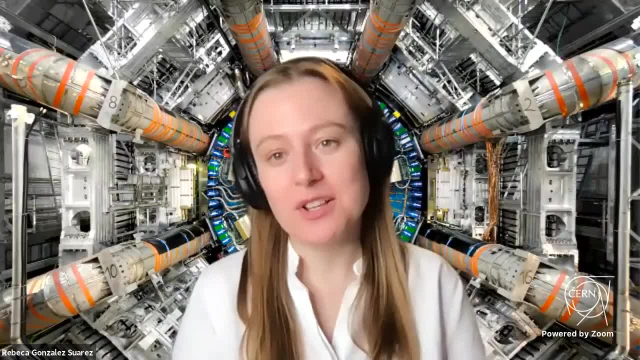 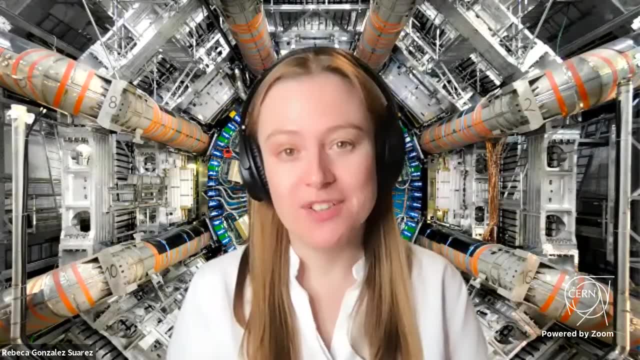 I think it did. However, I have to tell you that there are a lot of questions relating to this topic. So then there is like a quite straightforward follow up, That is, how much do they improve physics analysis, this machine learning techniques? Well, let's say, normally we're not talking about. 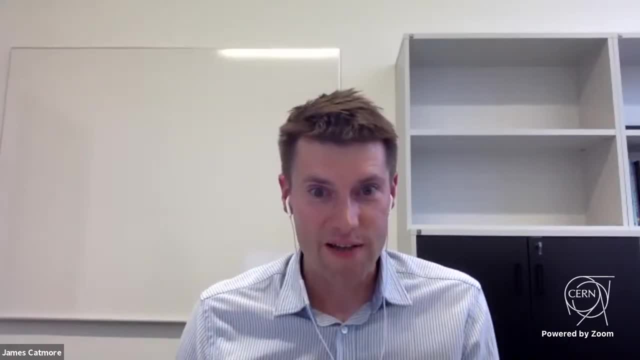 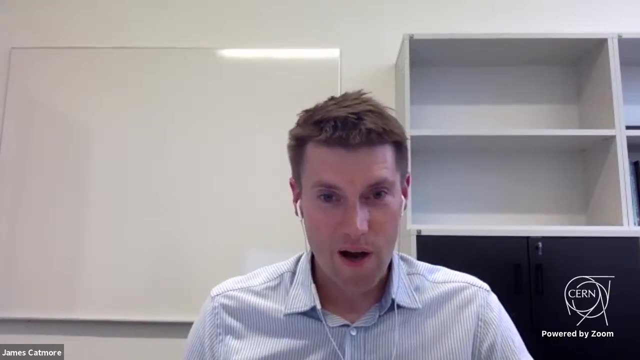 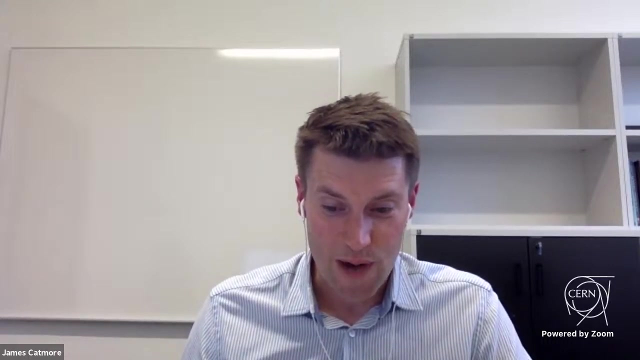 well, okay, let's put it one way: There are some physics analyses that it would be very difficult to do at all without it, Just because the background processes are so big in comparison with the signal. So, for example, I think it would be very difficult to do something. 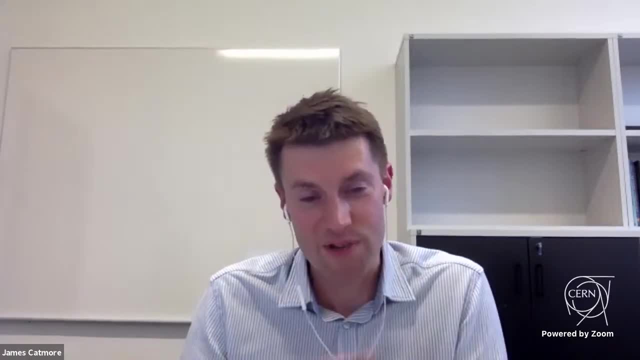 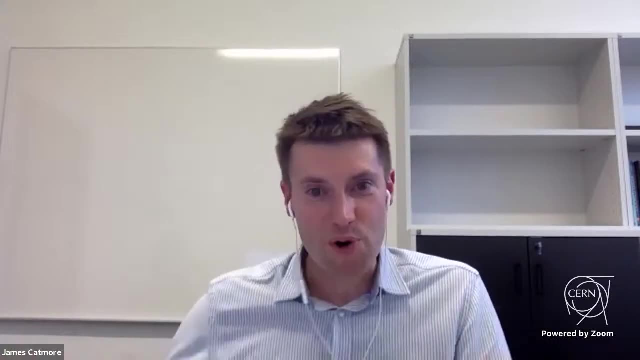 like Higgs boson decaying into two W bosons without using some kind of machine learning. It's not necessarily these very deep neural networks. It may just be some kind of thing like a boosted decision tree which we've been using for years. 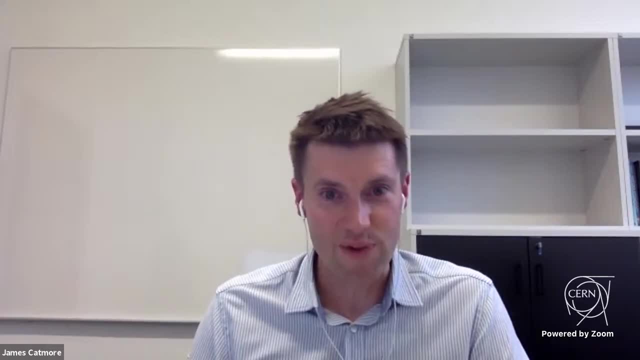 But without some kind of machine learning, it would be extremely difficult to do this. Now, when it comes to deep learning, we're only at the beginning. We're usually talking about improvements of something in the order of percents over what we have already. 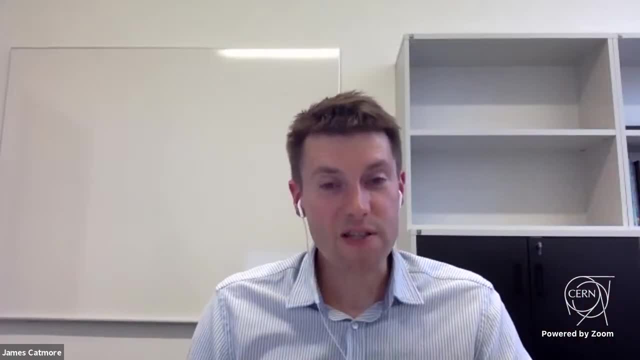 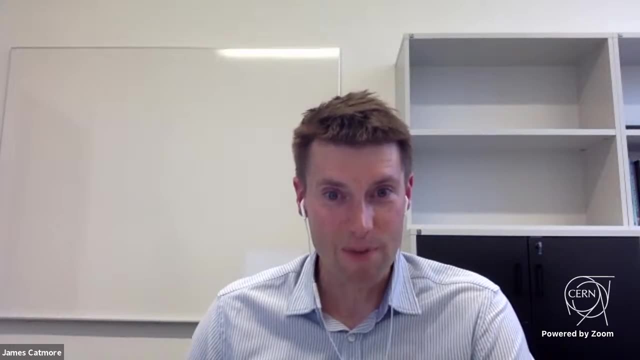 from simpler machine learning techniques. But these deep learning techniques really come into their own when they're given a lot more data. So if you have massive quantities of training data, you can get much more performance from them. So, yeah, I think to summarize- 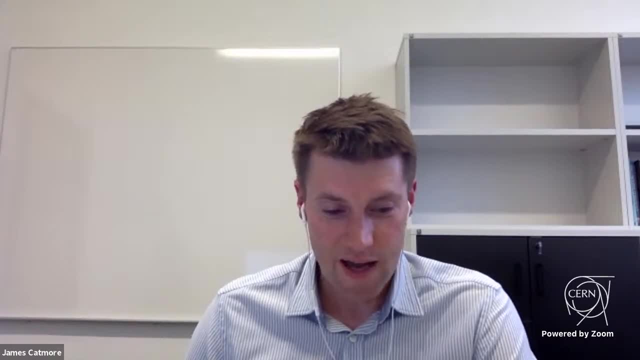 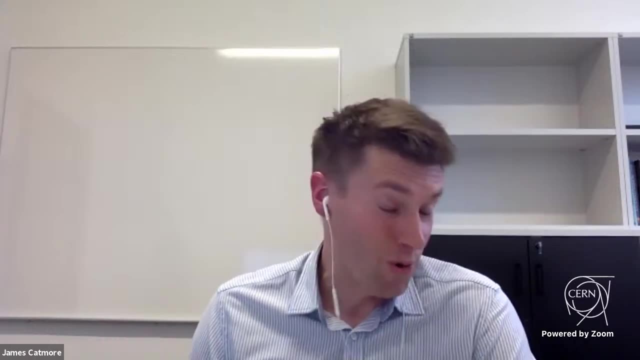 in terms of simpler machine learning techniques. it would be very difficult to do a lot of our physics without them. In fact, I would almost go as far as to say that almost not all, but almost all physics analysis now in ATLAS uses some kind of machine learning. 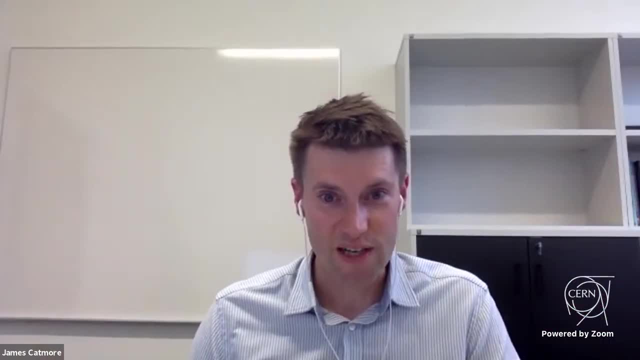 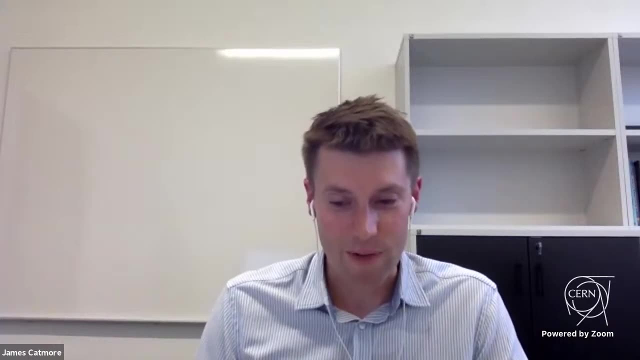 or multivariate analysis as we sometimes more traditionally call it, And the deep analysis is now starting to find its way into deep neural networks, and deep learning is starting to find its way into analysis. I think this is, by the way, clear that we're going to need another outreach talk. 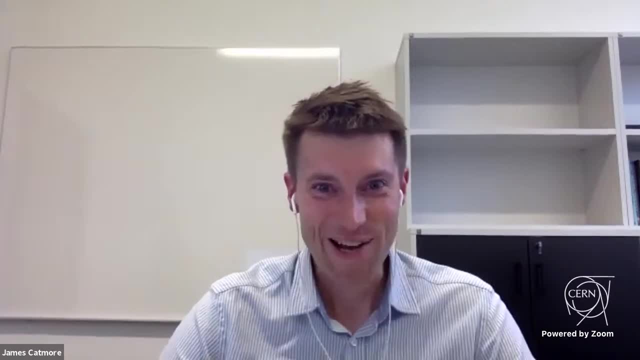 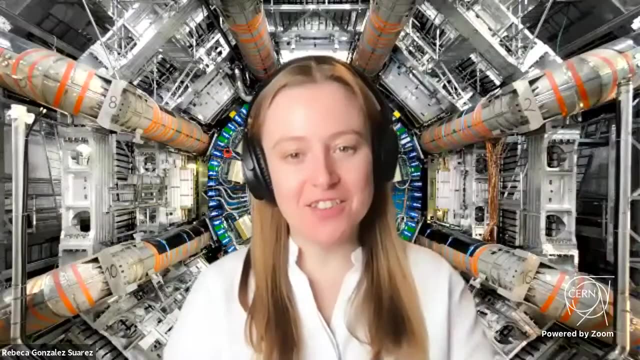 on machine learning and AI in physics, because I didn't have time to discuss much of it, but it's clearly something people are very interested in. Yeah, I think it's something that is coming up, so we can all look forward to that. 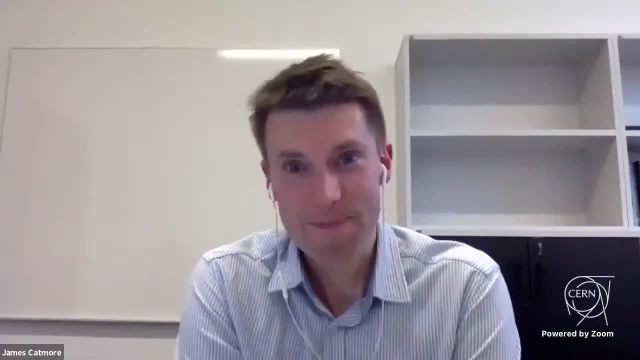 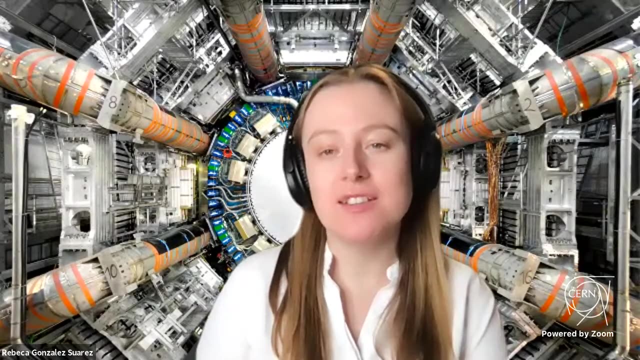 But it's obviously so related right that it's normal that the questions come All right. so then I think we can move on from the machine learning and just think about having this for a future talk and think about things that are a little bit more related. 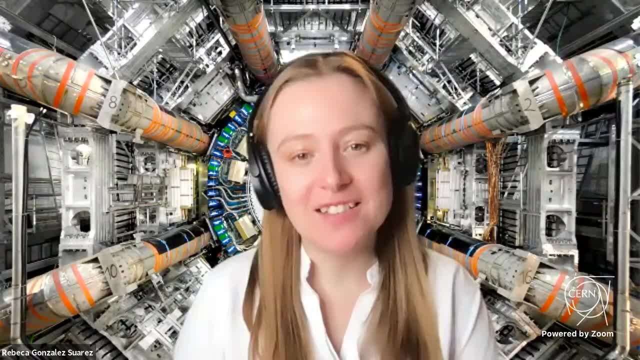 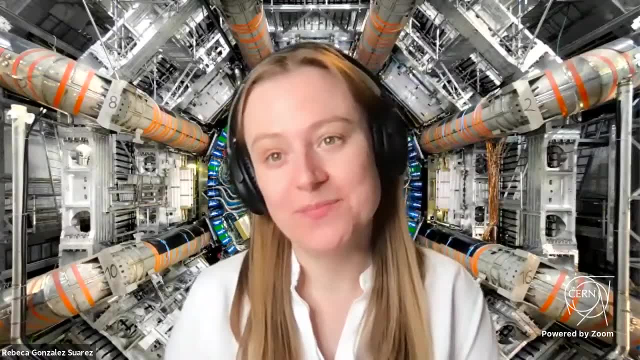 to your talk. So there is something that is being asked that I want to ask you. I don't know if you're going to know the answer, but how many lines of code does Atlas use Millions and millions? Actually, I wanted to look this number up. 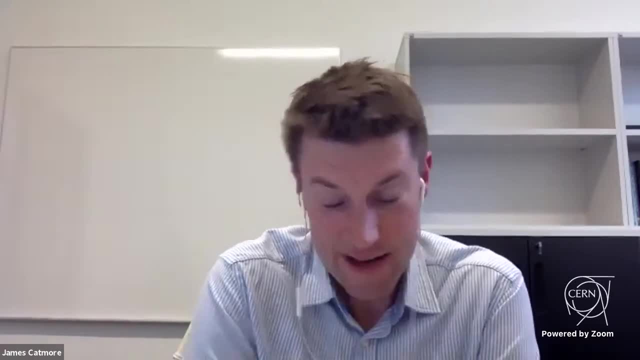 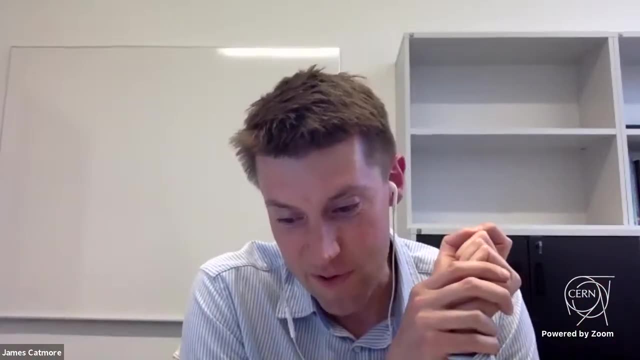 in order to put it in the code. but I was a bit in the slides but I was a bit reticent because there are different ways of defining. What I should have said is that some of the software we use particularly for the event generation, 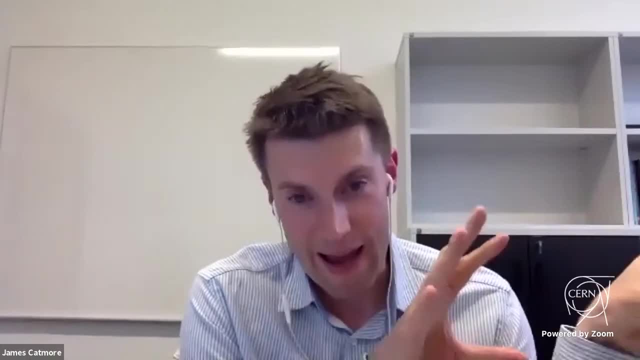 and for the simulation is not written by Atlas, It's written by bodies that are external to Atlas. And then there's the code which is in Atlas, And then there's the code which is in Atlas, And then, of course, you have to decide. 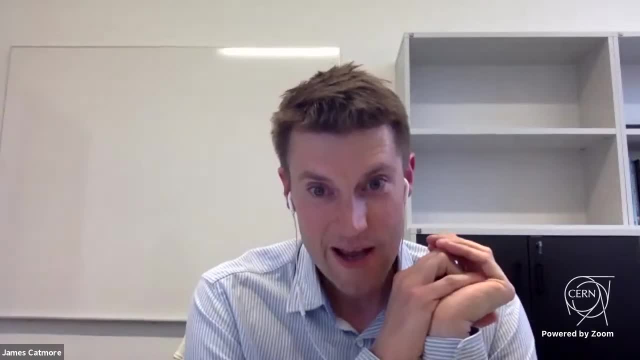 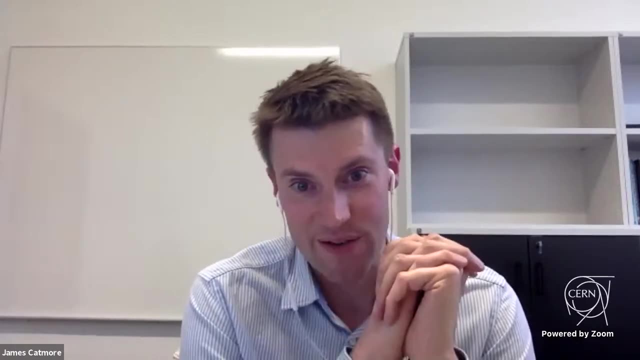 do you also count the analysis code? do you also count the analysis code which is written by physicists? But let's say we are talking about, let's say, millions of lines, not hundreds of millions of lines, but millions of lines, Some of it in C++. 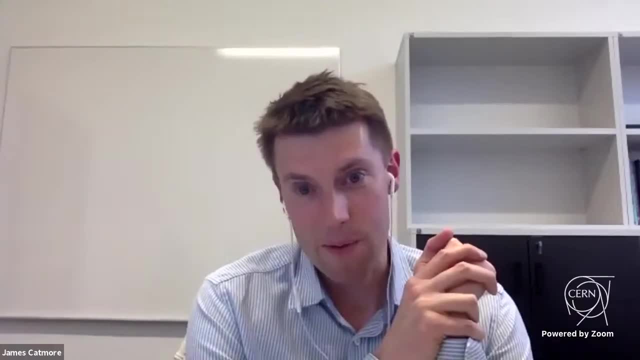 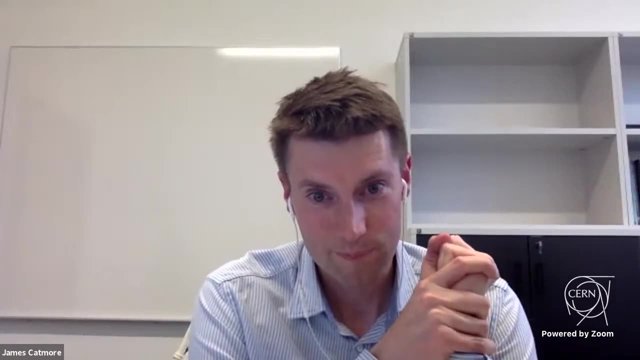 for the sort of hardcore calculations, And then some of it in Python, which is what we use for configuring the software And, as I said, it's also used a lot for analysis as well. And, as I said, it's also used a lot for analysis as well. 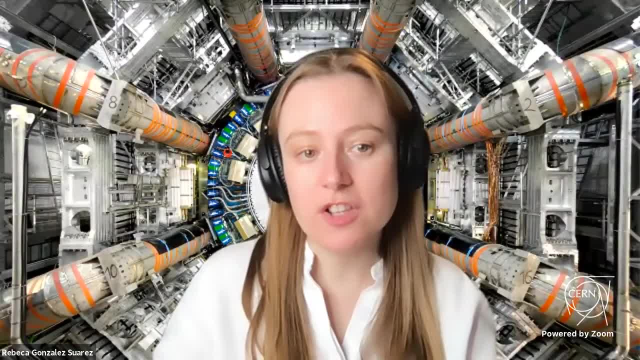 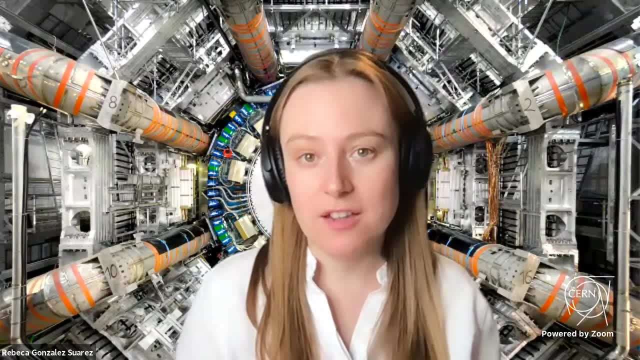 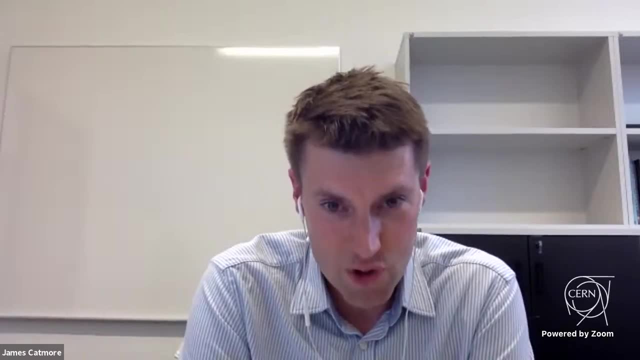 So I think you are asking- answering actually right now is actually right now a question that is also answered, but maybe you want to elaborate a little bit on that- that is, what software languages do you use to process data, right? so yeah, that's a that's a good question because, uh, c++ is our, what i would call our- core language. um, it's the language. 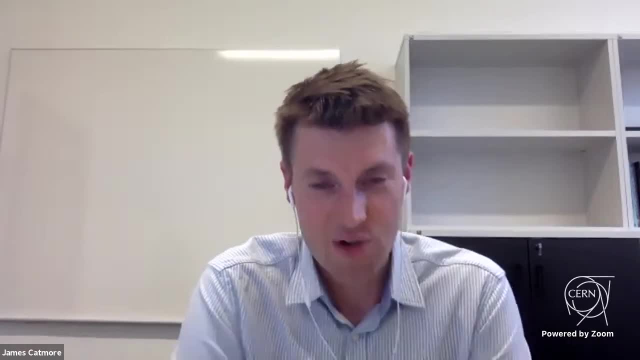 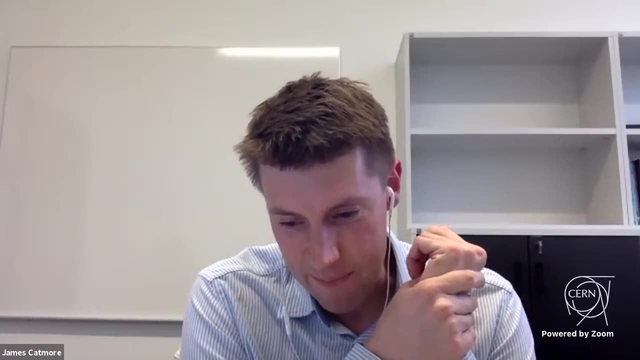 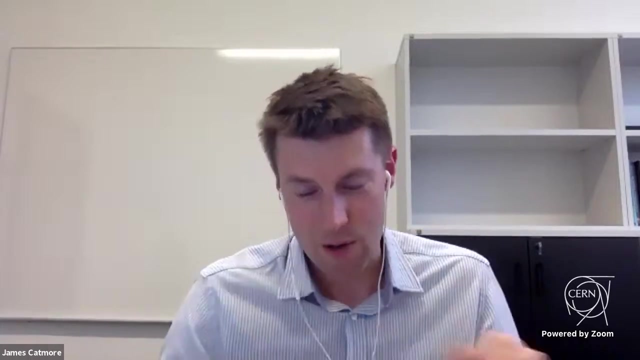 that we use for really doing the event generation simulation. when we have high, high volumes of calculations to do, we use c++. but c++, um, i mean it's, it's a tough language to to learn, it's, it's, it's quite complicated and, uh, you, you have, it's very powerful. but with power comes responsibility. 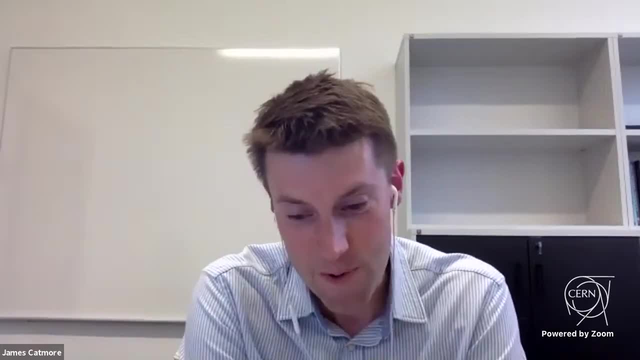 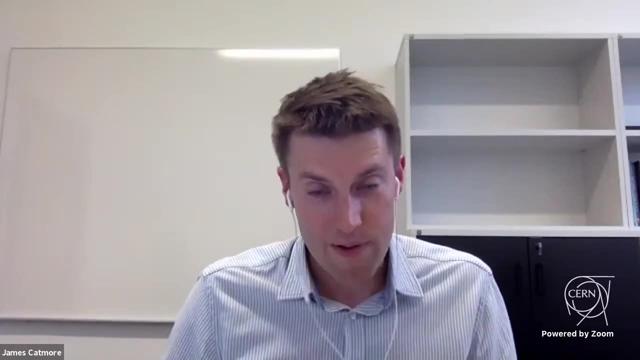 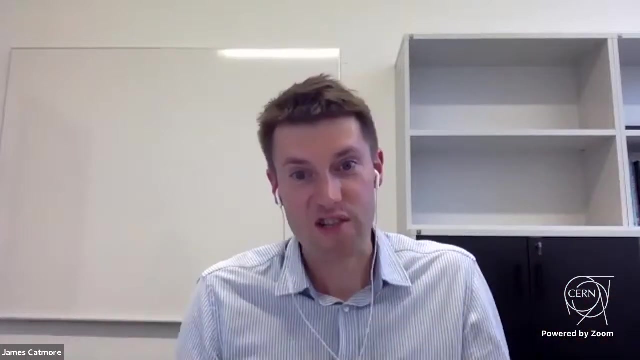 and it can be quite tricky to to get it right. so, um, for, for, uh, applications that are more facing, let's say, the user, we use python. so, for instance, we configure the software using python, so we give instructions rather than having. if we need to change the settings of the software, then we will use python. 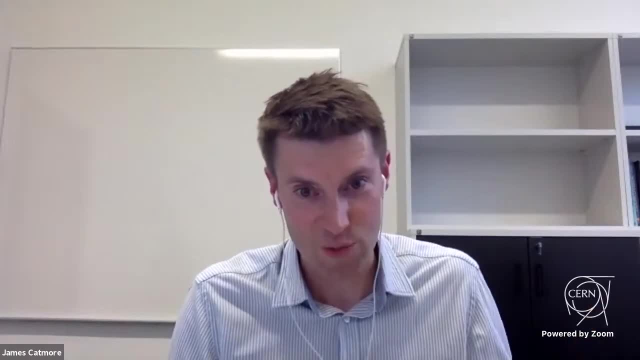 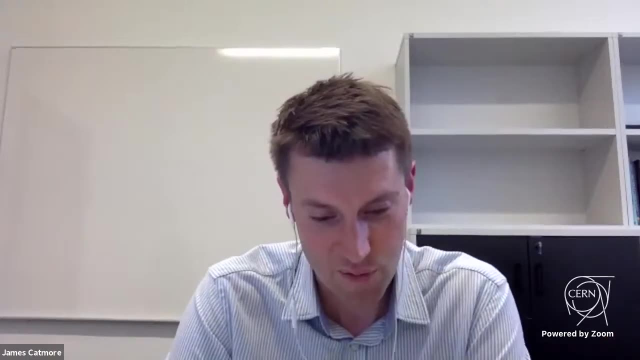 to change the settings. we don't change the c++. if we want to change the settings, we just use different python, uh, and that means that we can very easily uh change the configuration of the software without recompiling it. um, and also, as i said, although many people still use c++ for 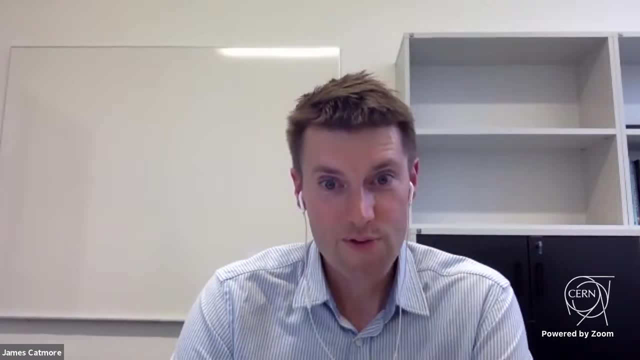 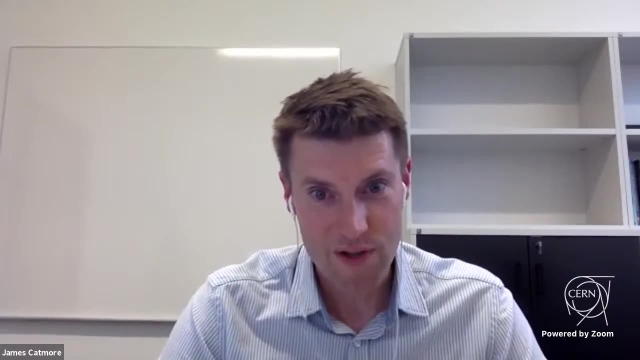 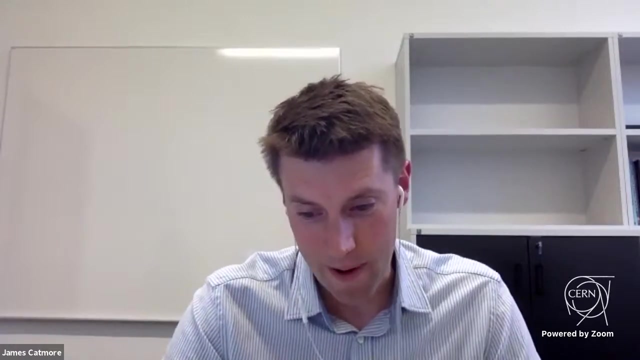 analysis. more and more people are now moving to python for their physics analysis just because python is a friendly user, user, user of doing things. it's more often taught in universities now than uh, than c++, so a lot of students come to uh to cern or to the experiments uh knowing more python than they. 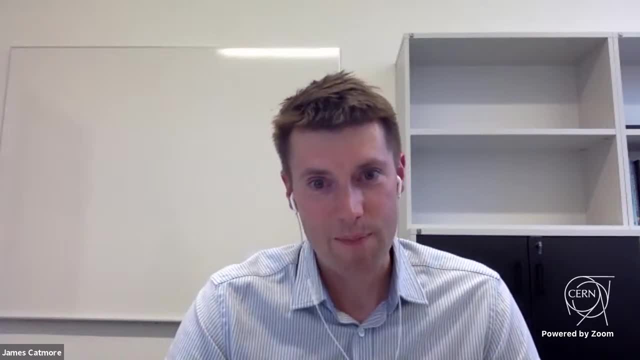 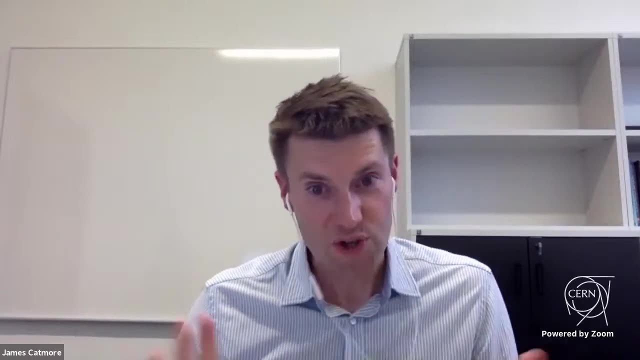 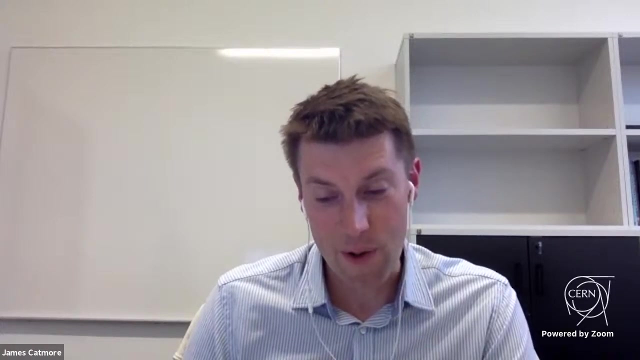 know c++ and also, uh, there's a lot of um software for, for instance, machine learning and for all kinds of graphics and so on, uh, which are also written in python, that you can just grab from the uh, from the internet. there it's freeware, uh, and and it's very well documented, and so a lot of physicists and 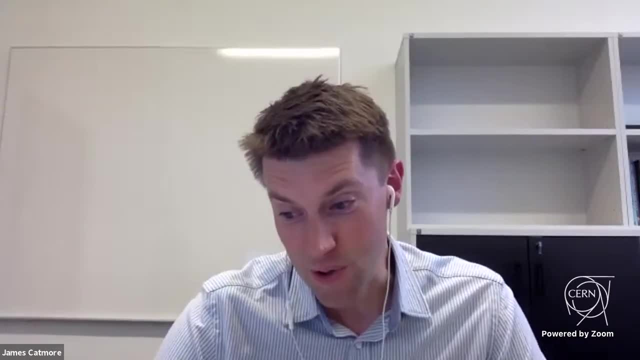 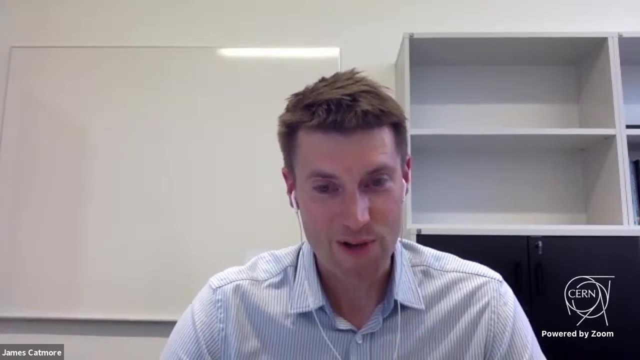 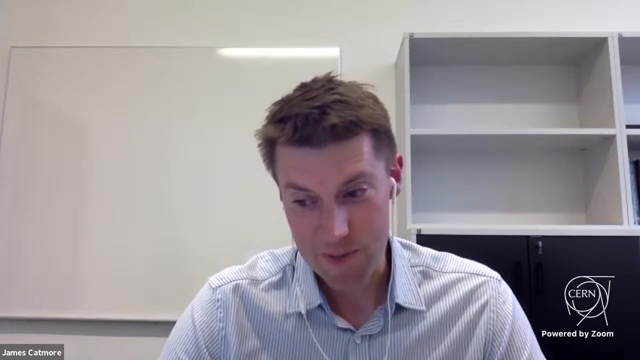 now using this? um. now, uh, when we go to uh gpus, that opens up another zoo. uh, because there are different languages for different manufacturers of gpu. so the biggest manufacturer of gpu is nvidia that uses a programming language called cuda, which is very similar to c++, but it has certain 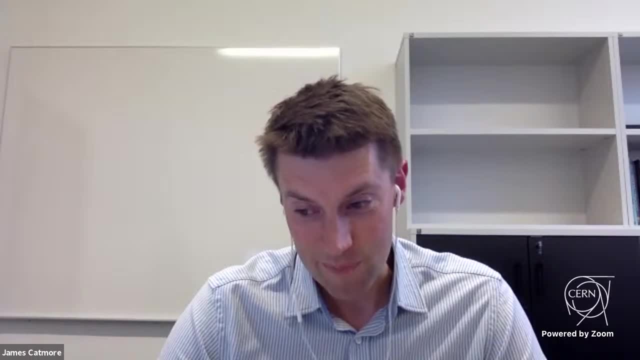 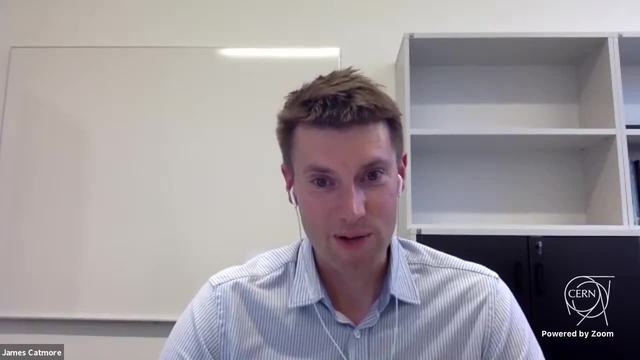 special features and different manufacturers have different proprietary languages, so that's going to be actually a big challenge when we start using gpus. how are we going to be able to write one version of the c++ and how are we going to be able to write one version of the c++ and how are 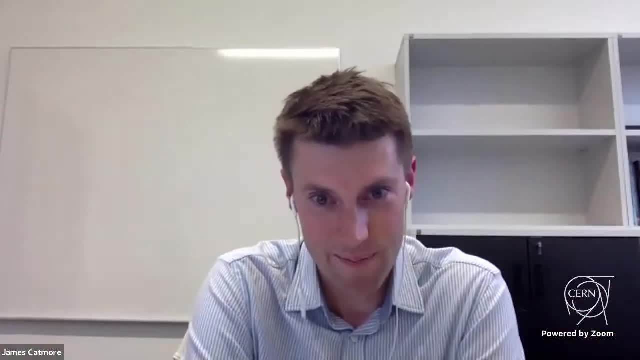 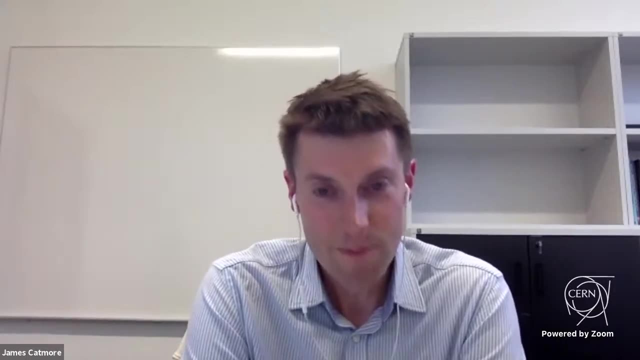 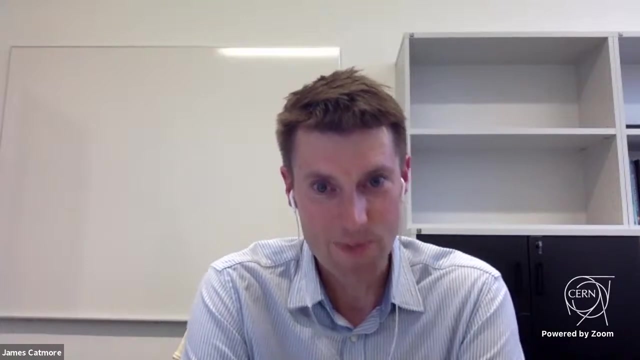 the software for all of these different kinds of uh, of um, of gpu. so yeah, to answer the question, c++ for the heavy duty stuff, python for the configuration and um and and then uh, yeah, potentially uh other other things when it gets to uh to gpus. all right, i think that's a very nice. 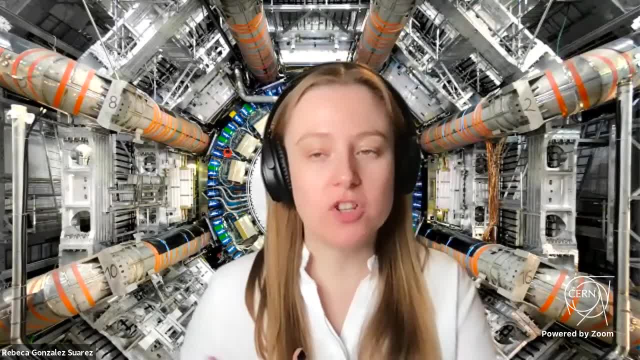 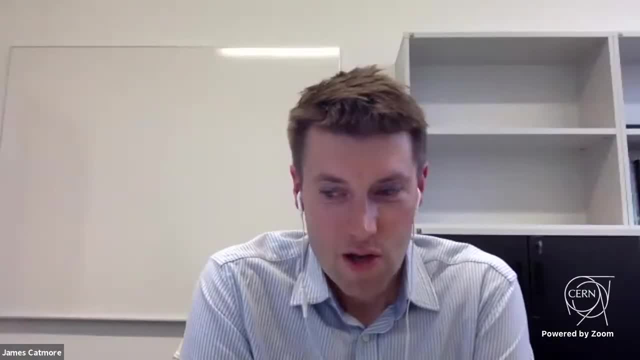 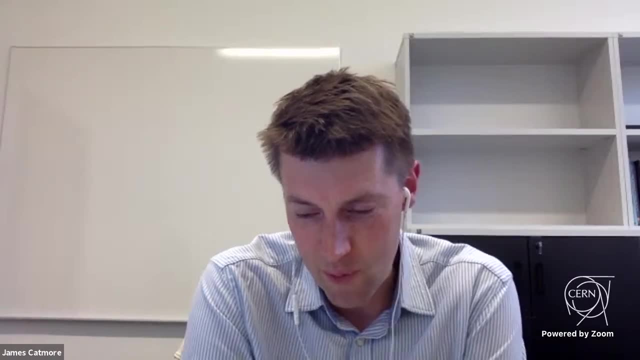 comprehensive answer. so, following up on this one, there is a question about what kind of applications are actually used. so it's not, it's a little bit beyond the the languages. yeah, so well, um, in terms of the data processing frameworks, uh, that we are, that, we that. 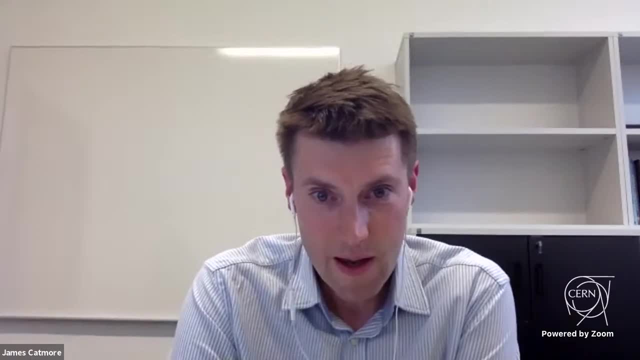 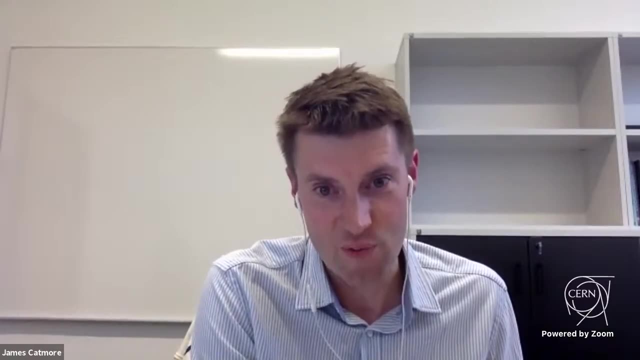 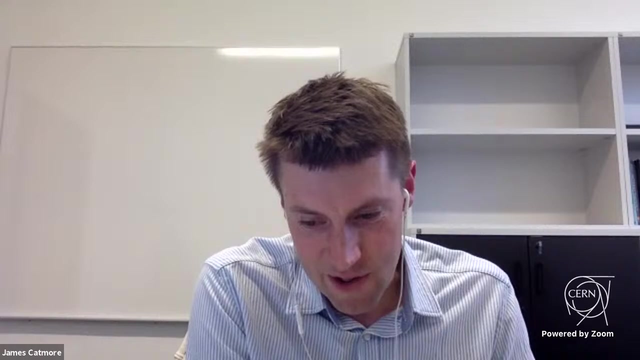 we use in atlas. it's a homemade thing called athena, and this is a c++ based framework and that's the framework which drives, when we're running it, the event generation, the simulation, the reconstruction, um, and that's, uh, that's our sort of big framework and, um, there are software. 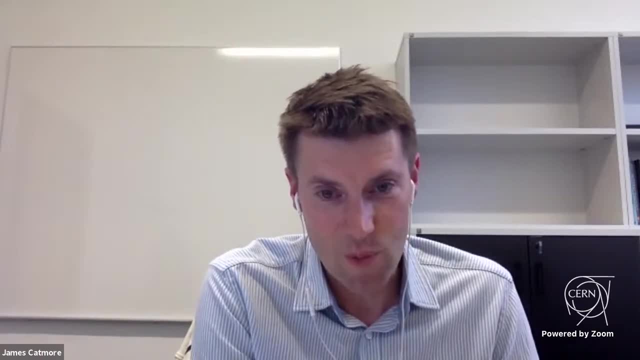 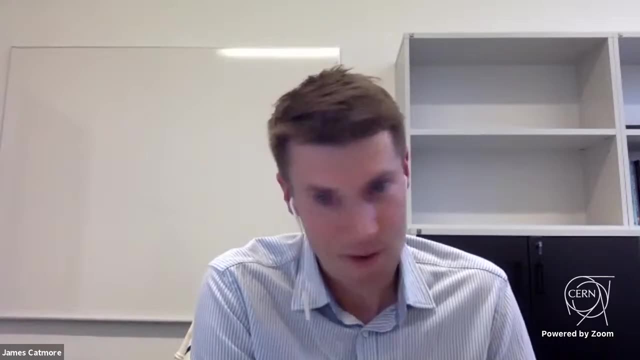 external software packages that plug into this and that's a big framework and that's a big framework, uh, that we use for doing the event generation. so there are event generators with names like pithier and herwig and these are all written by, by researchers in different uh universities and 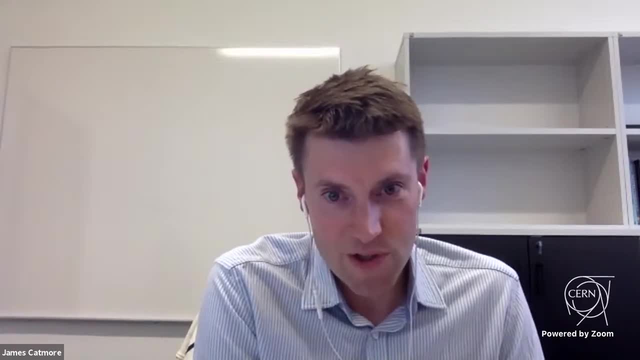 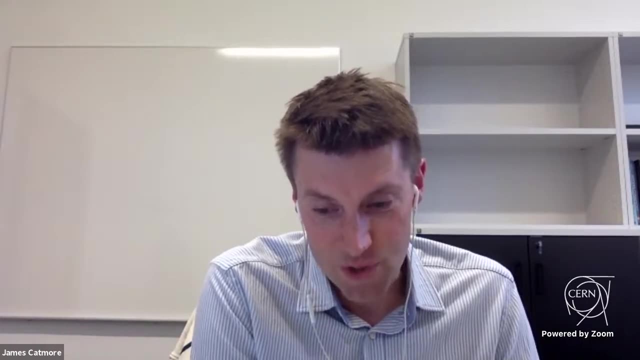 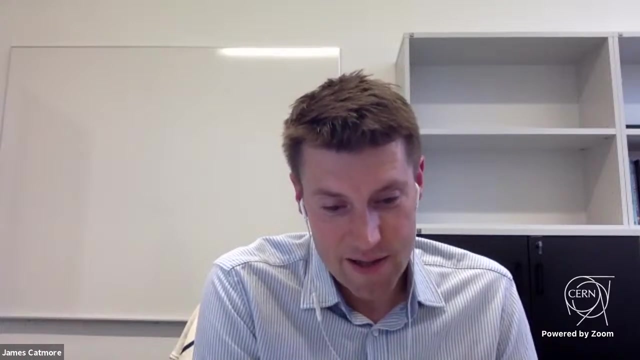 laboratories. the big simulation package that we use is called giant four. uh, that's written mainly by: uh. well, it's a big collaboration, um, and that also plugs into our athena framework for doing uh, simulation and then for analysis, uh, we use something called root. now, root. 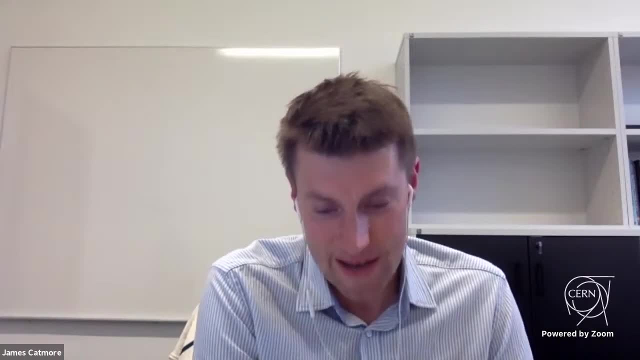 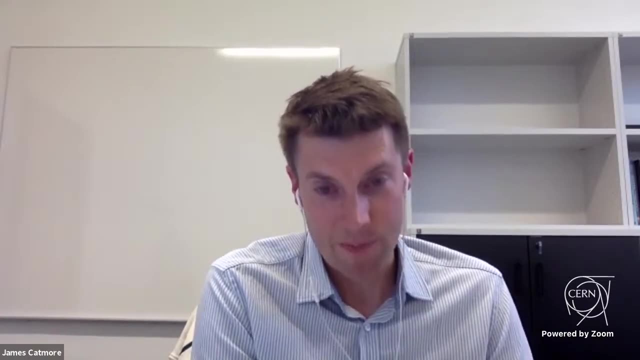 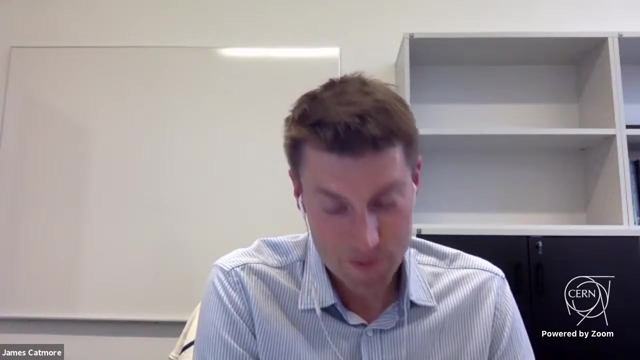 is a big software framework which is known by everyone in in particle physics and it provides many things. it provides an interface for doing analysis in both c++ and in python. it provides, uh software for drawing plots, histograms and other kinds of plots, all of the plots that many of the plots, at least, that you see coming out of cern have been. 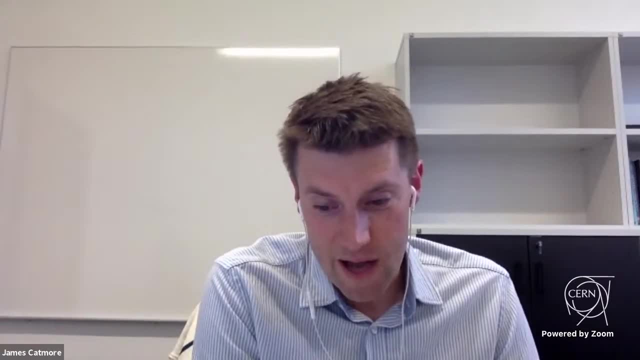 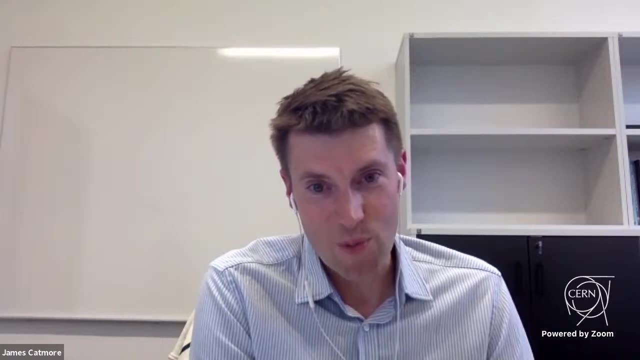 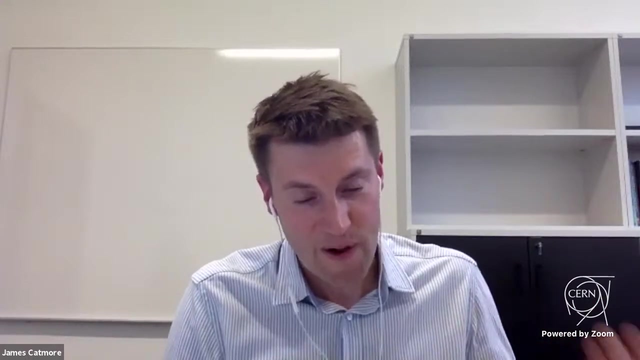 drawn using root, but it also provides, um, what we call an io layer, an input output layer. so all the data formats, or most of the data formats that we write in in atlas, are based on this root, uh, io layer. so, uh, most of the files can be read using this root framework as well. and then the 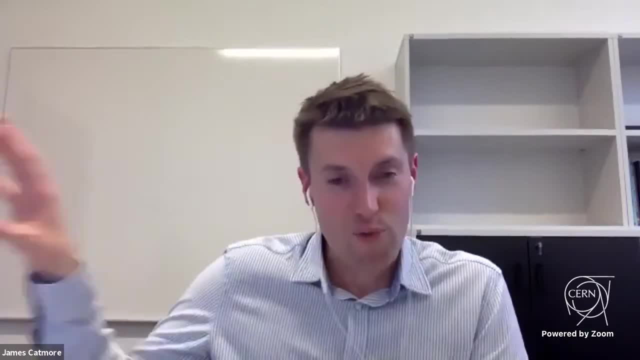 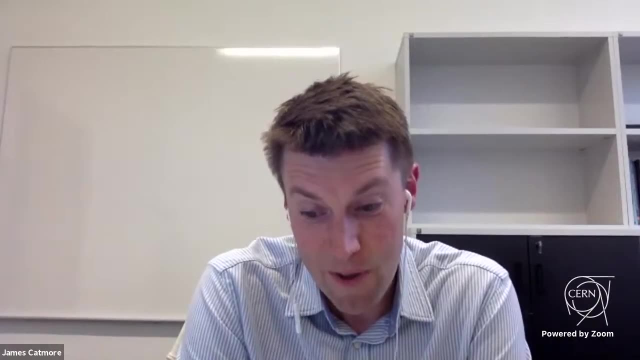 root framework itself can plug into other software packages. these things, uh, based on python that i mentioned, we can. we can make use of um of these. so yeah, for for a person on atlas, um, the, the, the data approach, the main application is um, is is athena for. 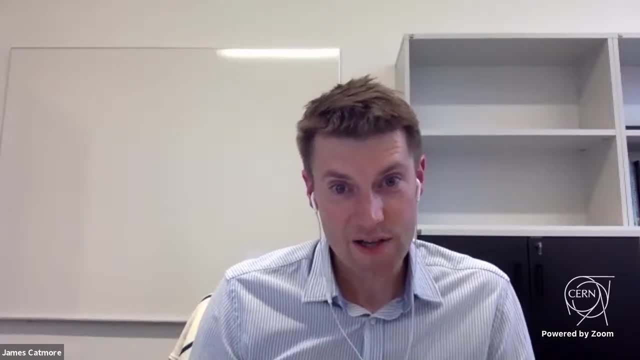 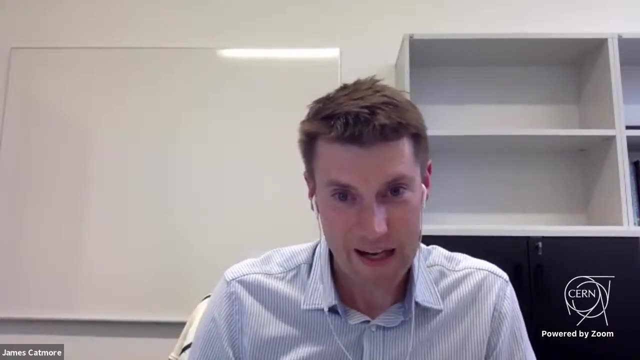 for for doing this bulk processing, but the average analyst will most often be interacting with root, with jupyter notebooks to do their, their python, with things like psychic learn and this. these are the sort of things which um data scientists in other fields would be very, um, very familiar. 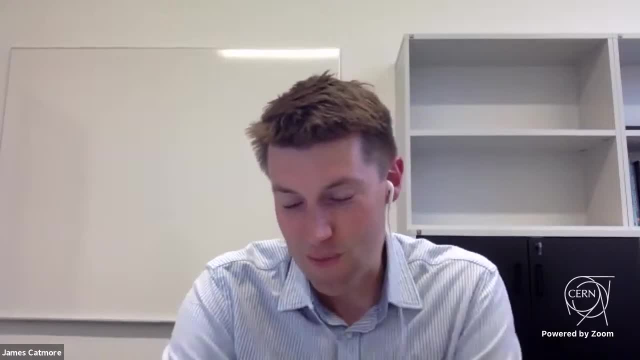 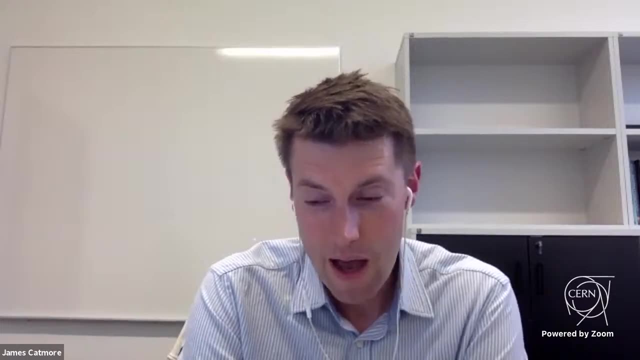 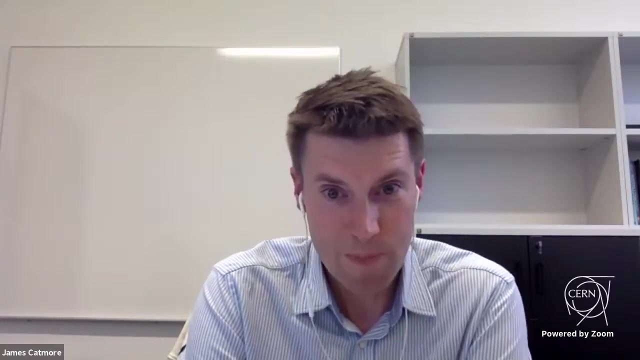 with um and then- and i mean, i guess the question people might also think: what uh operating systems do we use well, for doing the bulk data processing? we use linux, um and uh. a lot of people use linux personally as well, on their laptops. uh, and then a lot of people use max. 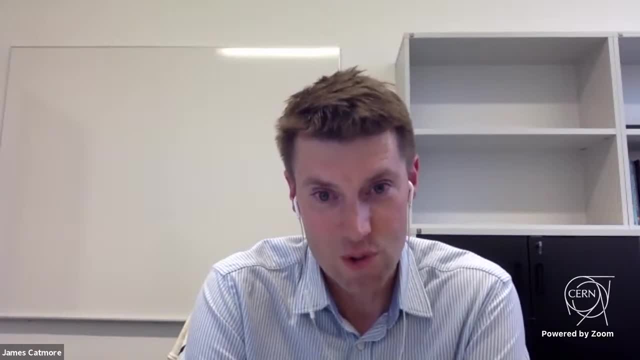 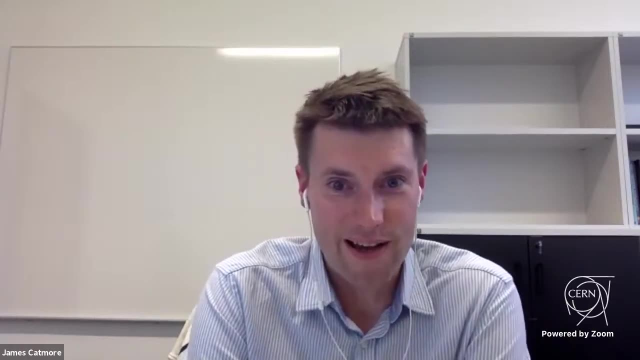 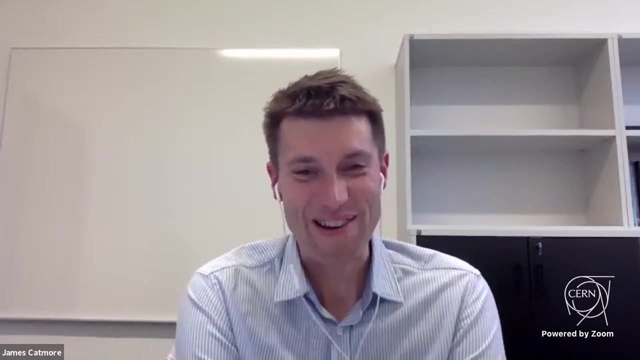 for um, because all of these uh analysis tools root will run on a mac, for instance, as will all this python based stuff, um and yeah. so that's uh, that's kind of the uh, the applications that we, um, we tend to use. we don't use spreadsheets very often. that's the one application that we don't. 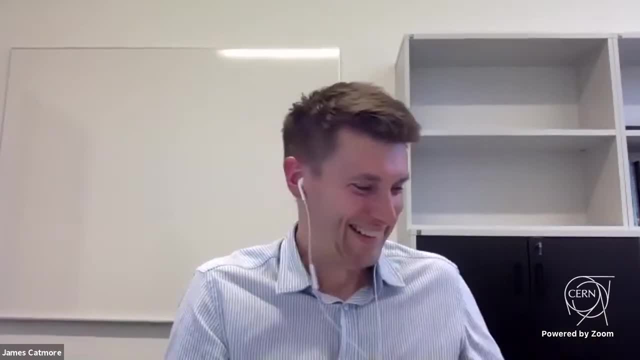 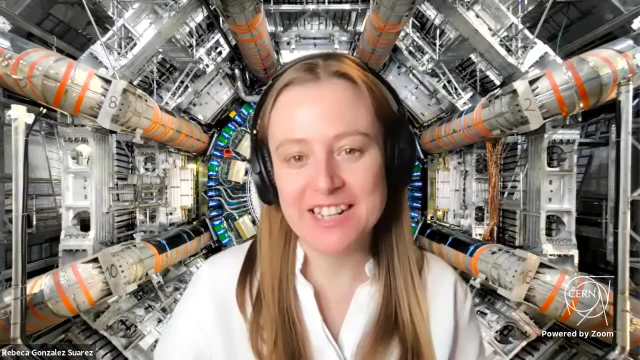 really use very often in uh in physics research. that's true, all right, so thank you for the answer. i think it was uh very comprehensive and uh very nice, but maybe it's time to come back a little bit to trigger. i think it's trigger has caught the attention of the audience today, so 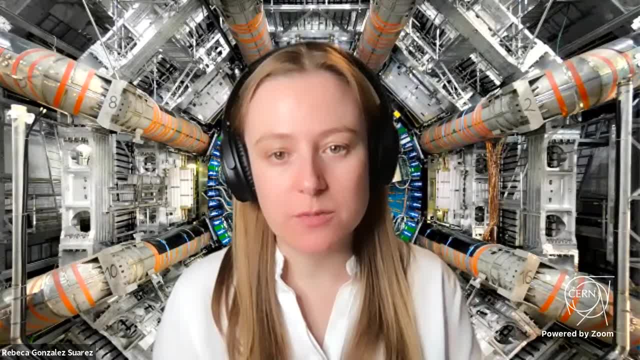 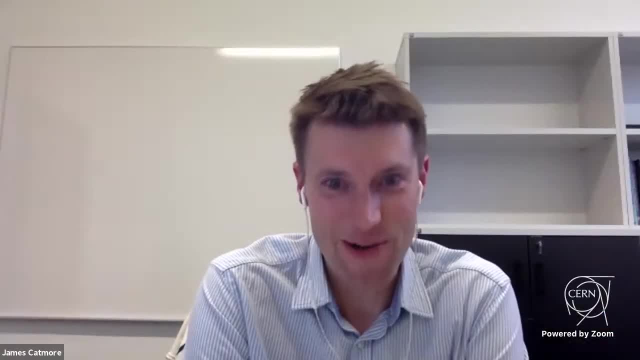 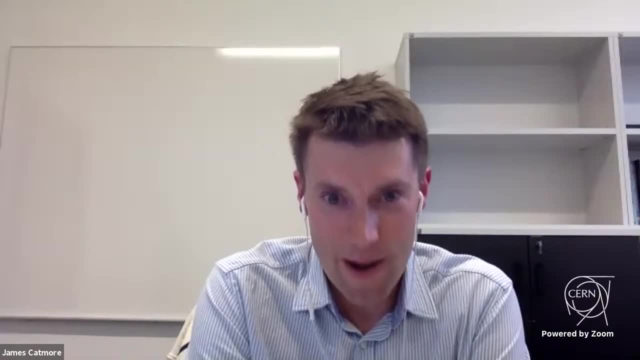 how sure are the physicists that the trigger selection does not reject possible new physics events that might have different signatures than otherwise? that's a very, very good question and the answer is: we don't know. um, we don't know for a fact that we are not throwing away new physics. 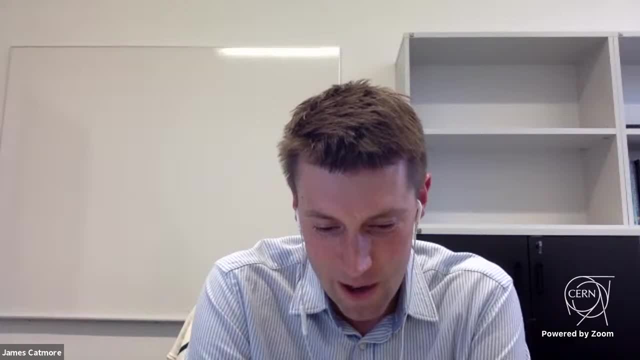 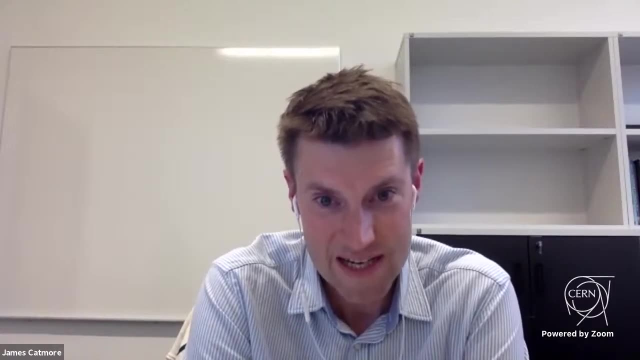 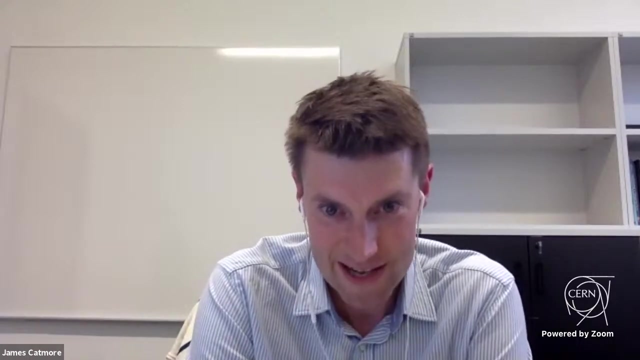 um, the problem is that, um, we are not able to because, as i said earlier, if we wanted to record every single event that the uh atlas experiment sees, uh, we would need, you know, the colossal amount of storage at 60 terabytes a second, or something like that. so we have to make choices, and the choices that we make. 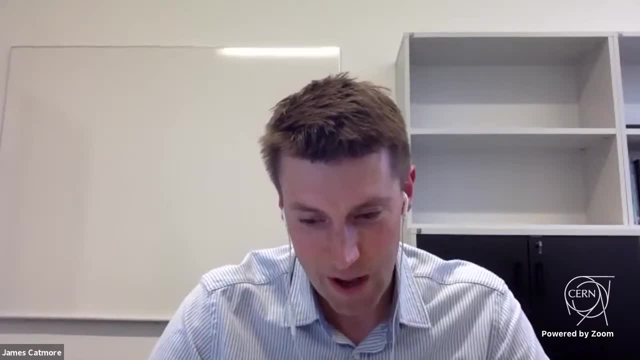 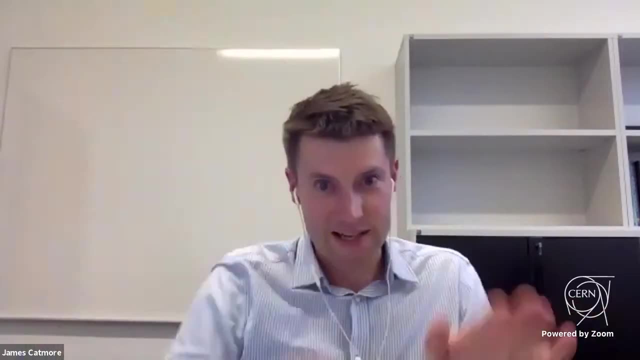 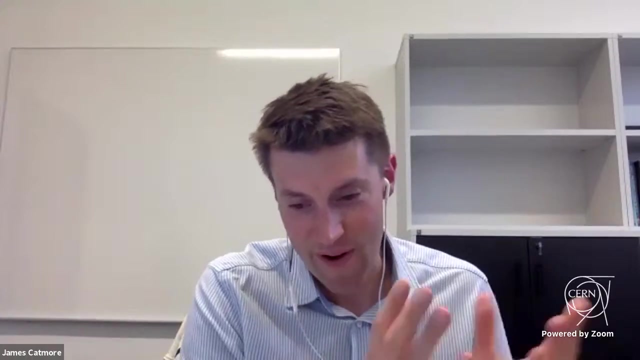 are that we we look primarily for what we call high momentum, high transverse momentum, so where the physics signature goes straight into the, the main bulk of the detector, at rather a high angle, or very high energy events, or events with very large jet, or with very energetic jets where lots of particles appear to be focused into a very small. 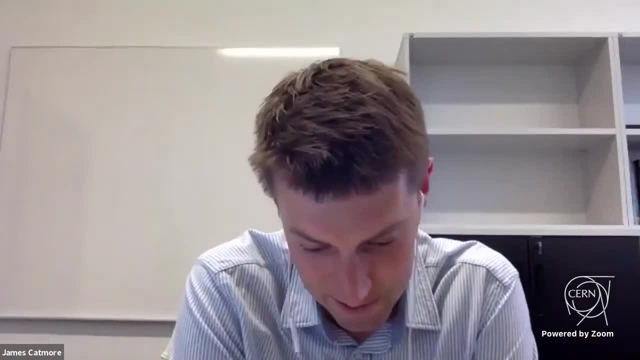 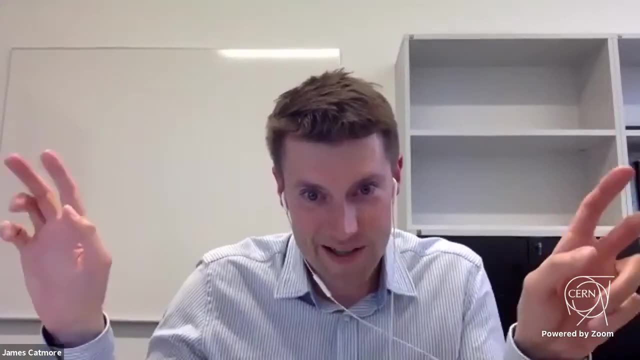 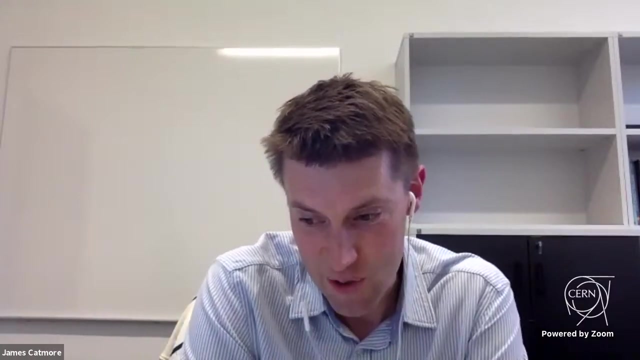 space that leave a very obvious signature behind in the detector. now we can uh record a small fraction of the- uh what we call lower, let's say lower transverse momentum events, but we can't afford to store all of them, because the data volumes are just too big. 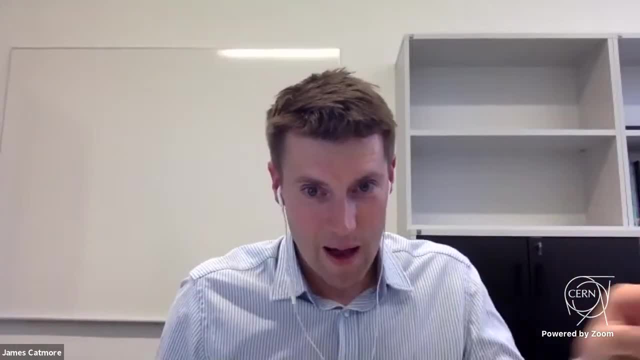 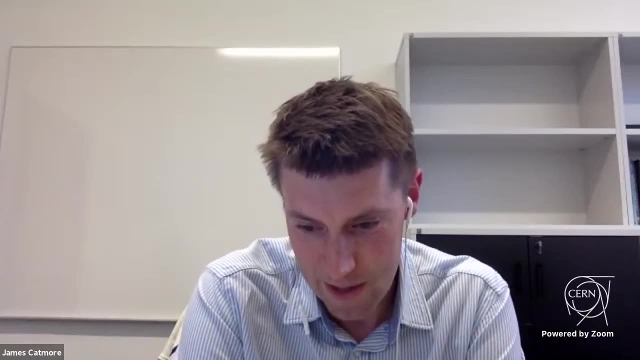 so we can sort of look at small fractions of them, um, and to see if there's anything interesting there. the other thing that we might be able to do in in in the future- and this is: people are looking at this and i think probably the talk from from christian that was already on youtube may have. 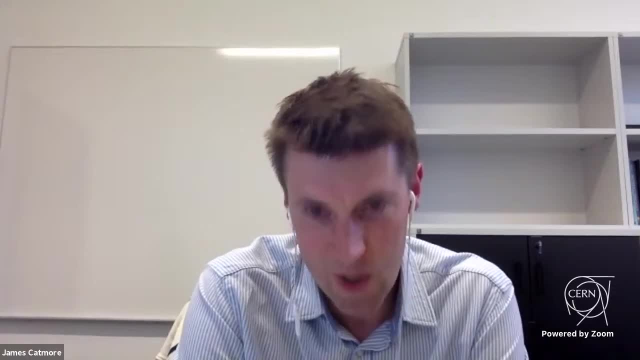 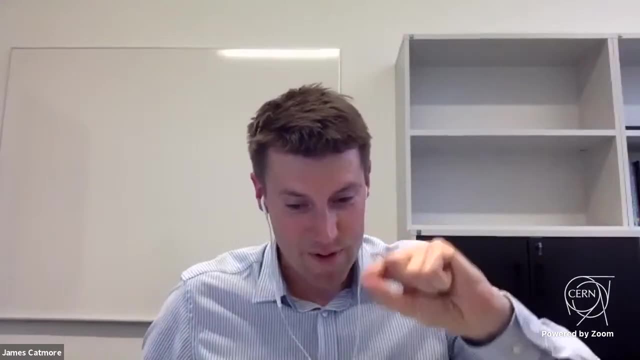 talked about this. the dark matter talk is that we can look at long-lived particles where something flies, uh really along. most particles, they, they, uh decay- the new, the, the heavy particles, they decay inside the beam pipe. so by the time atlas seems like it's going to be a long-lived particle. 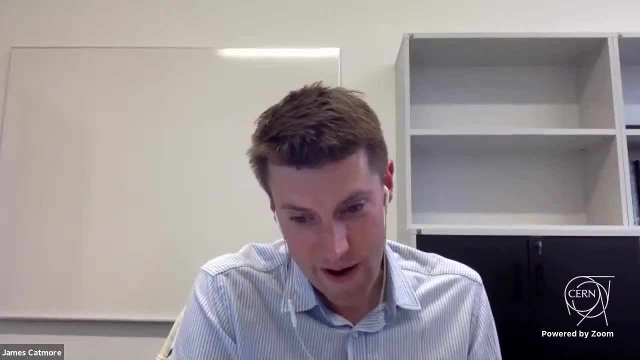 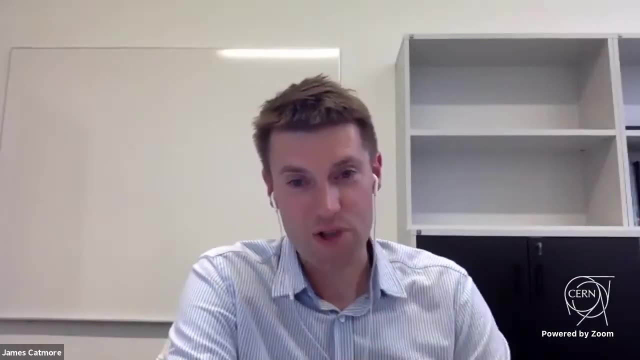 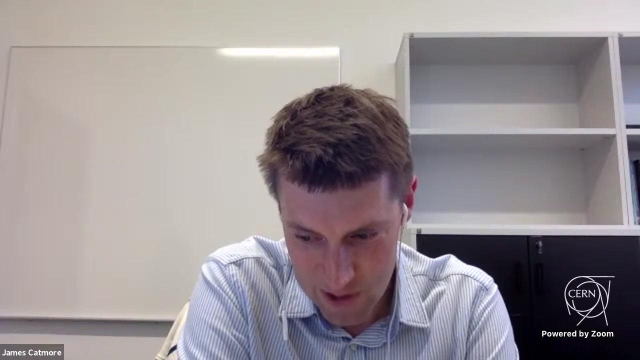 but it's possible that there are new. some new physics models give you a particle that can fly quite deep into the detector and this is something that we could also um trigger on. but again, to come back really to the question that the, uh, the, the, the viewer has asked, we don't know for a fact that 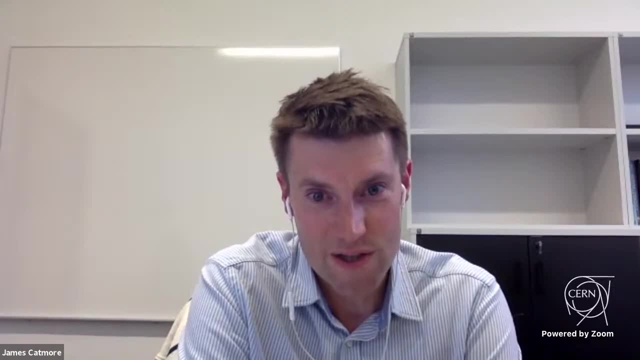 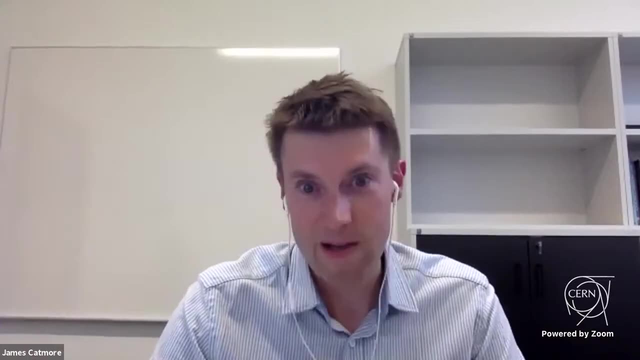 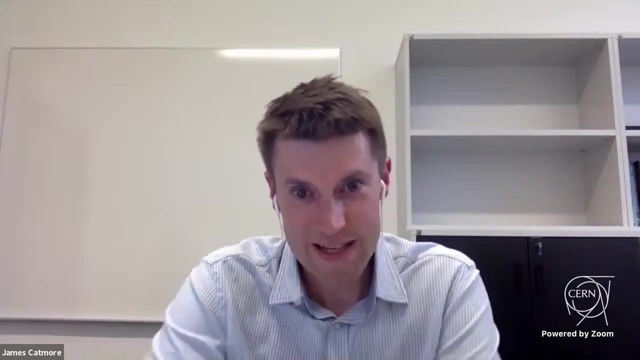 we have not thrown away interesting physics and we do have to make choices based on our assumptions about what new physics will look like. but as soon as we switch on that trigger, we are biasing the data. we call the trigger that looks at the very um low angle data, this low pt data. we 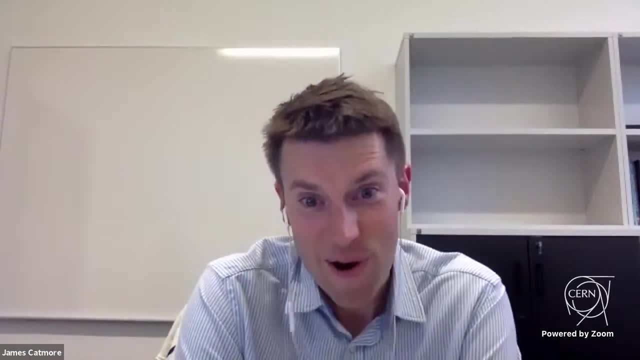 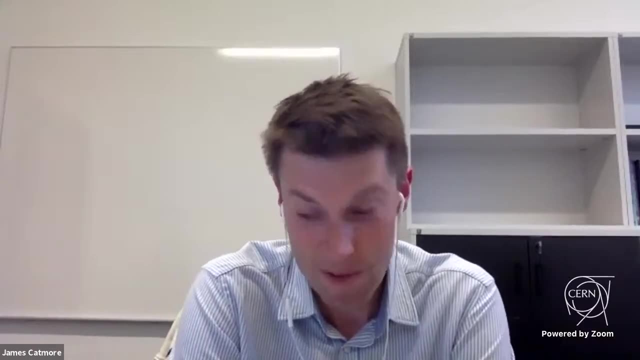 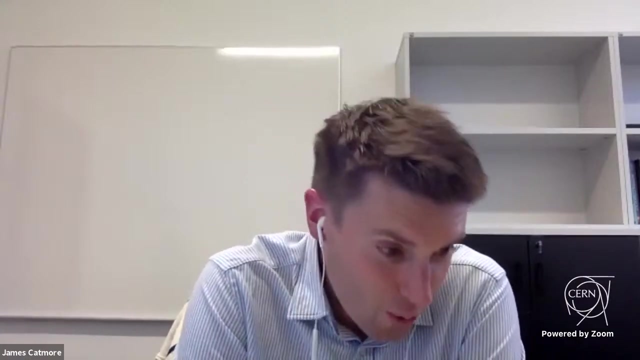 call that the minimum bias trigger, but it's not, uh, zero bias, you know, i mean it's still. there's still some bias if you want both ends of the detector to be lighting up at the same time. so the answer is yeah, the the trigger is, um, is is the thing that enables us to work with a reasonable 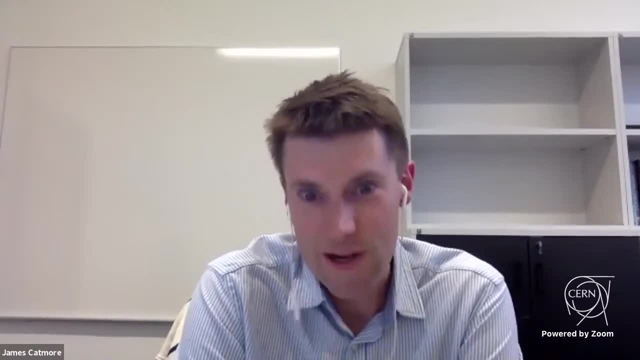 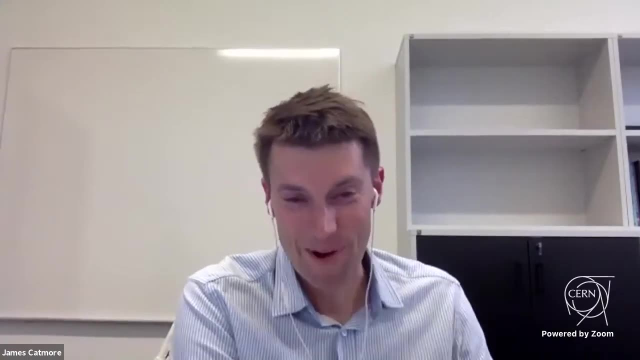 amount of data that we can handle, but equally, we have no guarantee that we are not throwing away interesting physics and that's um, that that's the life of, uh, of experimental particle physics. yeah, yeah, we have to live with that. we have to live with it exactly. 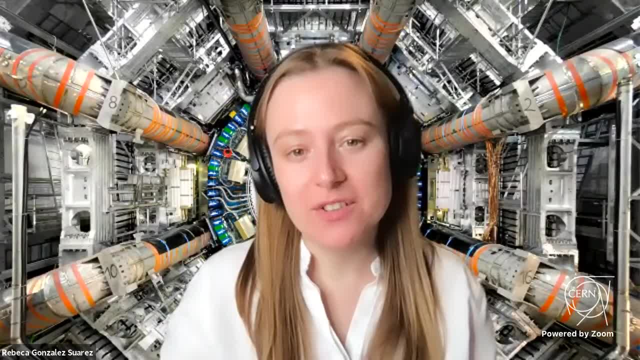 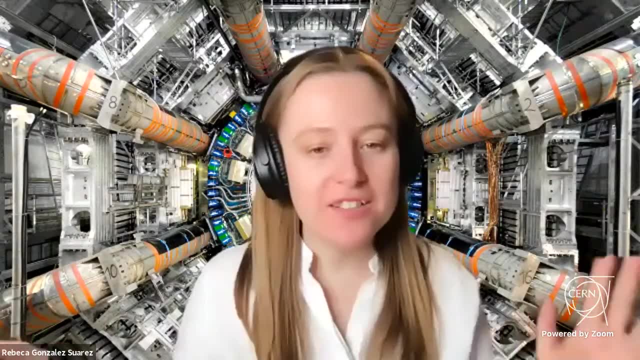 well. thank you very much for that answer. i think it was. it was also great, and i'm happy that you touched only particles that are very dear to my heart. so all right. so now for a completely change of topic and something that i was sure was gonna come out in this talk. the next question is the. 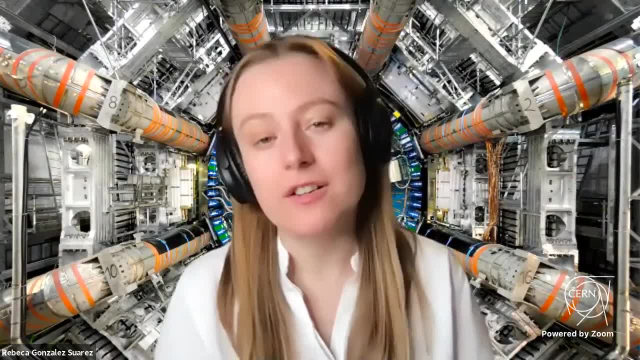 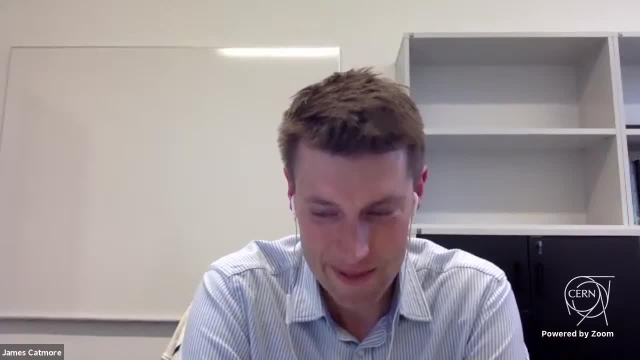 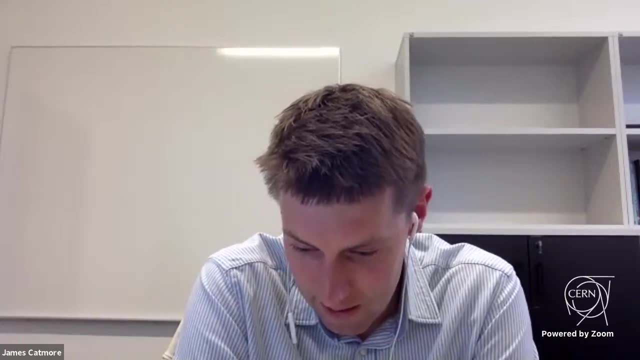 following: is quantum computing being used to control the energy of the universe, or is it just a concern or address, right? i was thinking about making a slide on quantum computing, uh, and then i, um, decided against it. i was also expecting this question, so now then, um, the people are. 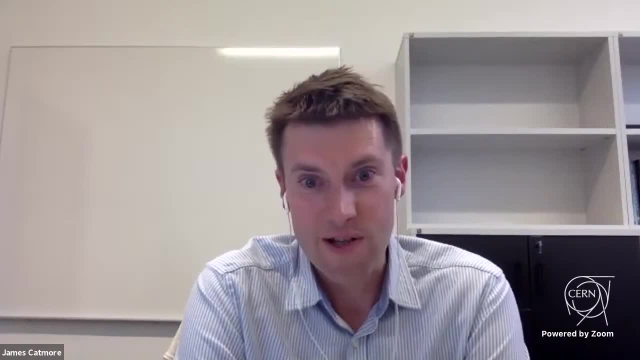 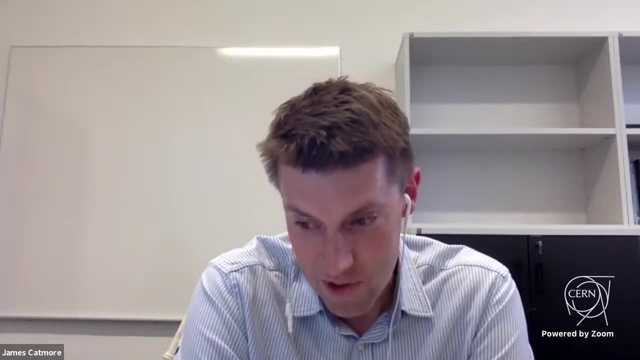 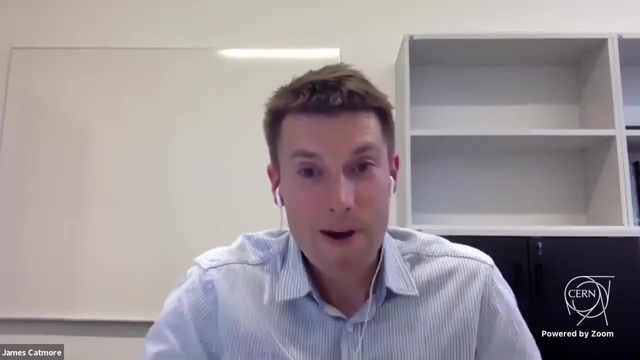 definitely looking at quantum computing, um, in various uh experiments, including atlas, and you, you see, talks about this. now, what should be stressed is that at the moment, uh, quantum computers of the kind that we could use in experimental particle physics don't exist. maybe i should explain a little, uh, in my limited knowledge. 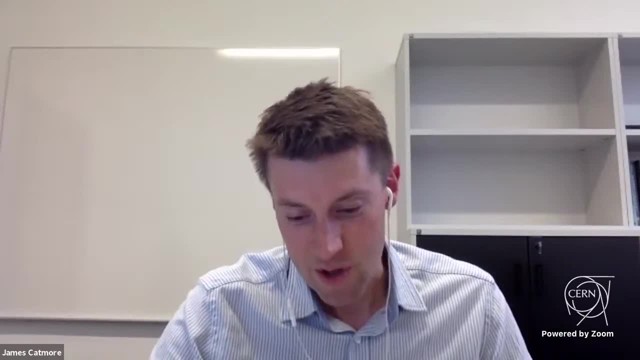 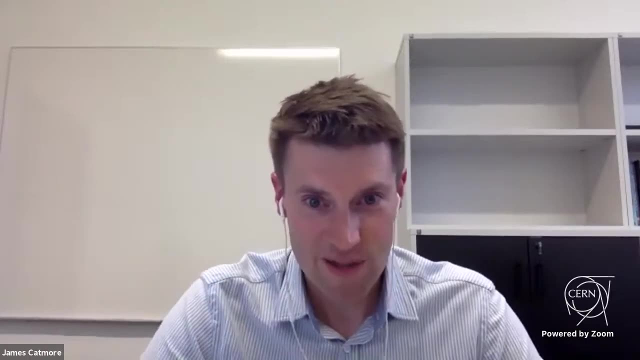 of quantum computers what they actually are for those who who don't know so. whereas with a classical computer the bits are either zero or one these bits that i showed, with a quantum computer you have something called a qubit, where, through the magic of quantum mechanics, you can have a 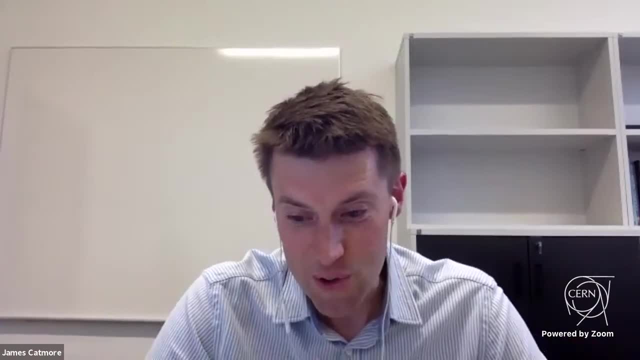 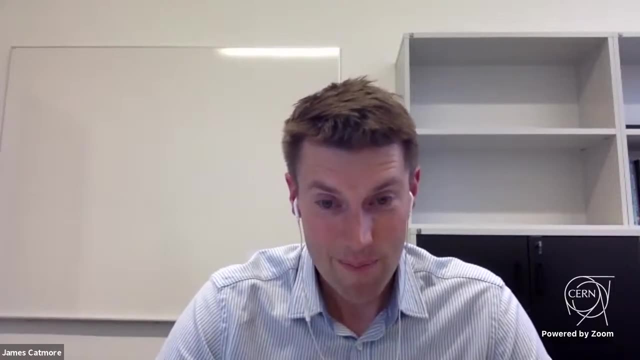 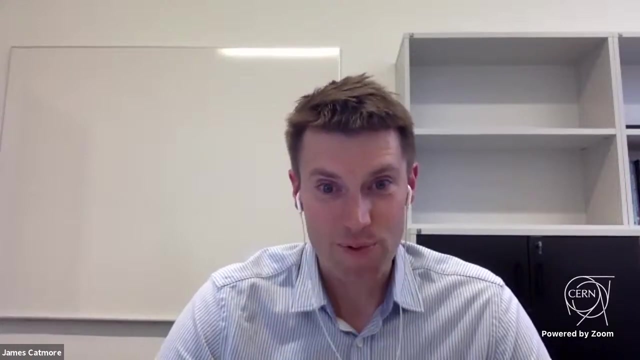 combination of zeros or ones, and this enables you in in theory at least, to do certain kinds of calculation far, for far, far faster um than a, than a classical computer can do. but the problem at the moment is quantum computers in any meaningful sense don't really exist in a form that we could actually use them. so at the 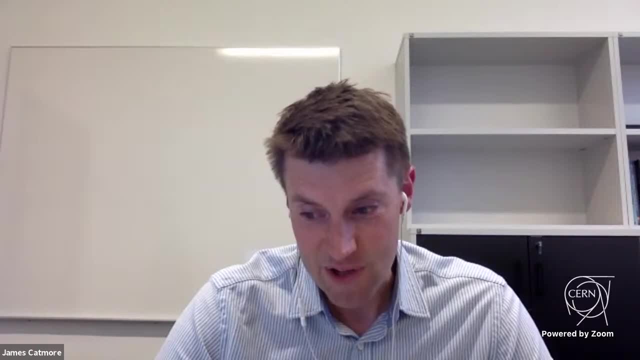 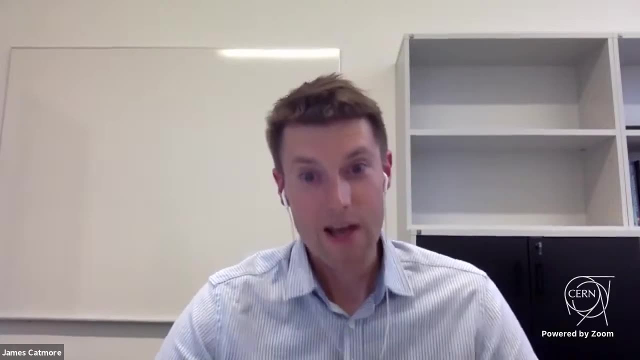 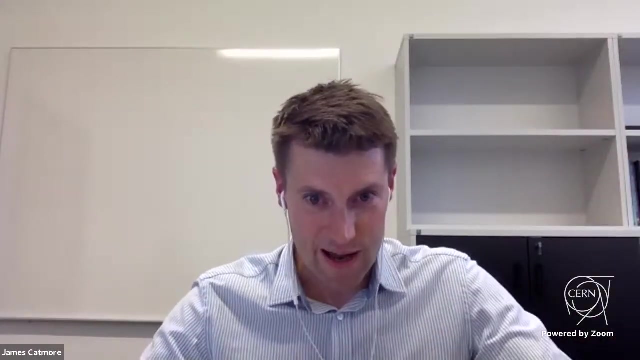 moment, the work that people are doing um across the different uh physics experiments in in uh at cern is that they're simulate, they're using simulations of quantum computers. so a a normal computer simulates how a quantum computer would work. and then these uh people try to work on programs that will computer, programs that could run on a. 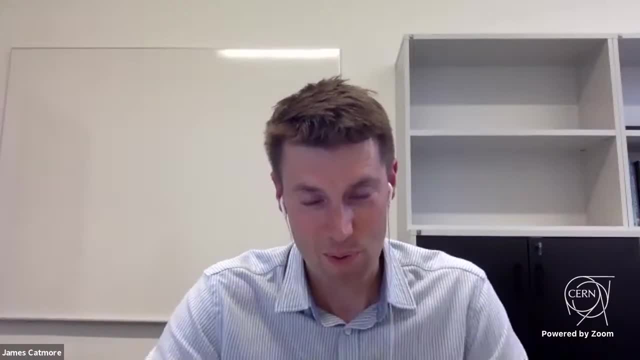 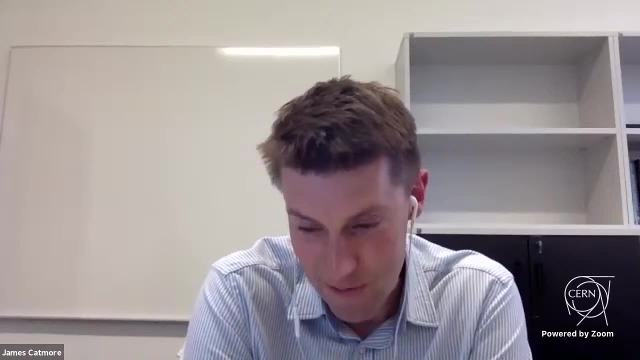 quantum computer, should it, in the future, uh, be brought into being? now i give you a an alert that i'm going to give you an opinion right now. maybe i will be proved totally wrong about this. my personal view is i do not believe that quantum computers will be able to help, as 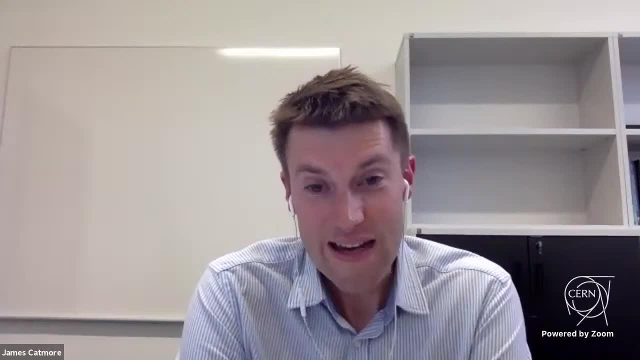 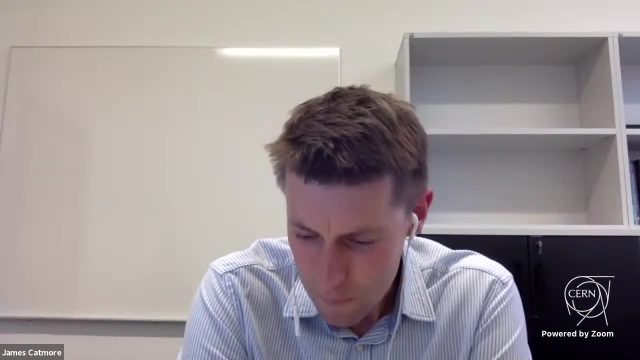 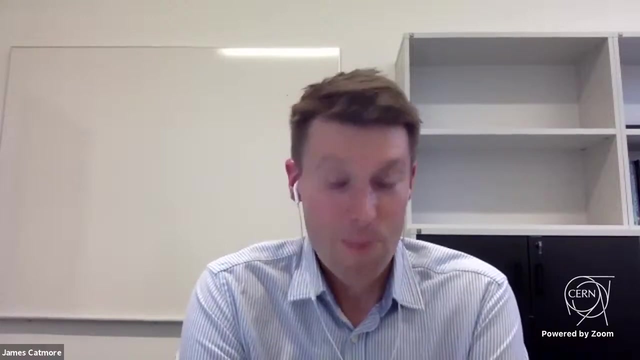 much for the high luminosity lhc. that's the phase of the lhc that will start in the late 2020s. even even quite um aggressive predictions for quantum computers are talking about something like 20 or 30 years before practical, usable quantum computers are are made available. 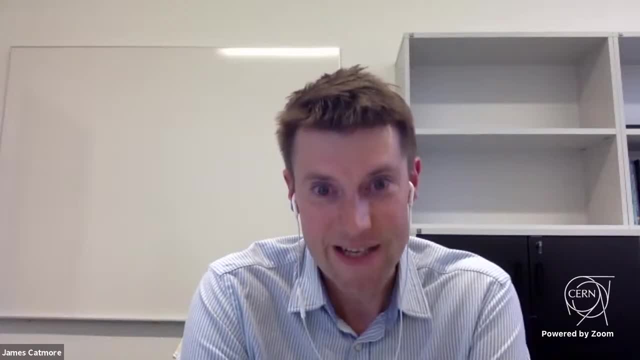 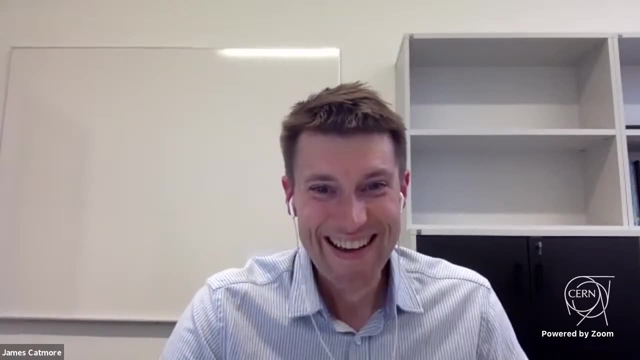 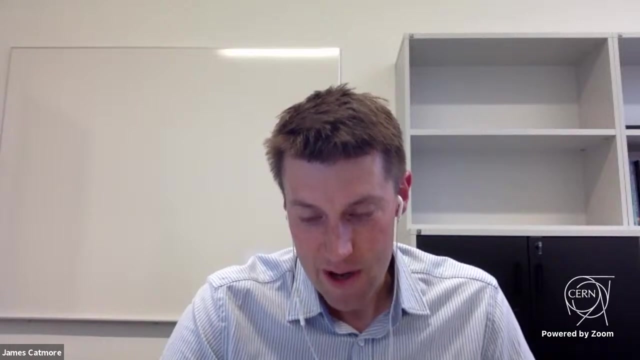 and that kind of takes us out of the um immediate uh use. so from my perspective, what i'm interested in is gpus, because they definitely exist, uh, we can buy them now. it's certainly important that people work on on quantum computing, but i think this is a very, very futuristic um thing and i i suspect 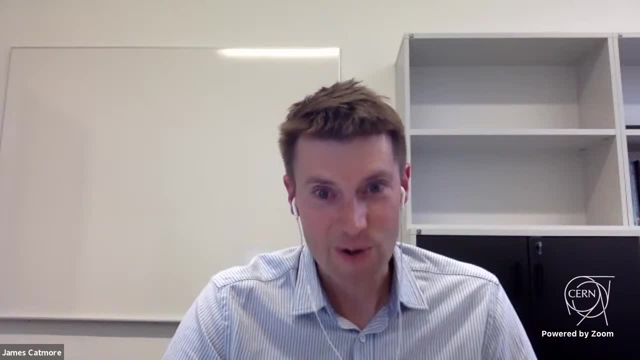 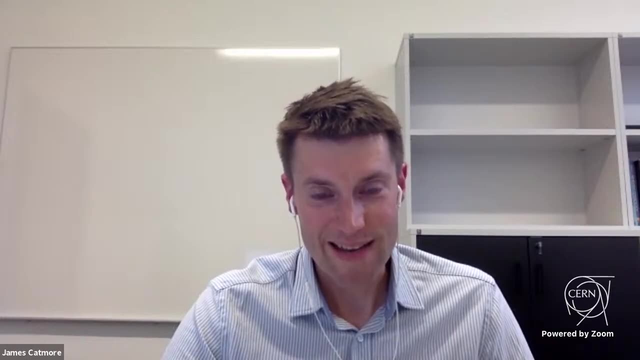 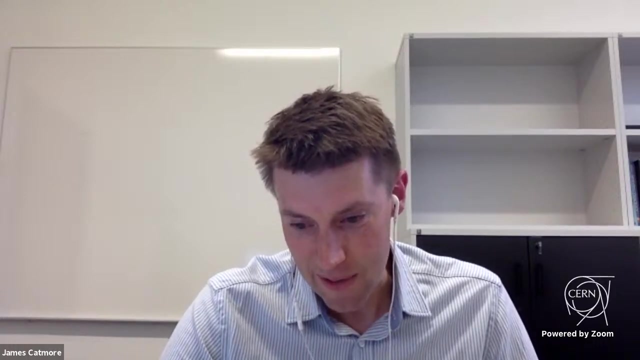 that people who are entering atlas now as students will be, uh, you know, senior scientists, uh, before they see kind of quantum computers coming in the um in any in any meaningful sense. i mean, you know they're making huge progress in companies like google and and others, but they are still many years. 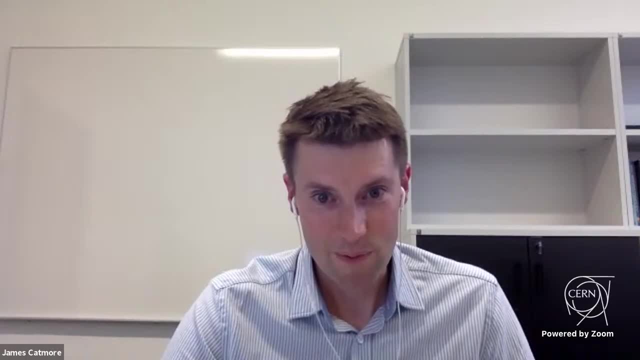 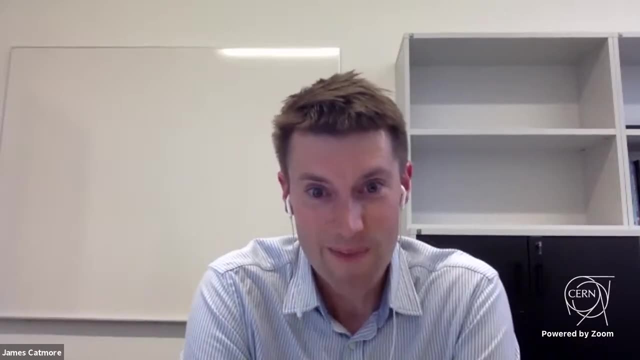 away from it, but still not much control over quantum computer. so, yeah, that's that's my, but that's my personal view. maybe i'll be proved wrong and in five years time we'll be, uh, forgetting about gpus and we'll be worrying about quantum computers, but i personally don't believe that will be the 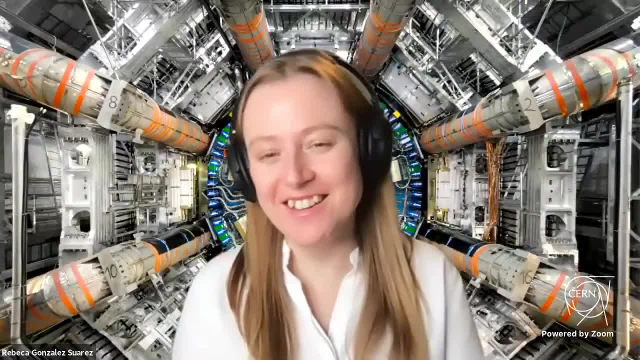 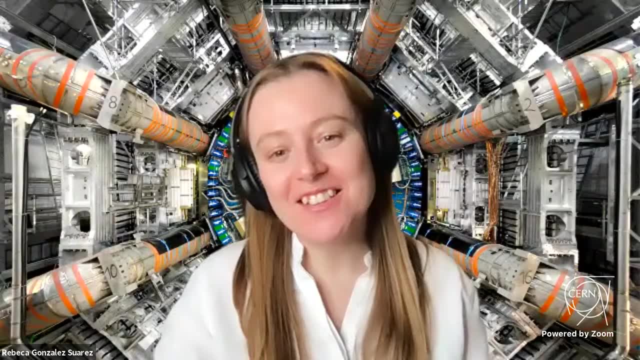 the case. all right. well, i think i think it's a pretty good answer as well, so i'm not. i'm not gonna go into this poster, so all right. so i think we are getting close to a pump, but we might have a couple of workshops on that, so we're hoping to work on that. i guess we could, you know, work on the ambient media of the bosporus or the little nuclear stuff. 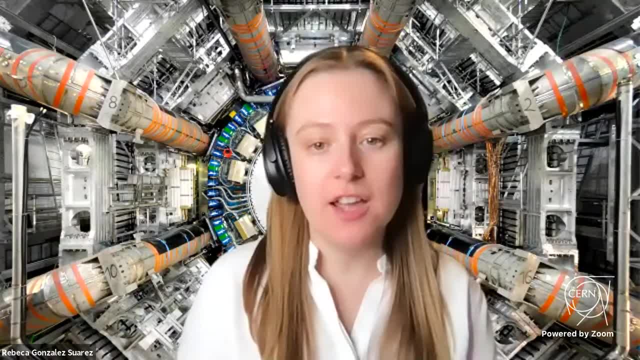 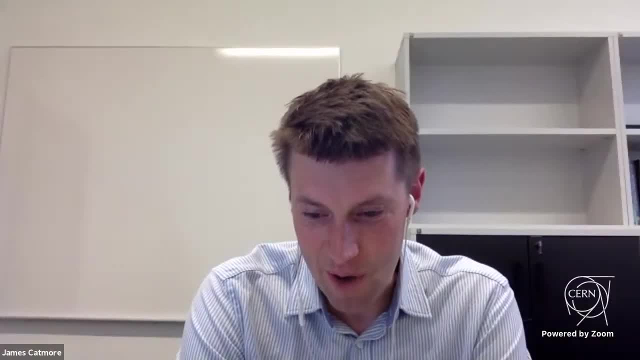 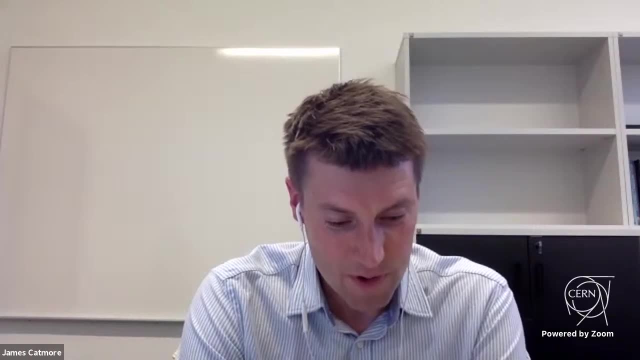 couple more questions. so one that comes from here, from the live chat, is, uh, which gpus are being considered for certain experiments? well, uh, at the moment, uh, it's this is a completely open question. uh, i mean, it's it's clear at the moment, um, that the easiest ones to use because of their 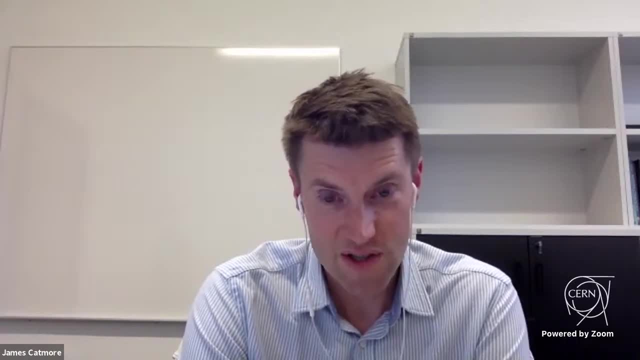 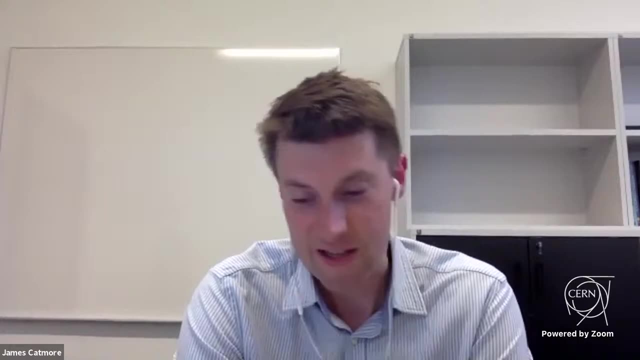 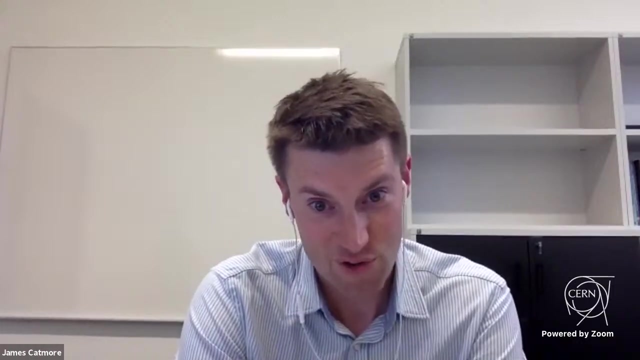 availability and also because the programming language is is the easiest to use and the most advanced is is nvidia. but that no mean by no means is the. this does not mean that we will be using nvidia forever. we'll probably end up using a mixture of different manufacturers. 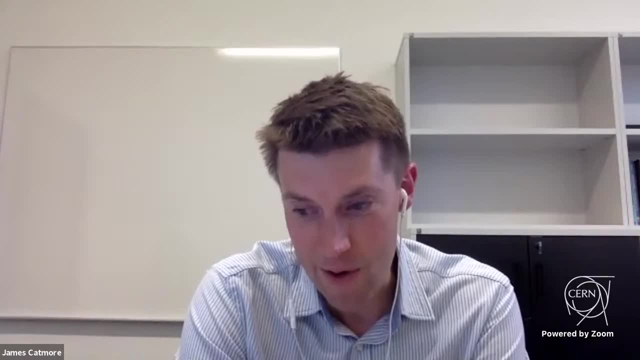 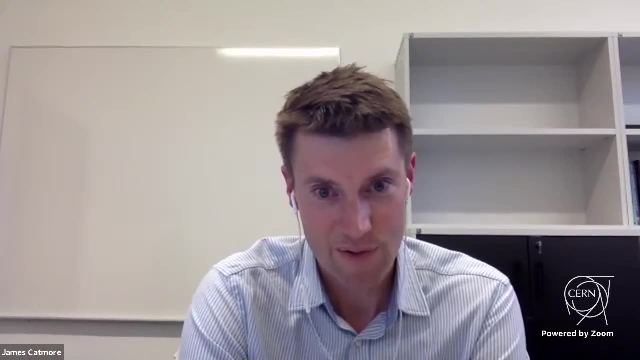 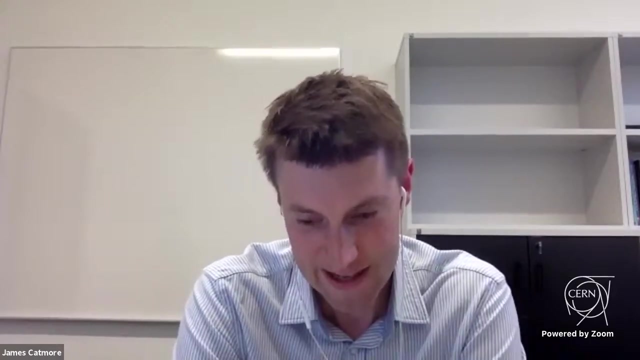 of gpus. i mean, we're talking here about gp gpus, so these are generally sort of um what they call server class gpus. it's not typically the kind of graphics cards that gamers will have in their um in their gaming pcs. they're they're a bit more powerful than this, and 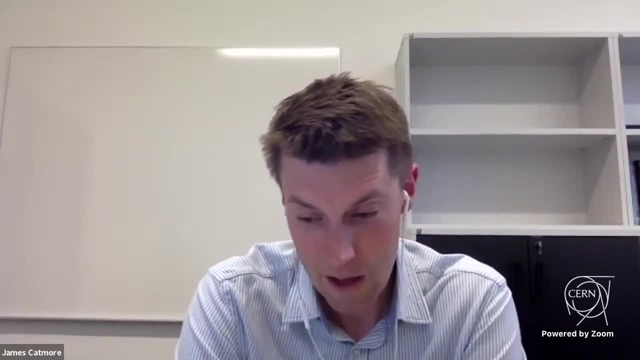 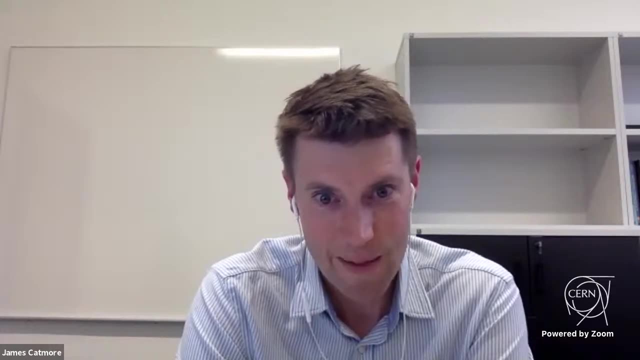 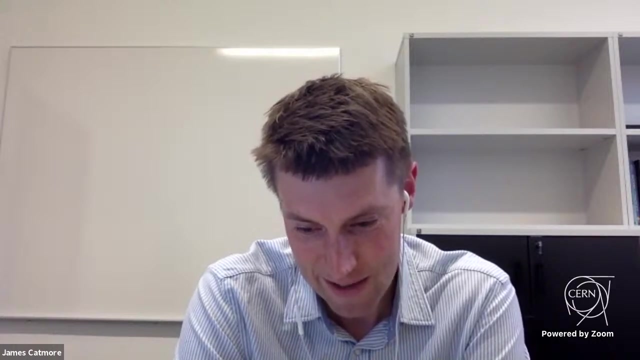 they typically are in data centers rather than in um, but yeah, i mean the, for instance in the uh, us, uh, different um very powerful computers are being built and they're buying the gpus from different vendors, not just from nvidia, but also from uh, from intel and and amd and other vendors as well. 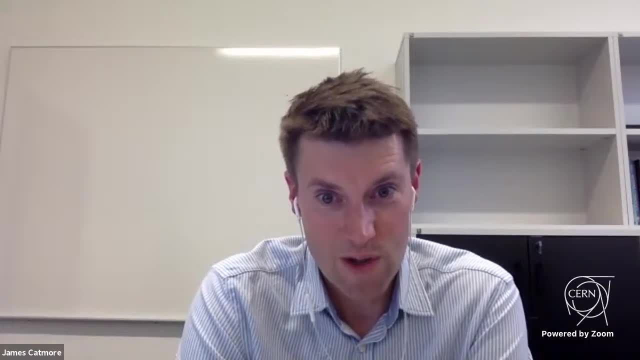 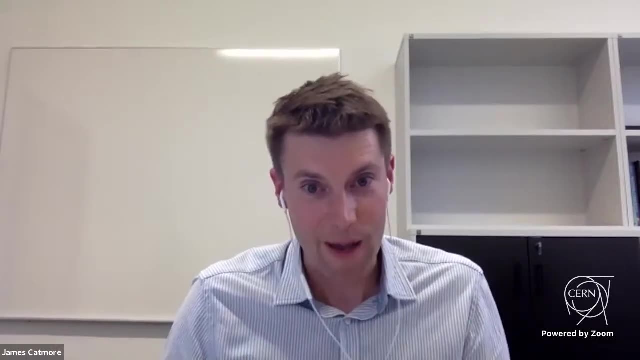 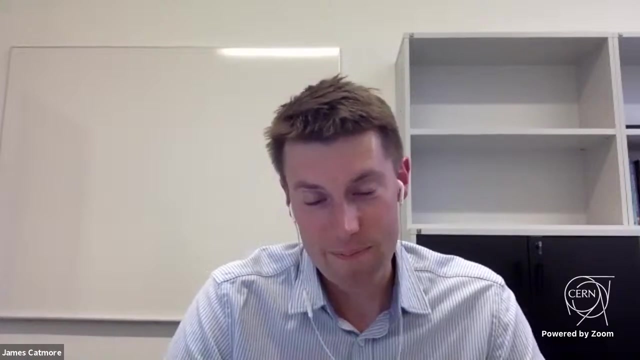 so yeah, at the moment it's a totally open question, if you want to, if people want to know what kind of gpus are we mostly working with at the moment to develop and to experiment and to find out how we may use them in the future. uh, the answer is mostly at the moment to nvidia, but, um, that's. 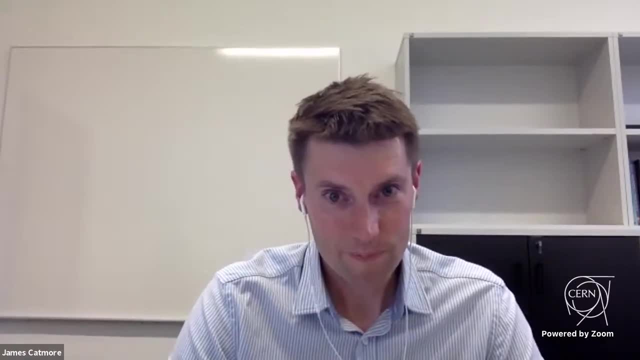 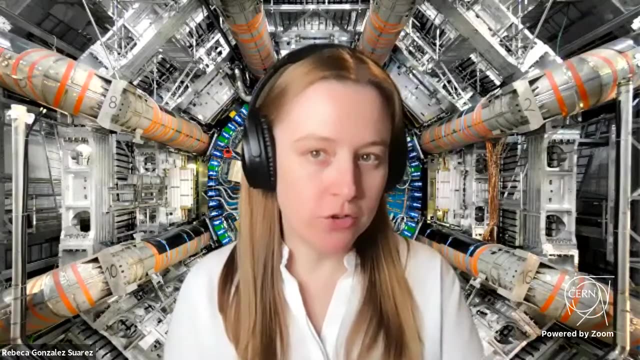 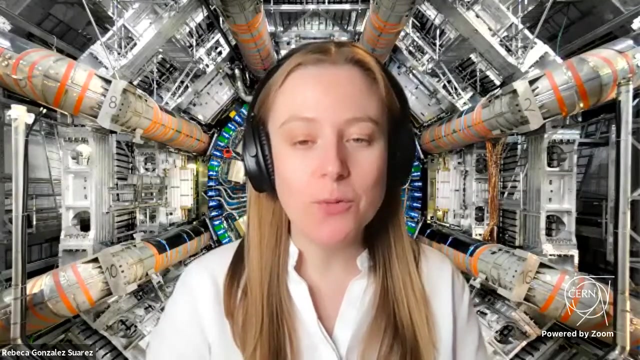 not to say that this will be the case, uh, for forever. thank you very much for that, and i think then we are about to close, so probably we give you the very last question. that is going to be a little bit more on the personal side. so that question is: how many gigabytes does your computer have? 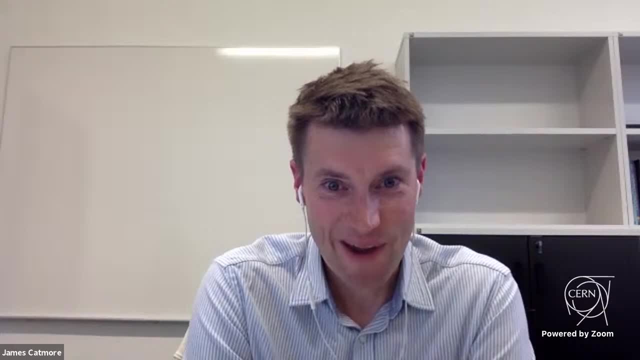 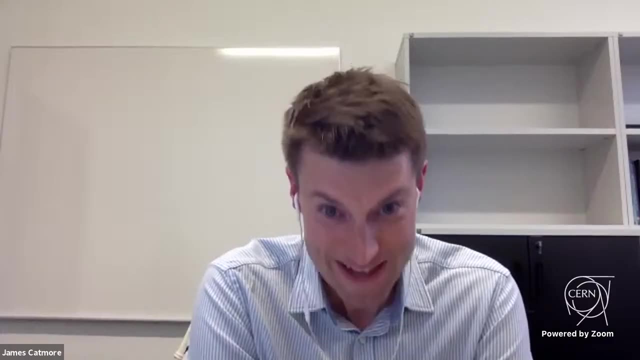 memory and storage, my personal computer, my laptop, right so well, uh, it's a very, very uh old one. my, my laptop is from 2015, so, uh, i think even it's on the slides, actually, because i i didn't, i didn't draw my attention to. 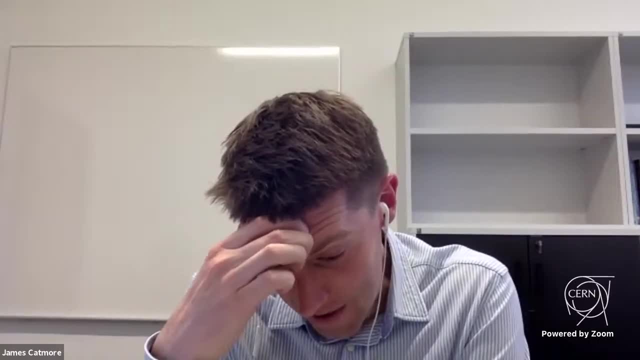 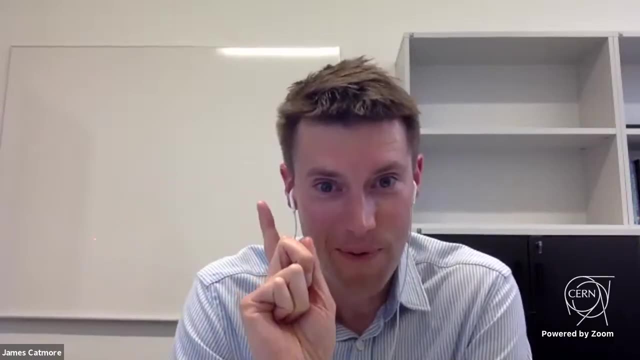 it. so it's dual core, um, it's a dual core, uh, macbook air, um, and memory, uh, i. ah, now i. i remember i asked the university that i wanted one with a really good memory. so it's eight gigabytes because i wanted to have one with a really good memory. so i wanted to have one with a really good. 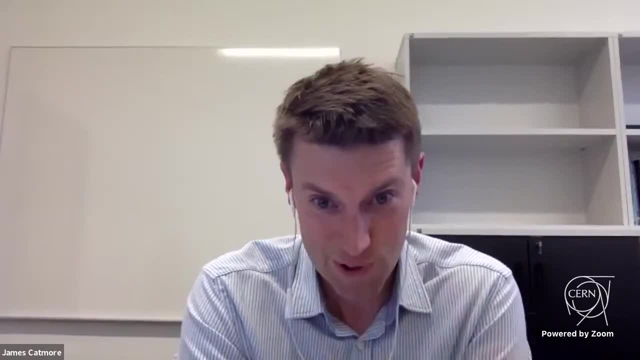 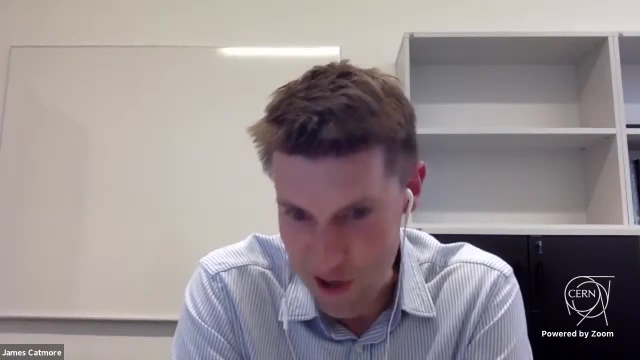 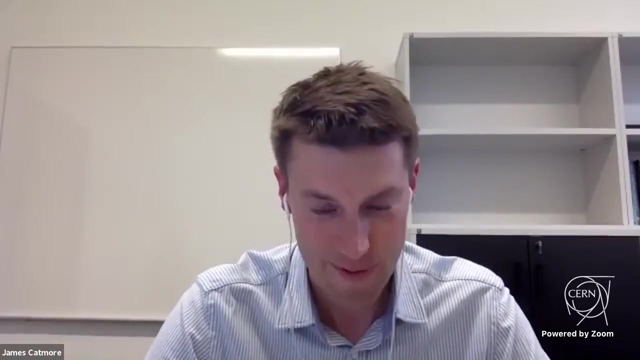 oh no, no, that wasn't available. my personal computer is eight, but this one is four, so two cores and four gigabytes. and just as a bit of a humorous joke to finish, i said: i don't care you know what color it is or how big the screen is, but i really, really want it to have.